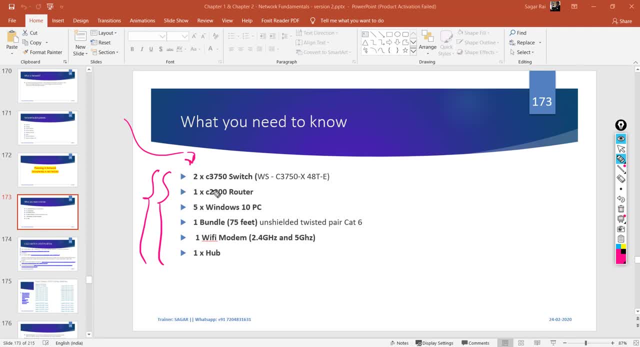 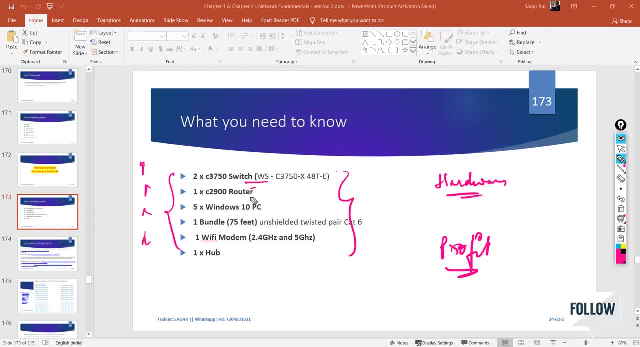 he is sending us Now. it is up to us to buy the best hardware. So this is the requirement he is sending us Now. it is up to us to buy the best hardware. So this is the requirement, me. okay, so we will understand the requirement first and then, accordingly, we will buy whatever. 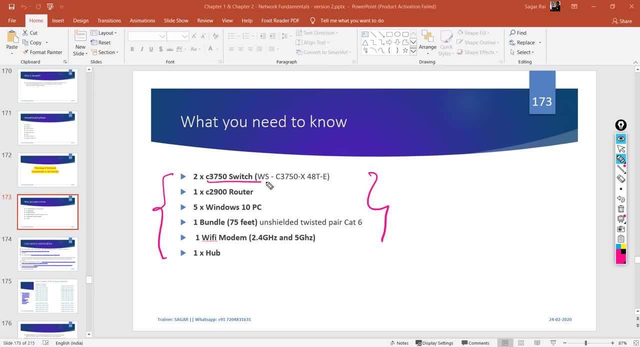 he wants? okay, so he has mentioned us the variant. okay, he wants cisco 3750 model. okay. so first of all we should understand what types of models are available, okay, and then he has given some code. so what is this code actually referring to? okay, so i hope you guys understood what are each. 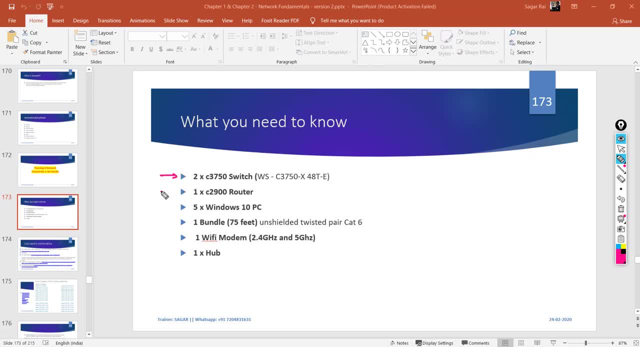 components: okay, this is a cisco switch, cisco router, uh computers cable, wi-fi model hub, okay. so basically, you can imagine the design something like this: okay, like five computers kept next to next which are connected. you can imagine the design something like this: okay, like five computers kept next to next. 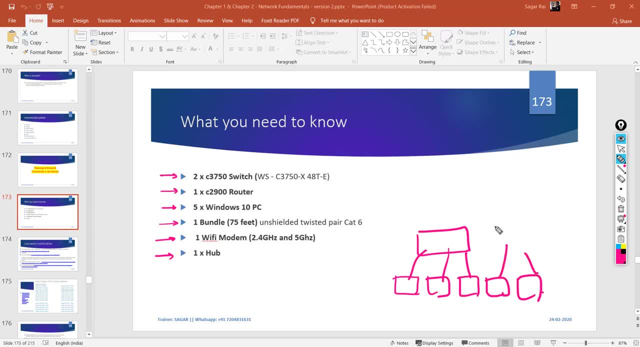 you can imagine the design something like this: okay, like five computers kept next to next to two switches- okay, then i have one router. okay, router is used for connecting to isp, and then i have all the cables used up. i need one modem so i can connect one mod modem here, wi-fi modem, okay. 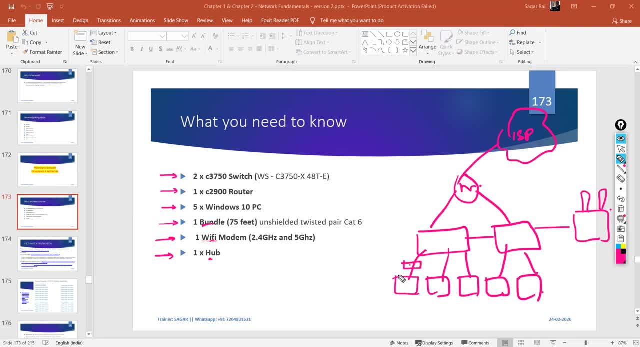 and one hub, so probably i can keep one hub here, okay, so something, something like this: so this would be my network, would be my network design of that company. okay, and only for five users. so let's first understand in terms of devices. okay, if someone is asking you that he needs this uh variant, so that means this: 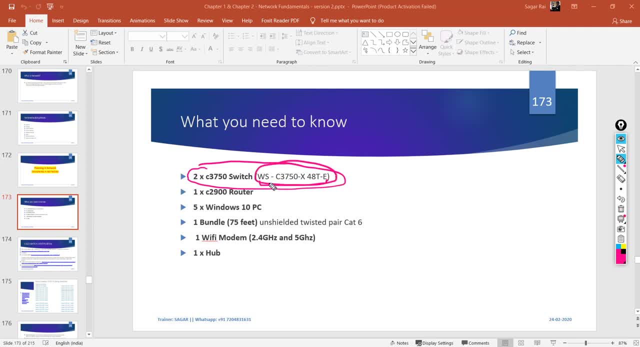 device is this particular device is capable of something? or or, if someone asks you, or at least in your interview, someone asks you: what does ws refer in this switch? or what does t refer? okay, so what does e refer? so you should know, right. so we will go to the next slide, where i'll first tell you the terminologies here. 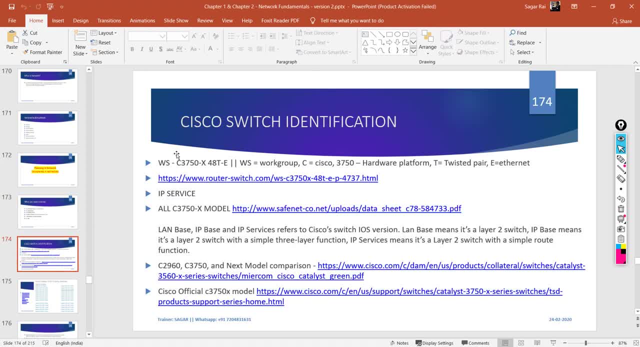 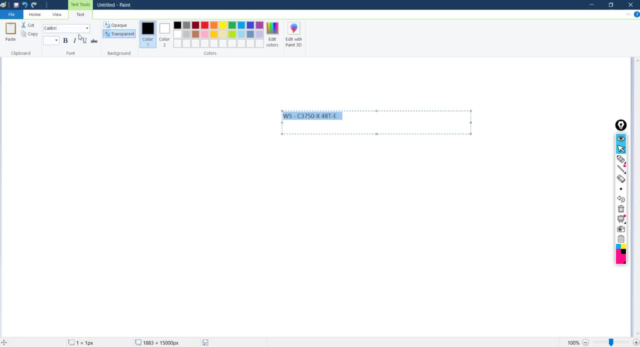 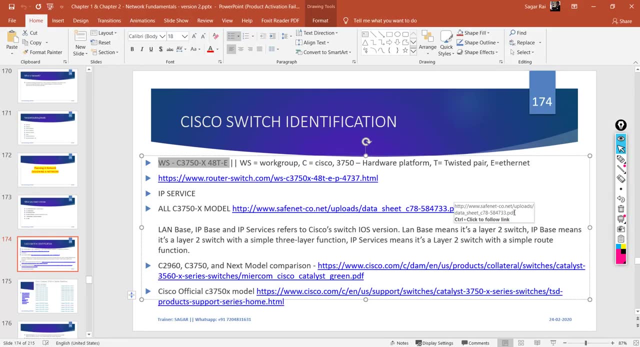 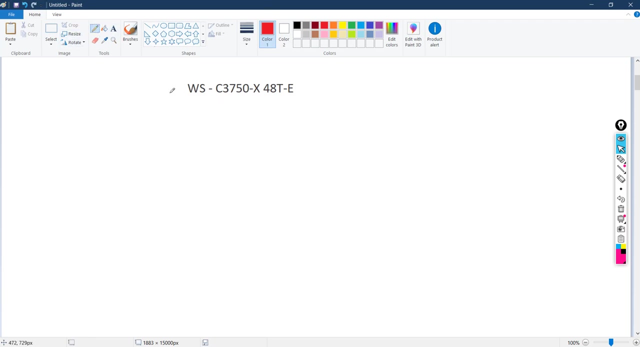 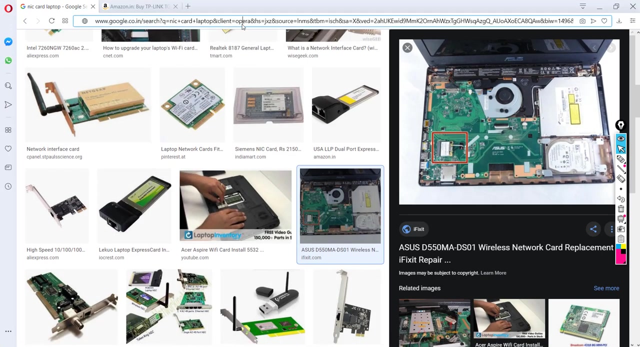 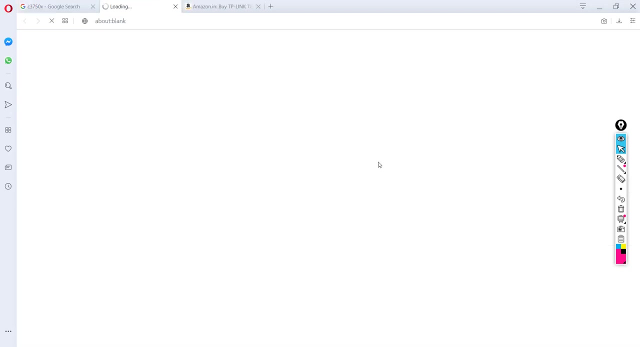 okay, so let's pick up this for explanation. okay, so imagine the customer wants this switch. this is one of the switch model, okay, and if you want to see how do this looks like, so you can just search over here. so this is the switch which, which is a part of our requirement, okay, 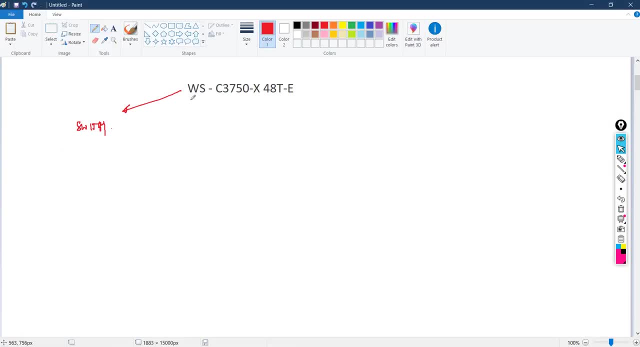 so first we should understand what. what is this referring to? so ws is nothing but work group. okay, work group c refers to cisco. this is the platform or the hardware version. i can call it as hardware version or platform version. okay, x is nothing, but it's an upgraded version of the previous model. so basically, you can see. 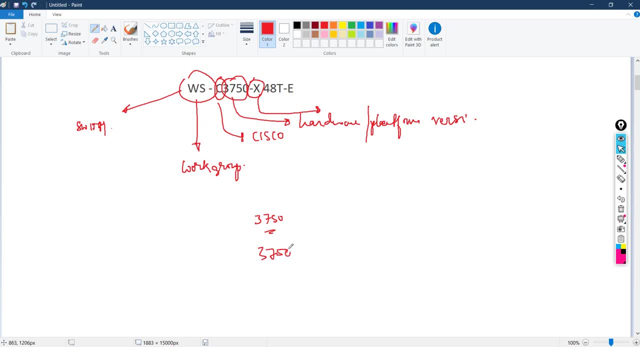 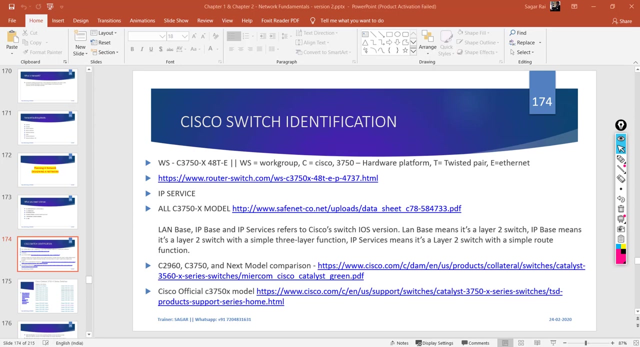 3750 also and you can see 3750x. so basically, x is the latest version of this. okay, i, i will write it as latest version of 3750. okay, 48 is nothing but 48 ports, that is so if you see here the ports here. so basically that refers to: 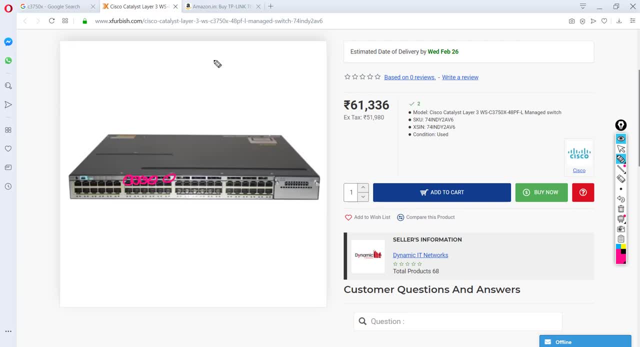 48 port number. so how many port numbers can we uh get in the market? so minimum: start with 8 port, then comes uh the 24 port, then we have 48 port. okay, so our customer wants 48 port. so basically this switch is 48 port. 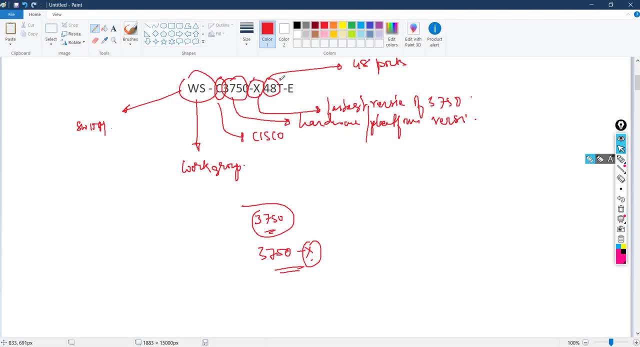 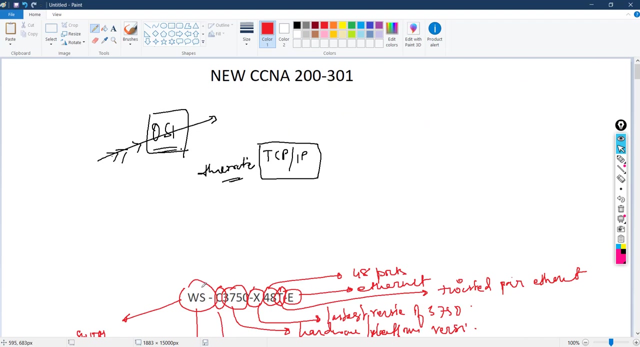 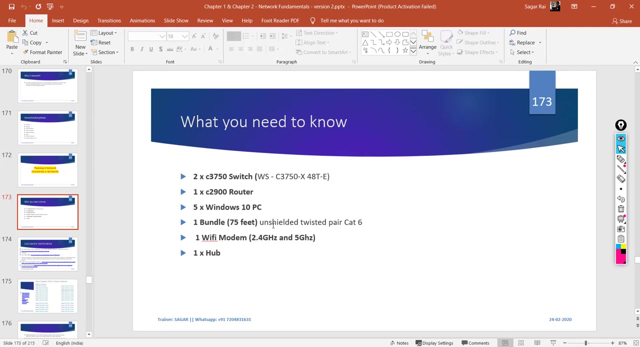 okay, what is t referred to? t is referring to twisted ethernet pair. okay, twisted pair and e is nothing but ethernet. okay, so this is what a complete terminology is referred to. okay, a one small device. if someone is sending us a requirement to have um to have this devices installed in uh in in his office, in the customer office. 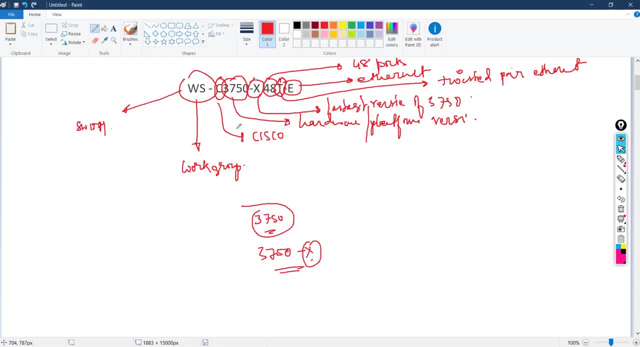 and he's giving us the requirement. so we have to first understand. what does it mean? what does that hardware refers to? okay, so let's first see different types of variant available in this, okay, so we will understand like what kind of different variants we can see. so, one among the variant is this one, okay, which is our requirement. okay, so this is one of the. 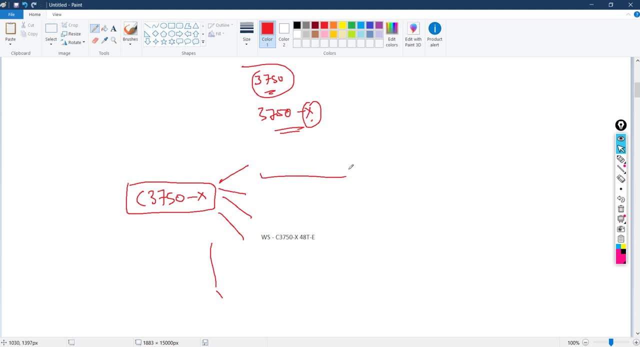 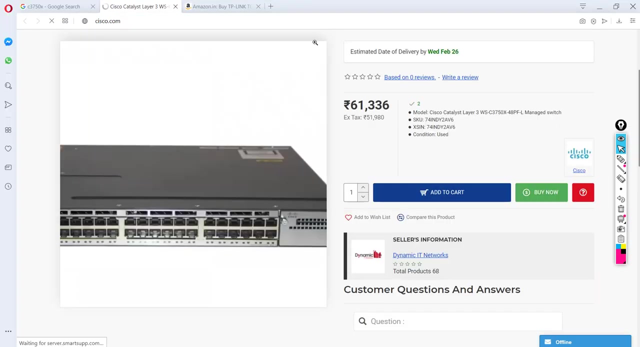 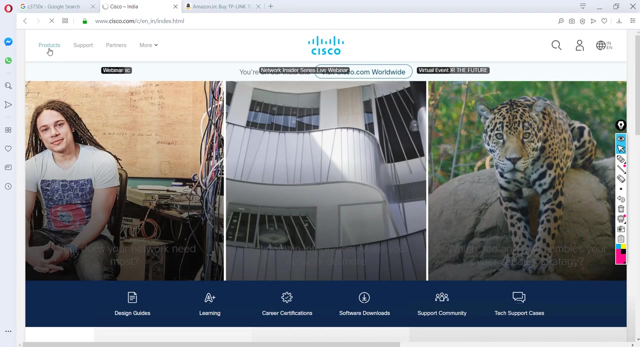 variant. now let's see if we have any other variant. and what does they mean? okay, why? why customer only selected this? why didn't he select anything else? okay, so if i go to the cisco website, ciscocom, if i search for the products, okay, if i click on the products so i can straight away click on switches. 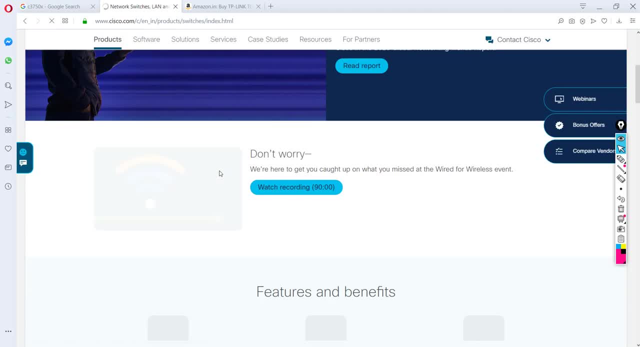 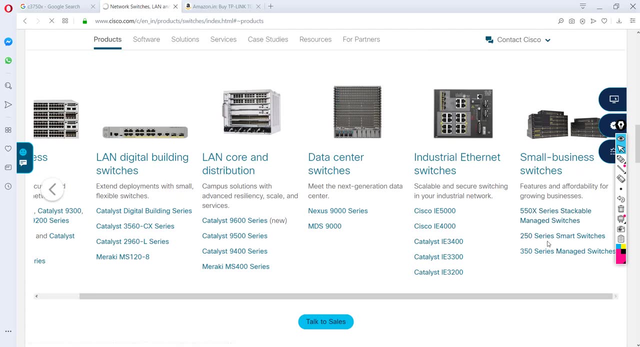 okay, so i can get a lot of things here. so basically they are all different variants. okay, so mine is somewhere here in the land switches. okay, so i can get a lot of things here. so basically they are all different variants. okay, so mine is somewhere here in the land switches. 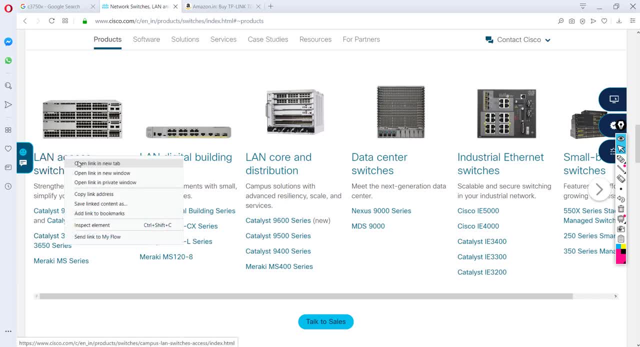 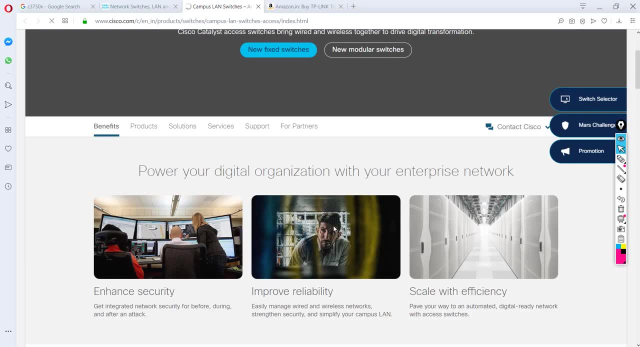 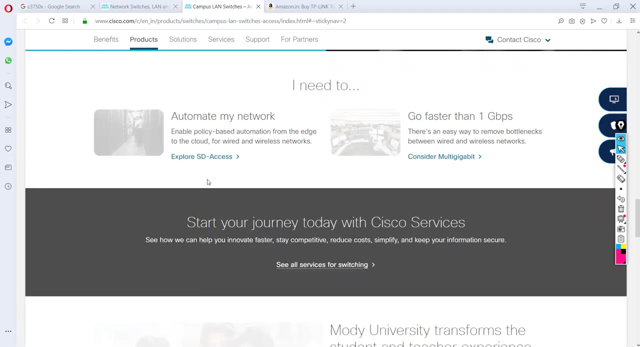 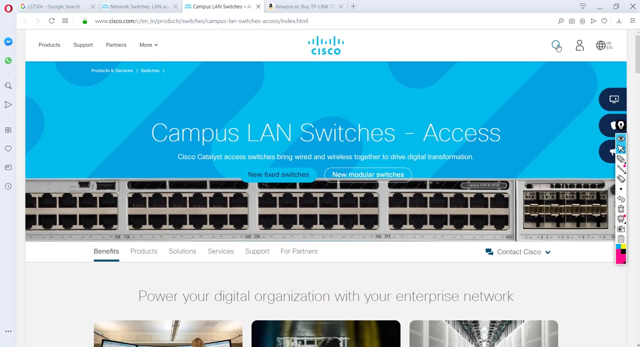 okay, which is used in the local area network, so i'll open up this. okay, so do i have my 3750 somewhere here? okay, or? or? in case, if you're not able to find, then just make use of the search bar. you can type 3750x. 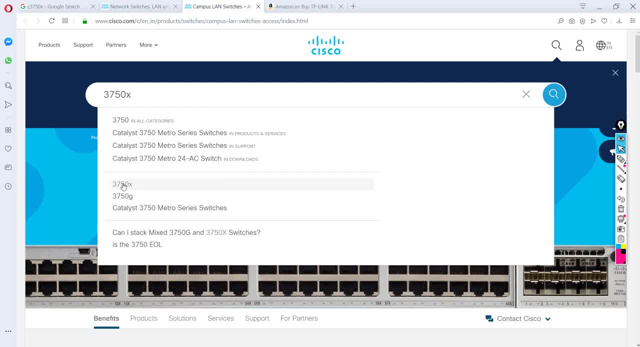 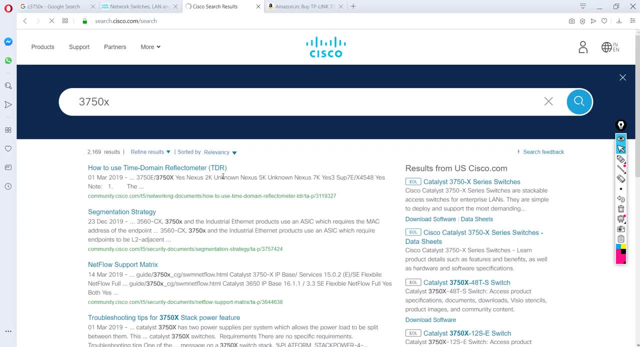 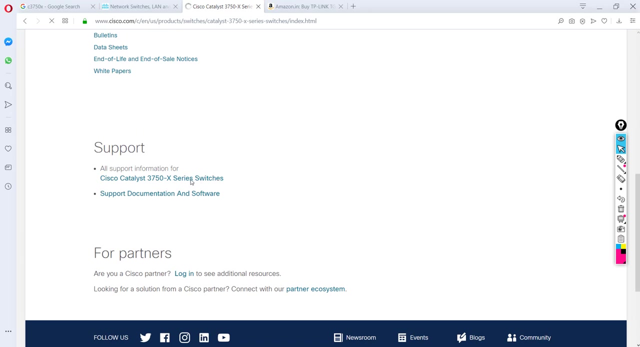 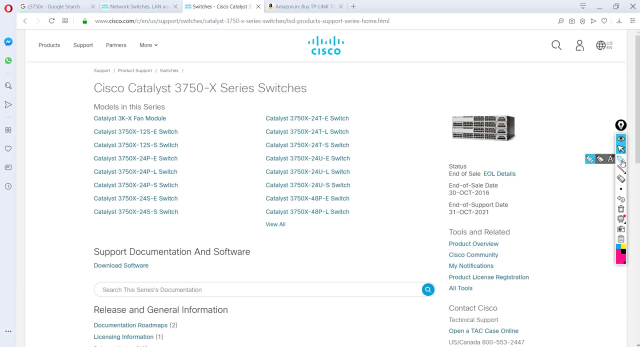 okay. so i'm going to open up this. okay, and we are going to get it 3750x. okay, and we are going to get it 3750x. okay, and we are going to get it 3750x. so this is all the variant of 3750. 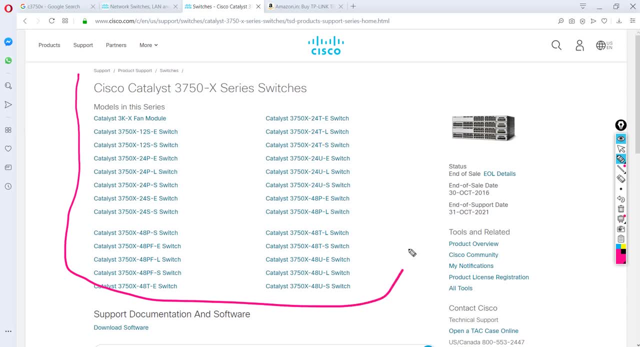 so this is all the variant of 3750. so this is all the variant of 3750. fine, so cisco has so many variants of fine. so cisco has so many variants of fine. so cisco has so many variants of 3750 and which is the one which customer 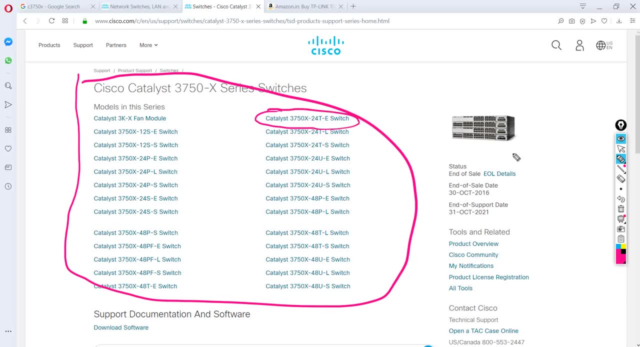 3750 and which is the one which customer 3750 and which is the one which customer wants us to install? that is this one. okay, wants us to install. that is this one. okay, wants us to install. that is this one. okay, sorry, not that one, it is 48. 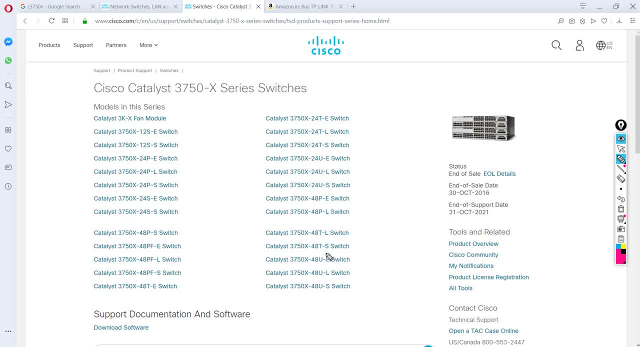 sorry, not that one. it is 48. sorry, not that one. it is 48. port right, so under 48. okay, this is the one. okay, this is the one. okay, this is the one. so, out of these many options, so out of these many options, so out of these many options, customer wants us to buy this one, so 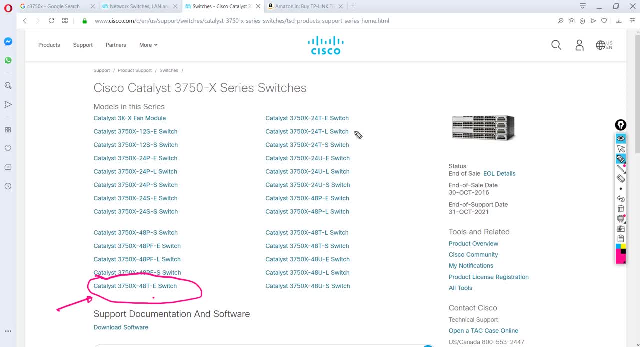 customer wants us to buy this one. so customer wants us to buy this one. so that is your first decision. you just that is your first decision. you just that is your first decision. you just cannot go and buy something else. just cannot go and buy something else, just. 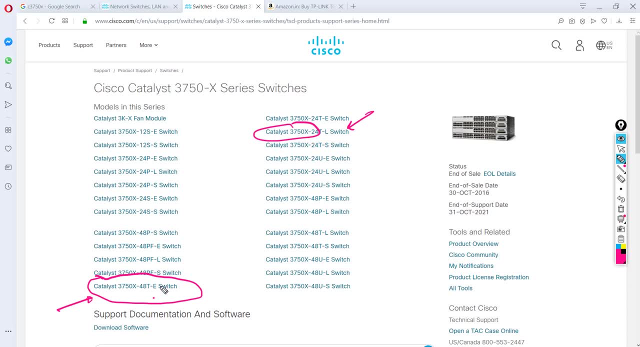 cannot go and buy something else just because it is also 3750x. you should, because it is also 3750x. you should, because it is also 3750x. you should understand what does 48 understand. what does 48 understand? what does 48 or t or e refers? see if you see other. 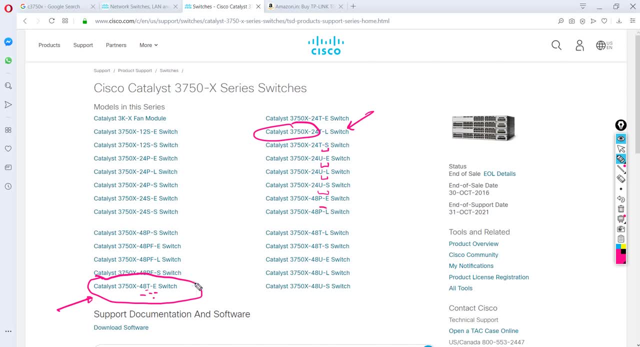 or t or e refers see if you see other. or t or e refers see if you see other things. they are different codes here things. they are different codes here, things. they are different codes here. okay, customer has asked us to buy t. okay, customer has asked us to buy t. 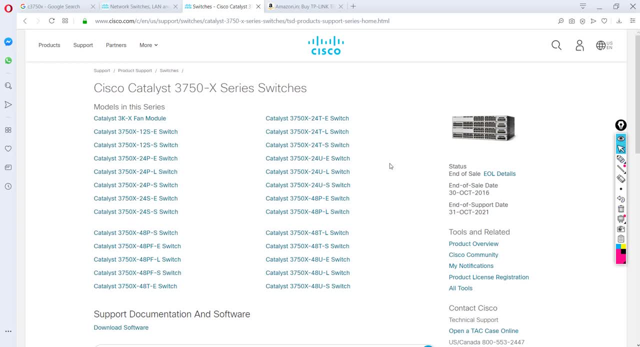 okay, customer has asked us to buy t hyphen e okay. so basically, if you try hyphen e, okay. so basically, if you try hyphen e, okay. so basically, if you try to understand, if you try to break down to understand, if you try to break down, 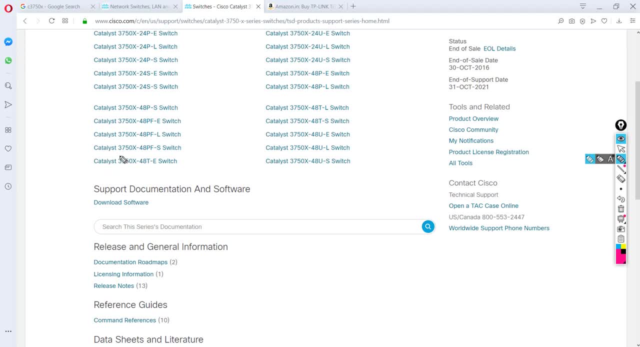 to understand if you try to break down them. so you know what is what okay. so them, so you know what is what okay. so them, so you know what is what okay. so this is a platform name. this is this is a platform name. this is, this is a platform name. this is the upgraded version of the 3750. 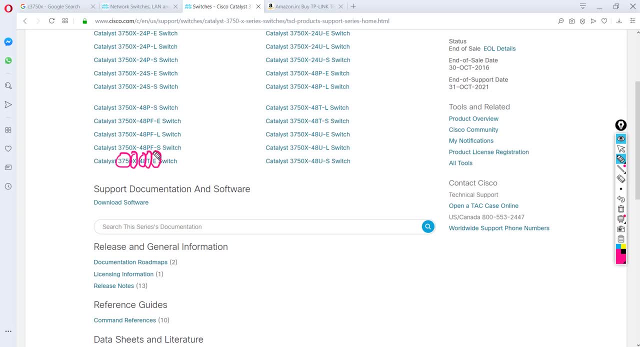 the upgraded version of the 3750. the upgraded version of the 3750. this is switchport. this is twisted pair. this is switchport. this is twisted pair. this is switchport. this is twisted pair. this is ethernet medium. okay, this is ethernet medium. okay, this is ethernet medium. okay, what about others? so let me uh quickly. 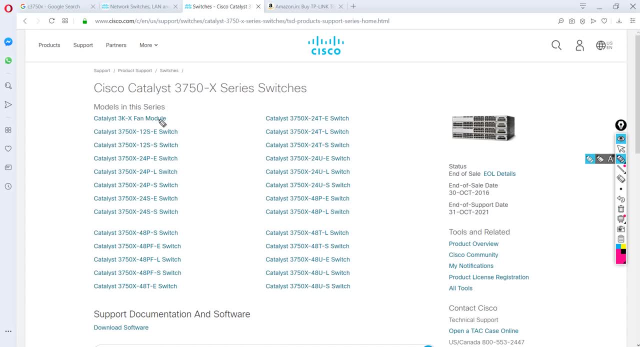 what about others? so let me uh quickly, what about others? so let me uh quickly uh summarize the other things. so if you uh summarize the other things, so if you uh summarize the other things, so if you see s that refers to stackable, see s that refers to stackable. 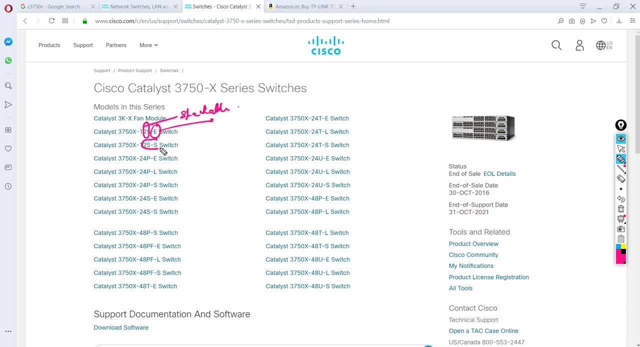 see s. that refers to stackable. okay, e is for ethernet. this is again okay. e is for ethernet. this is again okay. e is for ethernet. this is again stackable switch. stackable switch. stackable switch. this is poe power over ethernet. okay so, this is poe power over ethernet, okay so. 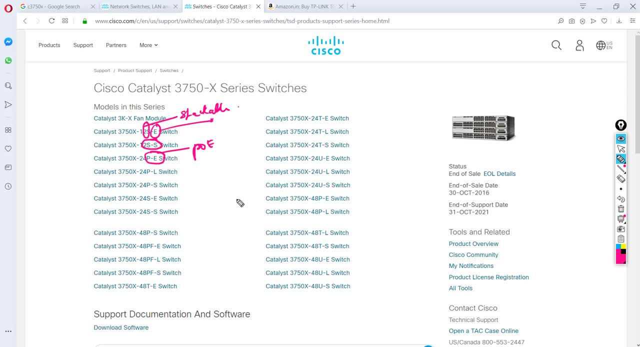 this is poe power over ethernet. okay, so that is why they are all defined with. that is why they are all defined with. that is why they are all defined with different terms. okay, so, if we can open different terms, okay, so, if we can open different terms, okay, so, if we can open them, we can, we can open this and we can. 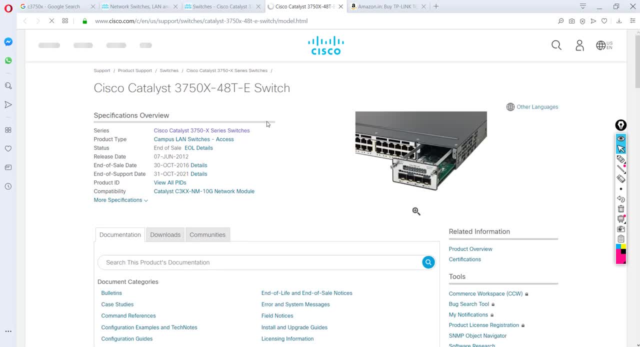 them. we can. we can open this and we can them. we can. we can open this and we can see uh what in depth, like what is support? see uh what in depth, like what is support? see uh what in depth, like what is support was supporting to all those things. okay. 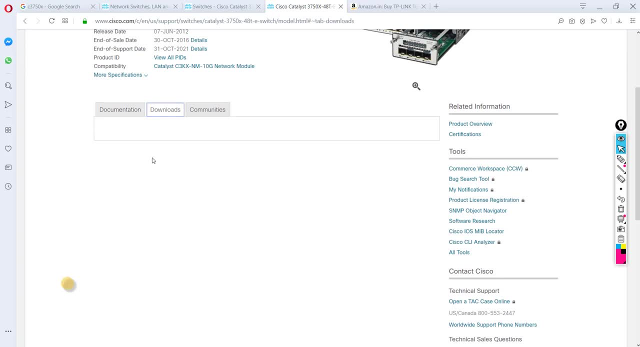 was supporting to all those things, okay, was supporting to all those things, okay. so basically, these are all the features. so, basically, these are all the features. so basically, these are all the features. okay, you can download the software. okay, you can download the software. okay, you can download the software for this. uh. 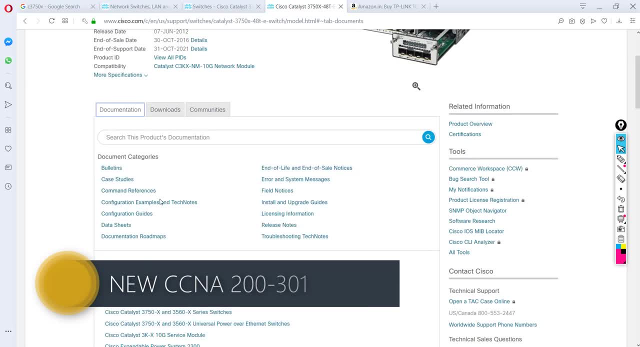 for this uh. for this uh: device from device from device from download center, download center, download center under documentation. you can see uh under documentation. you can see uh under documentation. you can see uh the data sheet, the data sheet. the data sheet, you can see the case studies. okay, so, 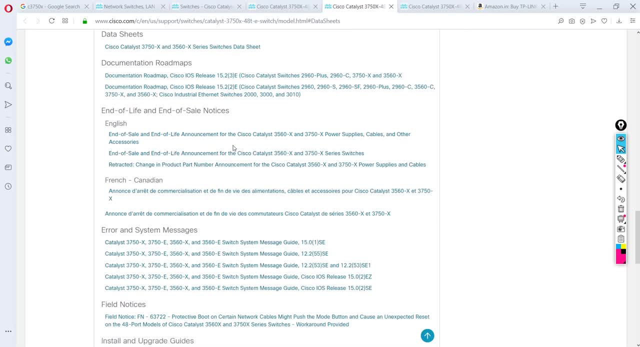 you can see the case studies. okay, so you can see the case studies. okay. so everything you can get as a uh network, everything you can get as a uh network, everything you can get as a uh network, design engineer- okay, so your your role. design engineer- okay, so your your role. 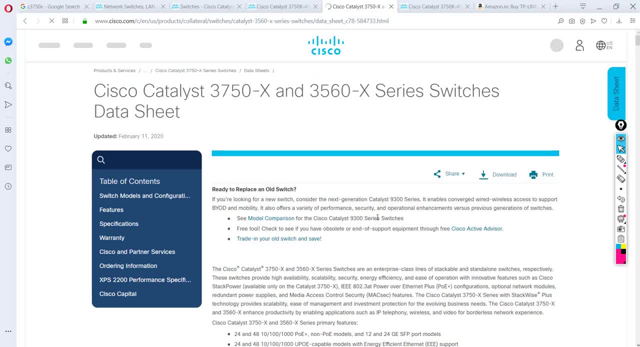 design engineer. okay, so your, your role is not just to go and buy blindly. you is not just to go and buy blindly. you is not just to go and buy blindly. you should understand, okay, you should, should understand. okay, you should should understand. okay, you should understand what features your customer. 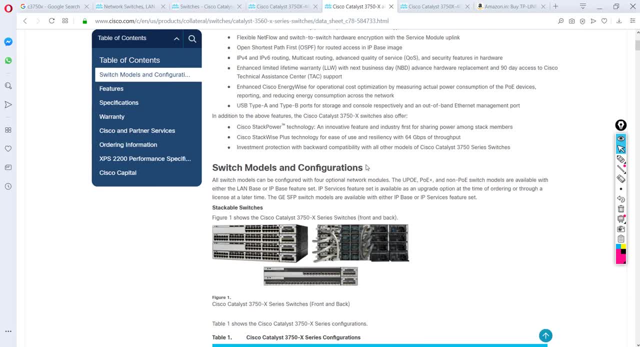 understand what features your customer, understand what features your customer wants and wants and wants and what are you going to buy? okay, so, if you. what are you going to buy? okay, so, if you, what are you going to buy? okay, so, if you, if you check the data sheet of this, so, 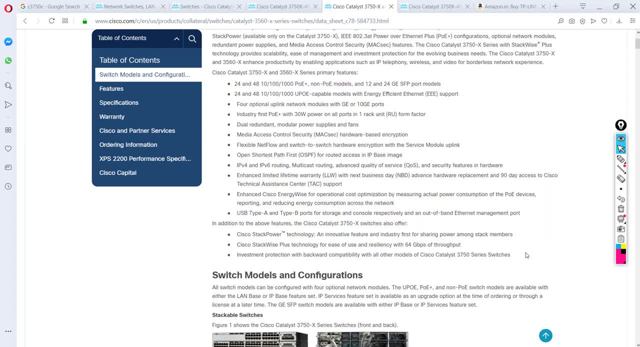 if you check the data sheet of this, so if you check the data sheet of this, so you will see every possible thing. this, you will see every possible thing. this, you will see every possible thing. this device can support: okay, it is supporting. device can support: okay, it is supporting. 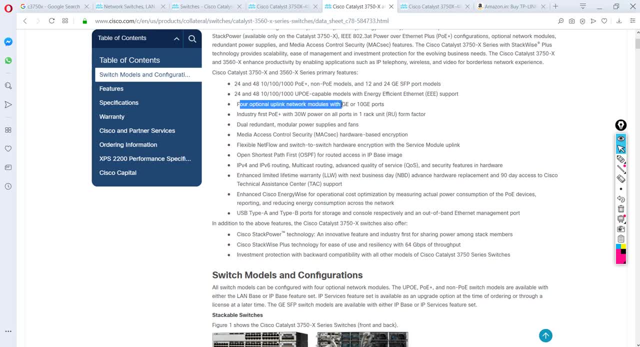 device can support. okay, it is supporting poe. it is having four optional uplink poe. it is having four optional uplink poe. it is having four optional uplink. okay, these are the different ports that. okay, these are the different ports that. okay, these are the different ports that it is coming up with, okay. 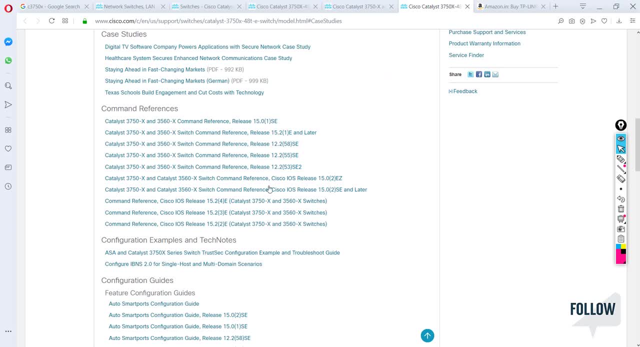 it is coming up with. okay, it is coming up with. okay, then the ospf, all those things. okay, then the ospf, all those things. okay, then the ospf, all those things. okay, there is. there is one more website which. there is. there is one more website which. 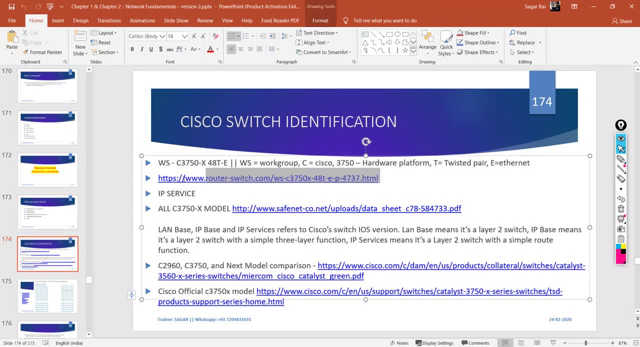 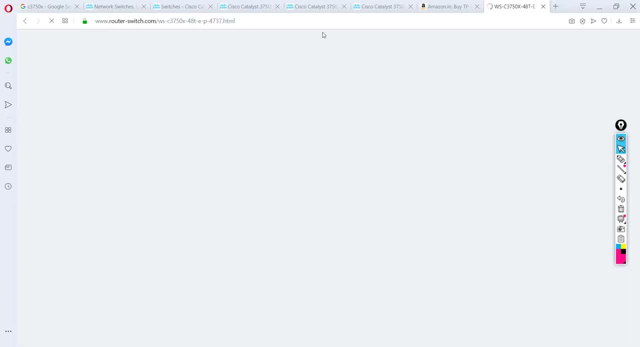 there is, there is one more website which, uh, uh, uh, can give you little bit more information. can give you little bit more information. can give you little bit more information, okay, okay, okay. so let me show you that website and let's search, and let's search, and let's search for. 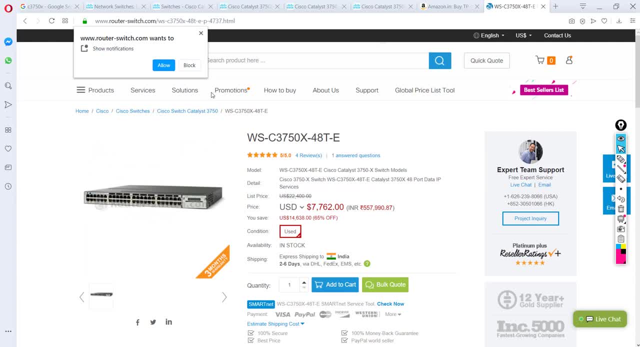 and let's search for this model, this model, this model. okay, so, basically, this is the model and okay. so, basically, this is the model and okay. so, basically this is the model and it has, it has. it has straight away come to that. okay. so, if we straight away come to that, okay, so, if we 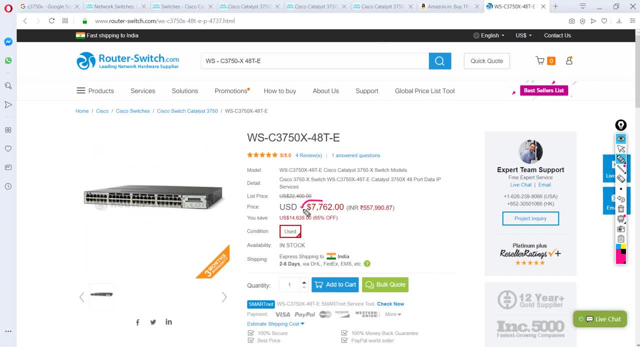 straight away. come to that, okay. so if we, if we see this model it is giving us, if we see this model it is giving us, if we see this model, it is giving us the price over here, okay, so, basically the price over here, okay. so, basically the price over here, okay. so, basically, this is a 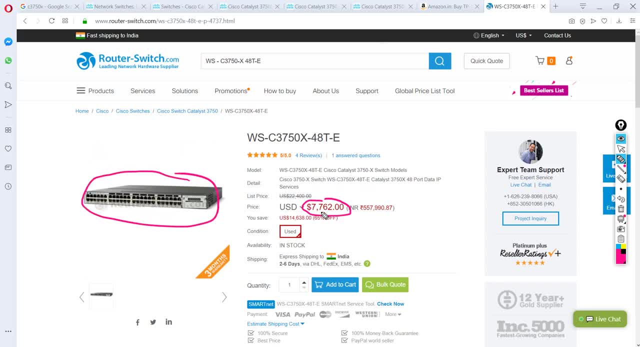 this is a this is a device which is costing up to 7.7 device which is costing up to 7.7 device which is costing up to 7.7 k usd dollar, which is which is k usd dollar, which is which is. 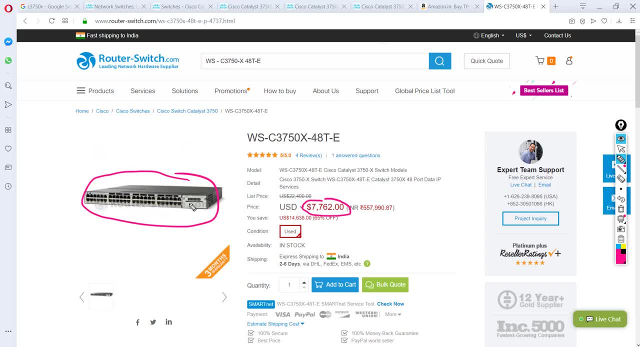 k usd dollar, which is which is a heavy amount. so you just cannot a heavy amount. so you just cannot a heavy amount. so you just cannot play around. you just cannot ignore the play around. you just cannot ignore the play around, you just cannot ignore the things. okay, 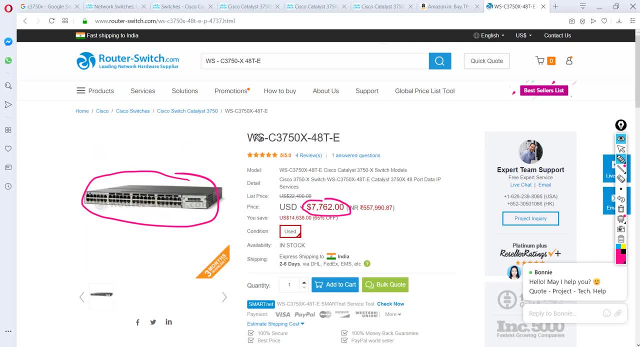 things okay, things okay. so you have to make wise decision before. so you have to make wise decision before. so you have to make wise decision before going and purchasing anything- okay, going and purchasing anything- okay, going and purchasing anything- okay, later on, you are the one who is going to. 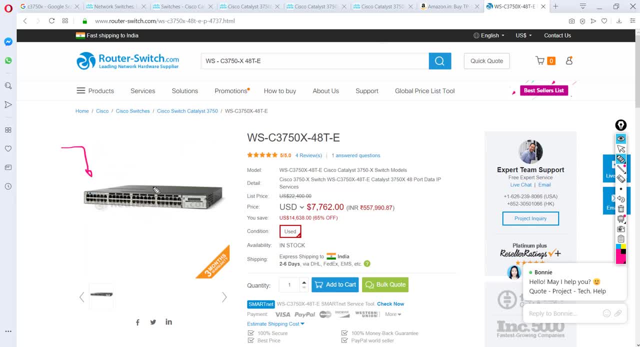 later on. you are the one who is going to later on. you are the one who is going to give the day-to-day- uh, give the day-to-day, uh, give the day-to-day- uh support on this device, right? so, if, support on this device, right? so if? 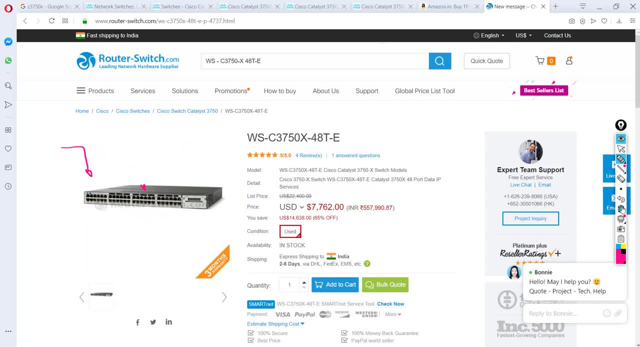 support on this device, right? so if something is breaking up, then you should. something is breaking up, then you should. something is breaking up, then you should know how to fix it up right. so you know how to fix it up right. so you know how to fix it up right, so you should probably become the master of. 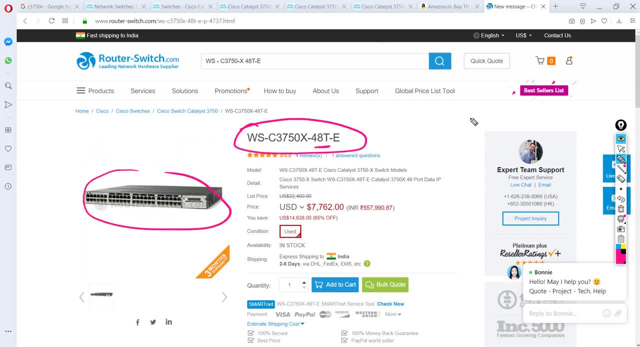 should probably become the master of, should probably become the master of this, this, this device or this variant rest. you can device or this variant rest, you can device or this variant rest, you can ignore it. so every time, whichever ignore it, so every time, whichever ignore it, so every time, whichever customer you are placed to. 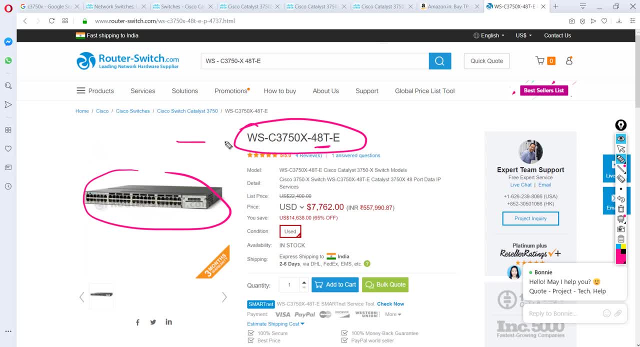 customer. you are placed to customer. you are placed to to to take care of their uh network. so to to take care of their uh network, so to to take care of their uh network. so first you have to learn what all, first you have to learn what all. 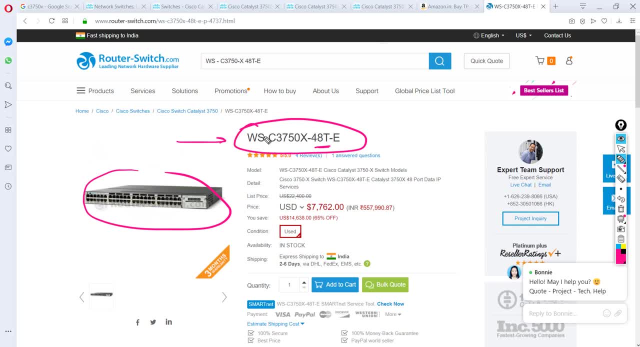 first you have to learn what all devices they have, and then you should devices they have, and then you should devices they have, and then you should learn about those devices only okay. learn about those devices, only okay. learn about those devices, only okay. you might have seen some people saying: i 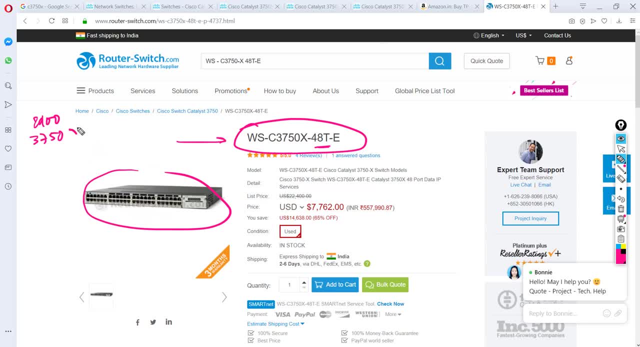 you might have seen some people saying i. you might have seen some people saying i have worked on 2900, have worked on 2900, have worked on 2900. i have worked on 3750x. i have worked on. i have worked on 3750x. i have worked on. 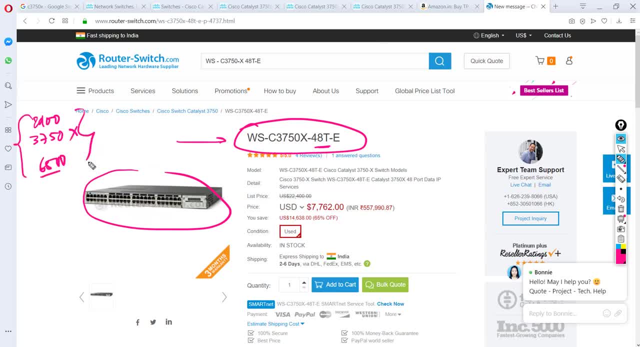 i have worked on 3750x. i have worked on 65, 65, 65- uh k right. so that doesn't mean that uh k right. so that doesn't mean that uh k right. so that doesn't mean that they, they are, uh, they, they are uh. 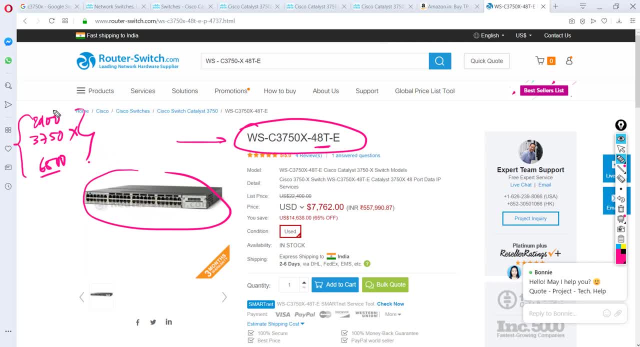 they, they are, uh, they, they are, they, they are, uh, they, they are, they, they are, uh, they, they are. they doesn't know any other variant, or they doesn't know any other variant, or they doesn't know any other variant, or something that means that they have. 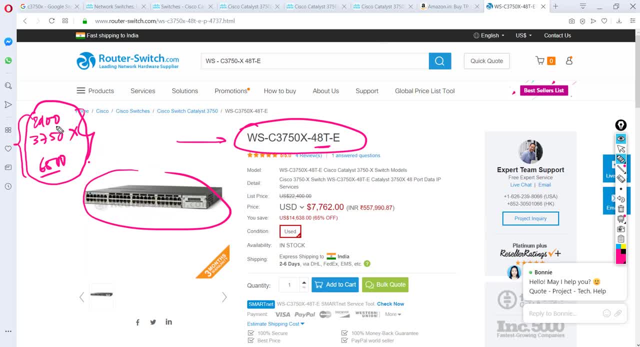 something that means that they have something, that means that they have uh like in-depth worked on these, uh like in-depth worked on these, uh like in-depth worked on these. technology in on these uh hardwares- okay. technology in on these uh hardwares- okay. technology in on these uh hardwares, okay. during uh your interview also. 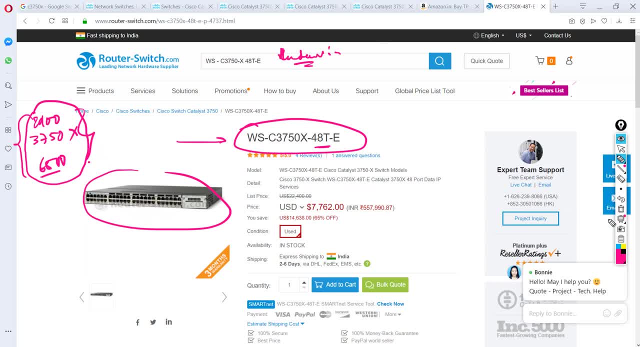 during uh your interview also during uh your interview, also straight away, interview straight away. interview straight away. interview interviewer is going to ask you that. which interviewer is going to ask you that? which interviewer is going to ask you that which? what kind of, what kind of what kind of uh switches or routers have you worked on? 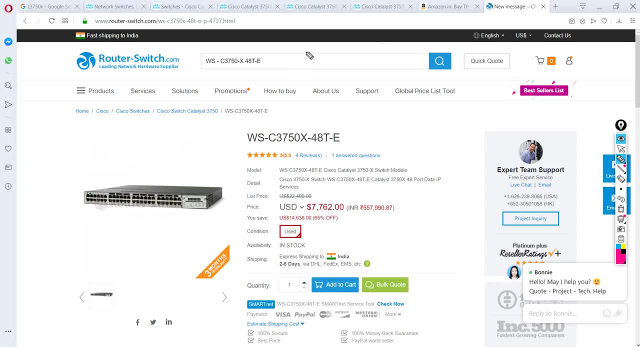 uh. switches or routers. have you worked on? uh, switches or routers. have you worked on what? what platform have you worked on what? what platform have you worked on what? what platform have you worked on? so you just cannot say: i worked on uh. so you just cannot say: i worked on uh. 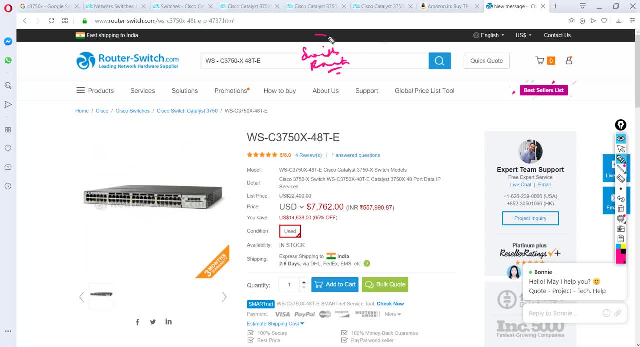 so you just cannot say: i worked on, uh, the switches, or i have worked on router the switches, or i have worked on router the switches, or i have worked on router. he is going to ask which variant in the. he is going to ask which variant in the. 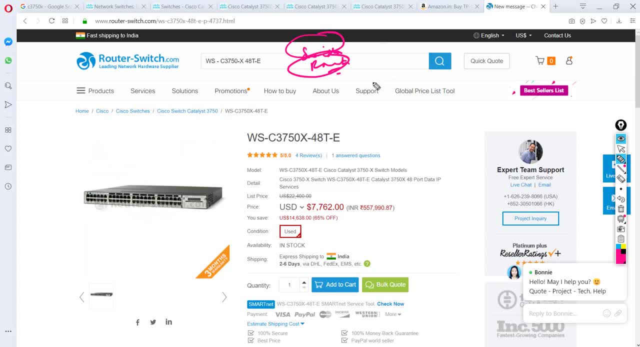 he is going to ask which variant in the switch or which variant in router so you switch or which variant in router so you switch or which variant in router. so you should at least know two three different, should at least know two three different, should at least know two three different names or two three different platform. 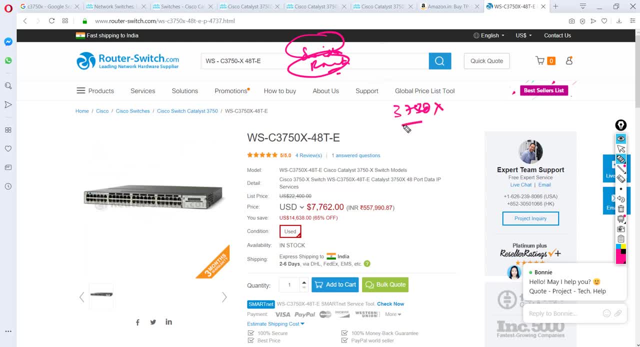 names, or two three different platform names, or two three different platform. you can say that i have worked on 3750x. you can say that i have worked on 3750x. you can say that i have worked on 3750x, which is a stackable device. 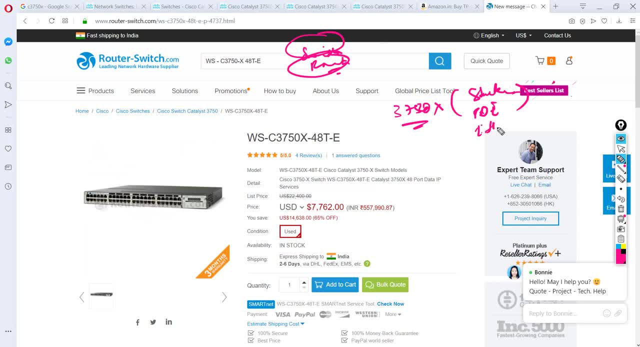 which is a stackable device, which is a stackable device which is a poe capable, which is ethernet, which is a poe capable, which is ethernet, which is a poe capable, which is ethernet, uh type which which has 48 ports, so, uh type which which has 48 ports, so 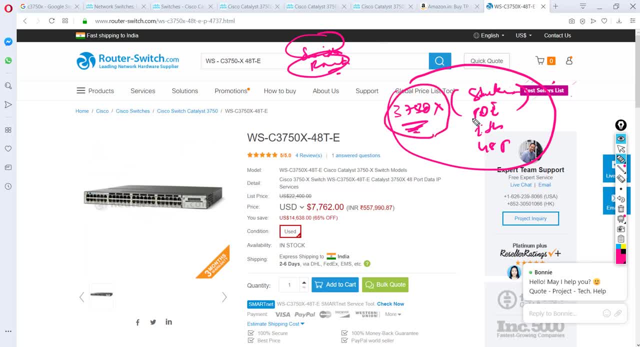 uh type, which which has 48 ports. so, basically, they are expecting you to, basically, they are expecting you to, basically, they are expecting you to explain the hardware um properties. okay, explain the hardware um properties. okay, explain the hardware um properties. okay, same way, you should know few things in. 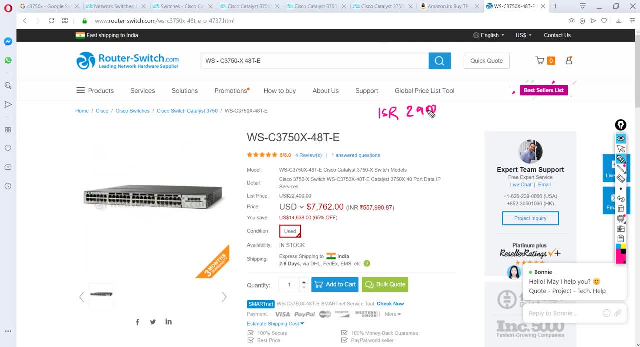 same way you should know few things, in same way you should know few things in router. you can call router, you can call router, you can call. you can remember one of them- isr 2900. you can remember one of them, isr 2900. you can remember one of them, isr 2900. this is integrated service router. okay. 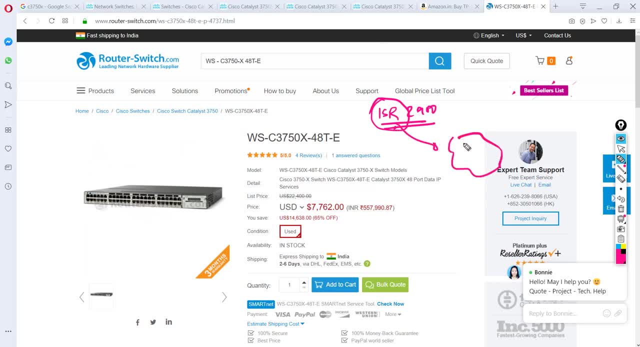 this is integrated service router. okay, this is integrated service router. okay, it is used for a small office, just for it is used for a small office, just for it is used for a small office, just for connecting internet. okay, you should connecting internet. okay, you should connecting internet. okay, you should know the feature, how. what is 2900? 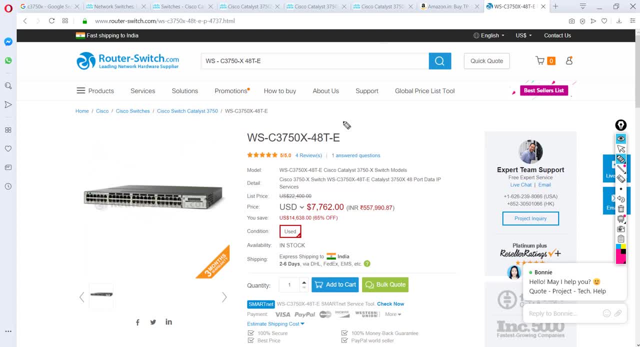 know the feature, how. what is 2900? know the feature how. what is 2900 capable of okay, capable of okay, capable of okay. so this is very important topic both in. so this is very important topic both in. so this is very important topic both in terms of uh interview and also when 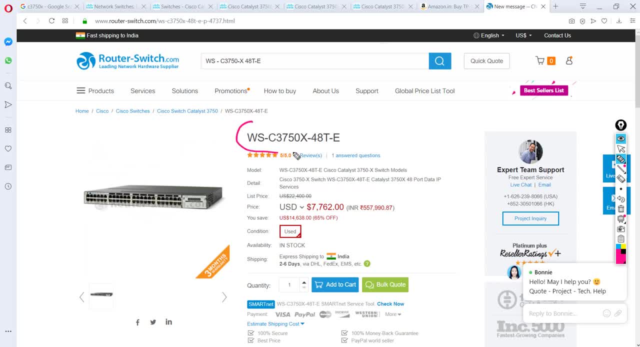 terms of uh interview and also when. terms of uh interview, and also when you're designing the network. okay, you're designing the network. okay, you're designing the network, okay. so, regards to, so, regards to, so, regards to the features they have given us, the features they have given us. 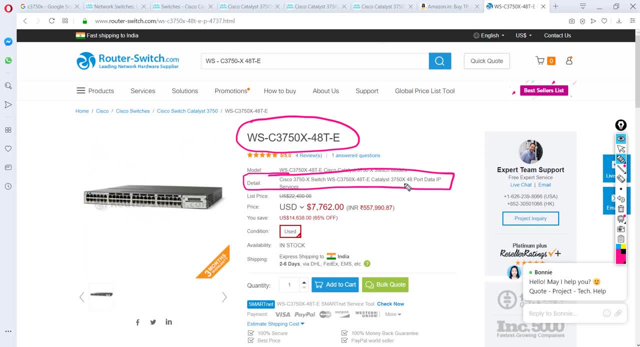 the features they have given us. few things here, okay. few things here, okay. few things here, okay. like it's a catalyst 37x. like it's a catalyst 37x. like it's a catalyst 37x 48 port ip services. so this ip services. 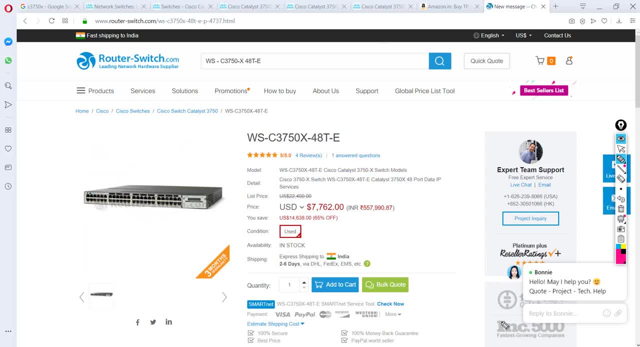 48 port ip services. so this ip services- 48 port ip services- so this ip services- is again a something new, okay, which we is again a something new, okay, which we is again a something new, okay, which we should understand, should understand, should understand. so let me tell you what it means. 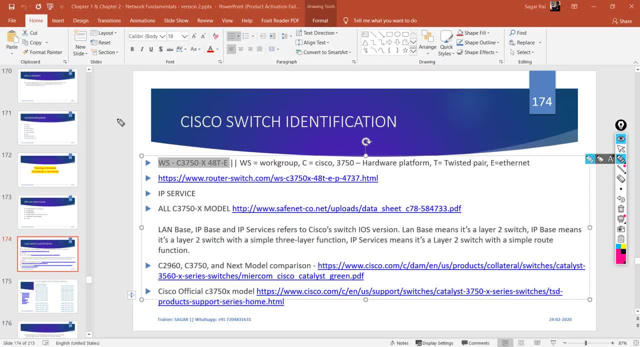 so let me tell you what it means. so let me tell you what it means: refers to okay, refers to okay, refers to okay. so basically a cisco, so basically a cisco, so basically a cisco platform. anything a cisco switch platform, anything a cisco switch. 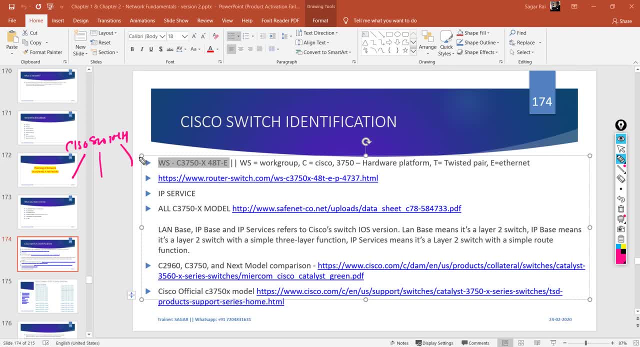 platform, anything, a cisco switch, okay. so basically they come in, okay. so basically they come in okay. so basically they come in three variants. okay, the first one is three variants. okay, the first one is three variants. okay, the first one is called as lan. called as lan. 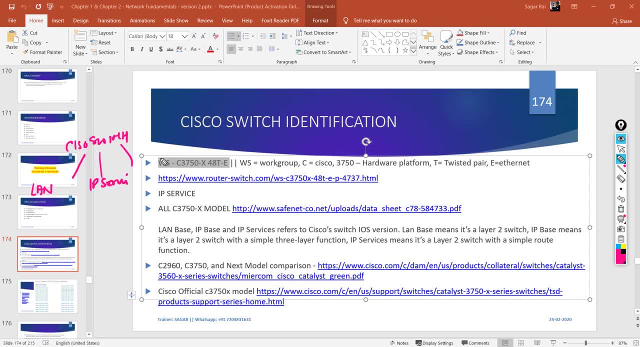 called as lan. second is called as ip services, and second is called as ip services, and second is called as ip services and third one is called as ip base. third one is called as ip base. third one is called as ip base. okay, so lan is something which we can. 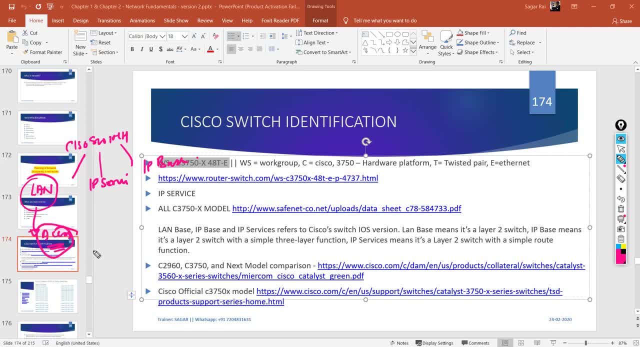 okay. so lan is something which we can. okay, so lan is something which we can use only for access purpose. access layer. use only for access purpose. access layer. use only for access purpose. access layer. purpose okay, purpose okay, purpose okay, which can only understand mac, which can only understand mac. 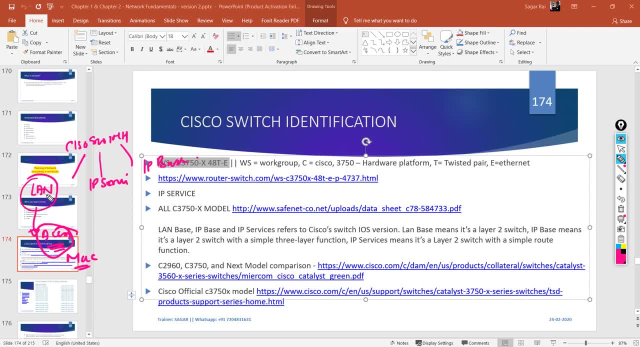 which can only understand mac. so, basically, if you want to connect it, so basically, if you want to connect it. so basically, if you want to connect it, uh to different computers, if you want to uh to different computers, if you want to uh to different computers, if you want to have a switch which can connect different, 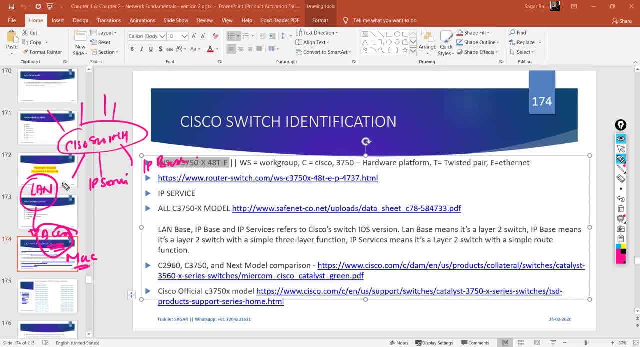 have a switch which can connect different. have a switch which can connect different computers and computers and computers and no routing features. then you can buy the no routing features. then you can buy the no routing features. then you can buy the land fee, land based, land fee, land based. 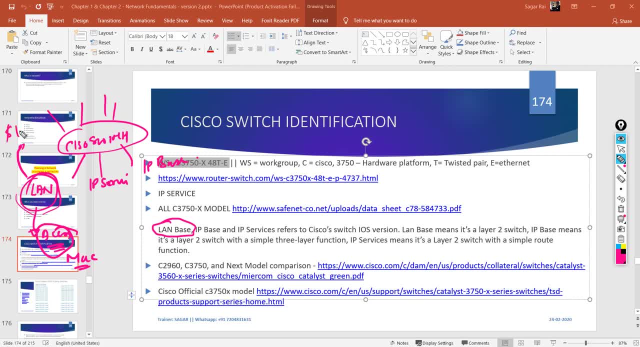 land fee, land based switches: okay, basically they will cost switches. okay, basically they will cost switches. okay, basically they will cost very uh, very uh, very uh. less in the market like a hundred dollars. less in the market like a hundred dollars. less in the market like a hundred dollars to like five hundred dollars. 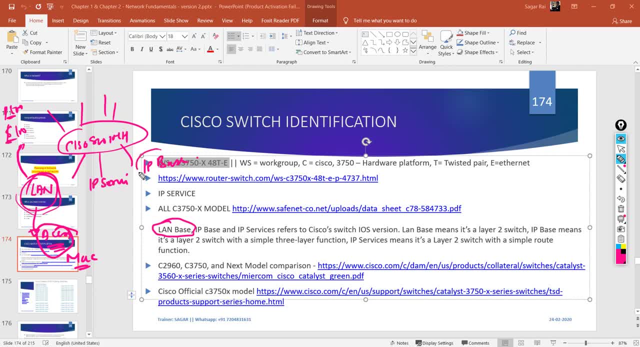 to like five hundred dollars. to like five hundred dollars- okay, it will serve the purpose. whereas ip- okay, it will serve the purpose. whereas ip- okay, it will serve the purpose, whereas ip base, base, base is again a switch, is again a switch, is again a switch. but it can understand little bit of. 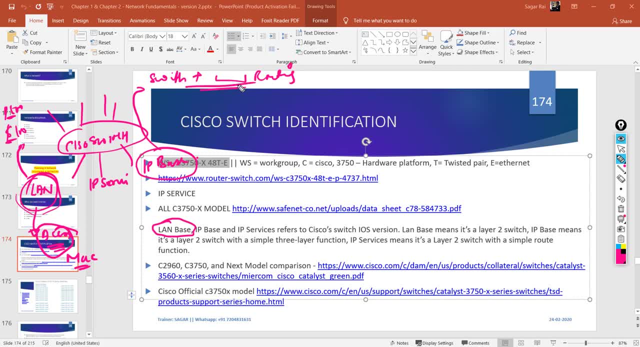 but it can understand little bit of- but it can understand little bit of- routing, routing, routing- okay, a very small number of routing. okay, a very small number of routing. okay, a very small number of routing, which which is required, which which is required, which which is required, in a small 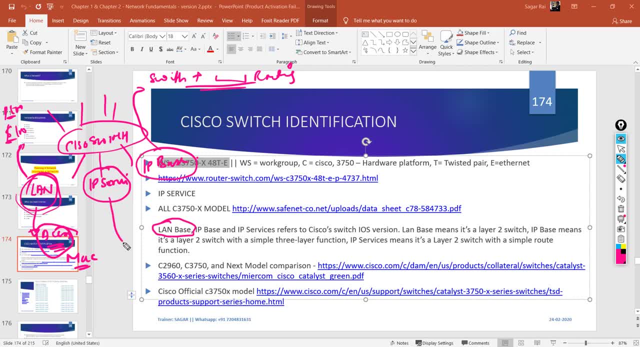 in a small, in a small network design. okay. the third one is ip network design. okay, the third one is ip network design. okay. the third one is ip services, services, services which, which, which, along with switch, it can understand, along with switch, it can understand, along with switch, it can understand, routing. 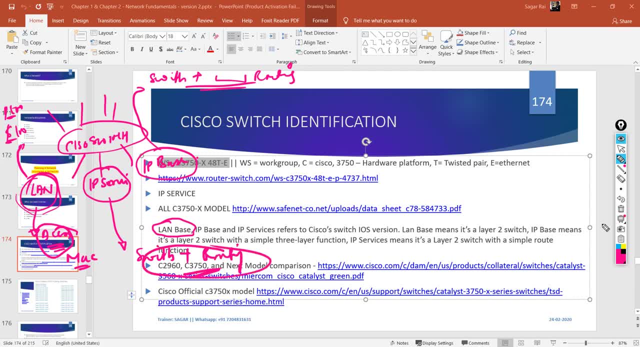 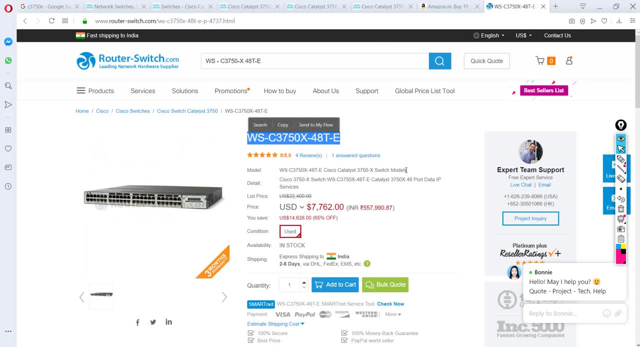 routing, routing also okay. so these are three different, also okay. so these are three different also okay. so these are three different variants. and if you variants, and if you variants, and if you go back to the website, the one which are we looking for it is ip. the one which are we looking for it is ip. 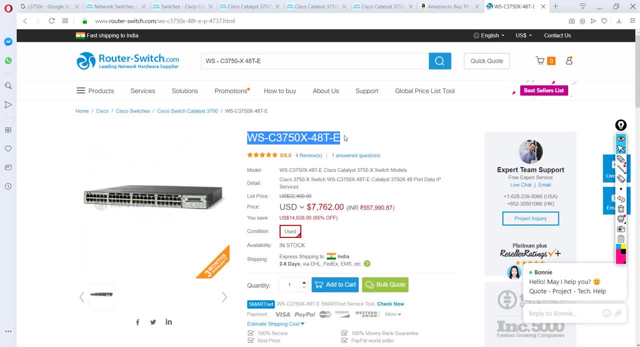 the one which are we looking for. it is ip services. that means services, that means services, that means this device, this device, this device can do the work of switch and it can can do the work of switch and it can can do the work of switch and it can also do the work of a routing, okay. so, 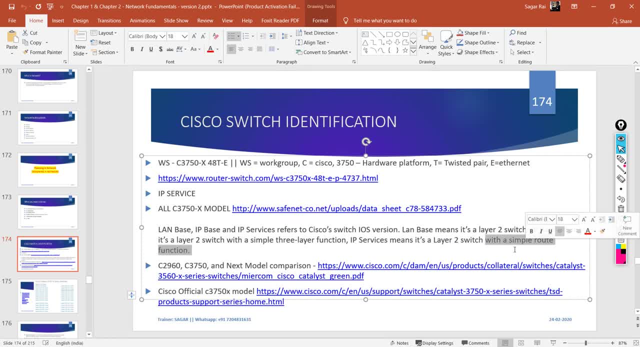 also do the work of a routing, okay. so also do the work of a routing, okay. so basically, it can be, basically it can be, basically it can be doing a work of routing as well, okay, doing a work of routing as well, okay, doing a work of routing as well, okay. so that was regards to the platform that. 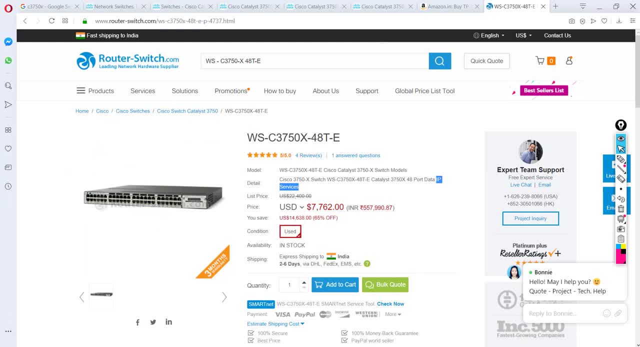 so that was regards to the platform. that, so that was regards to the platform that was regards to this complete switch. so was regards to this complete switch. so was regards to this complete switch. so now you have, now you have, now you have some understanding, some understanding, some understanding of your requirement. so if someone is 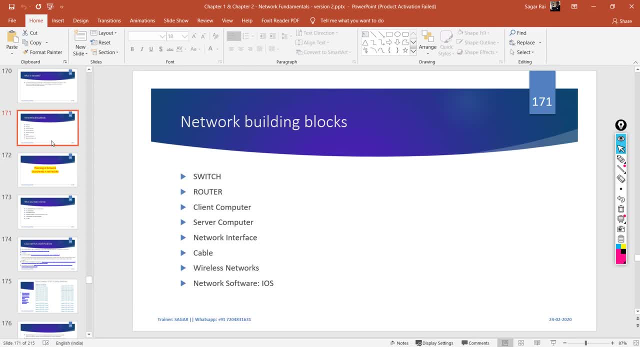 of your requirement. so if someone is of your requirement, so if someone is giving you, uh giving you the giving you, uh giving you the giving you, uh giving you the requirement, requirement, requirement, okay, so first thing is you have to. okay, so first thing is you have to. 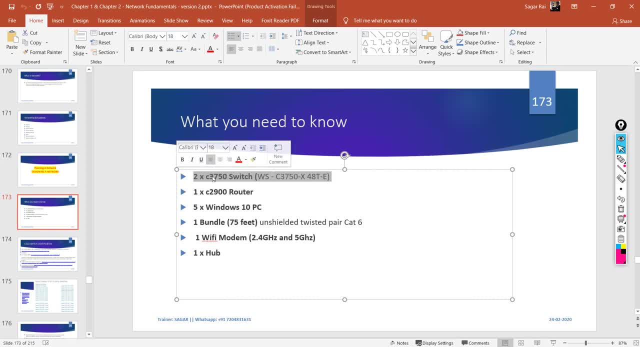 okay. so first thing is, you have to study the hardware. okay, you should study the hardware. okay, you should study the hardware. okay, you should understand what, what type of device that understand what, what type of device that understand what, what type of device that is is is. the next one is c2900. okay, 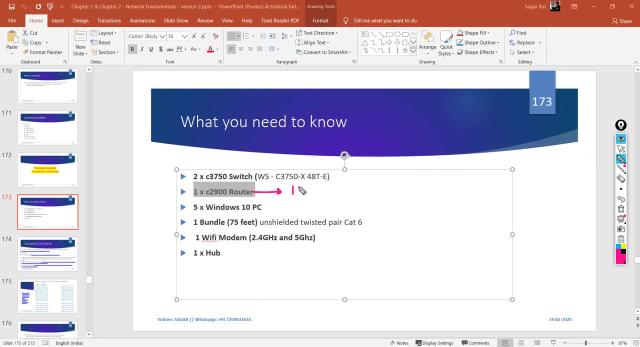 the next one is c2900- okay. the next one is c2900- okay. which is a router. which is a router. which is a router- okay. it is a isr router, integrated- okay. it is a isr router, integrated- okay. it is a isr router, integrated service router- okay. 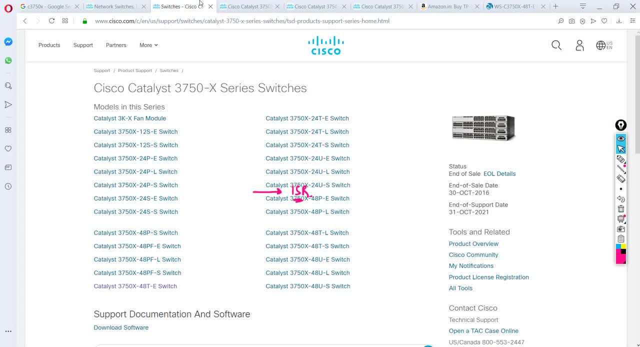 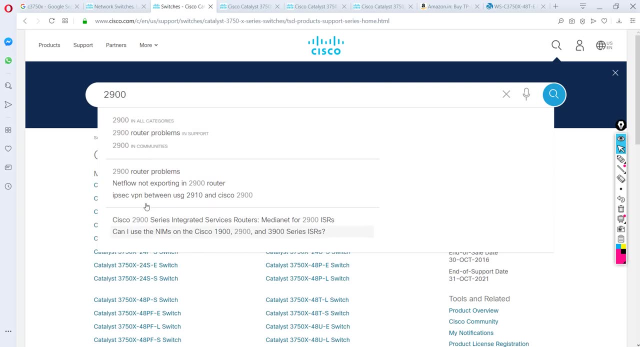 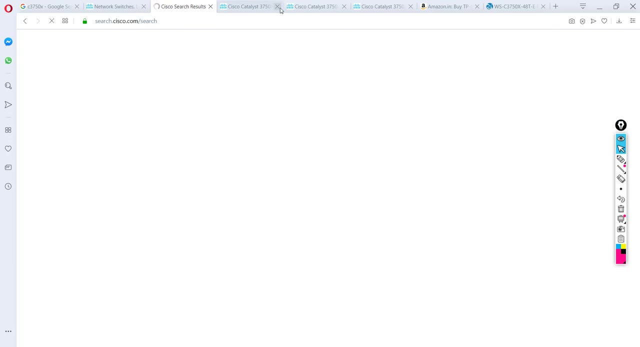 service router. okay, service router okay. so let's check out 2900 quickly. so let's check out 2900 quickly. so let's check out 2900 quickly. let me type 2900, let me type 2900, let me type 2900 okay. 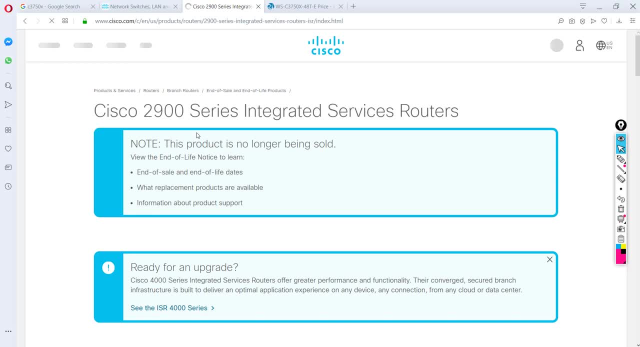 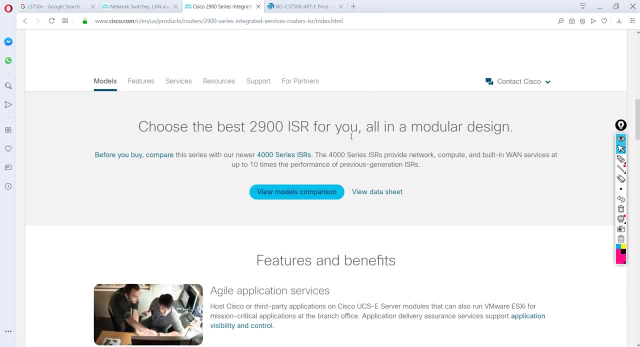 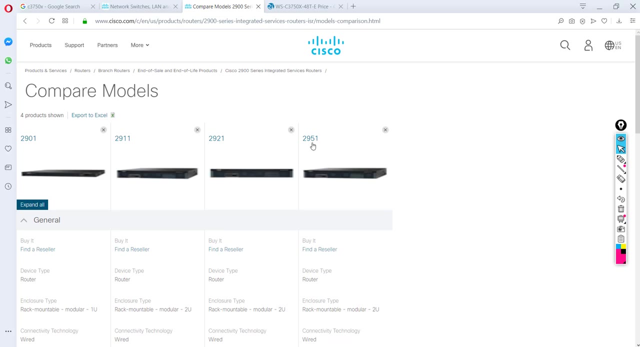 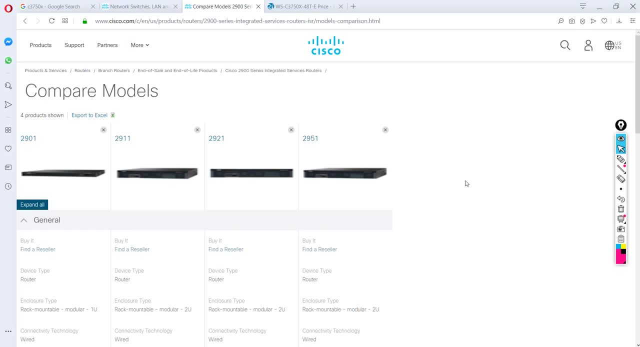 different variants: okay, two, nine, zero, one. different variants: okay, two, nine zero, one. two, nine one one, two. nine, two, one, two, two, nine one, one, two, nine, two, one, two, two, nine one, one, two, nine, two, one, two. nine five, one okay. nine five, one okay. nine five, one okay. and then they have their own features. 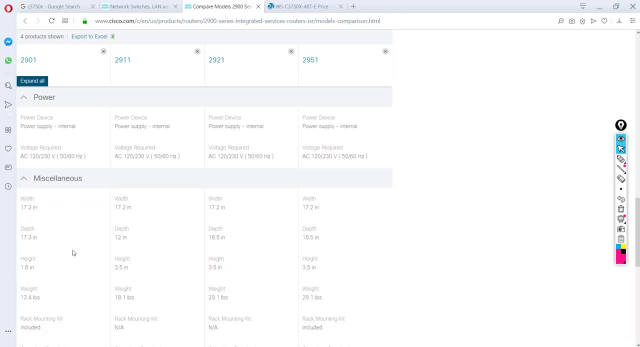 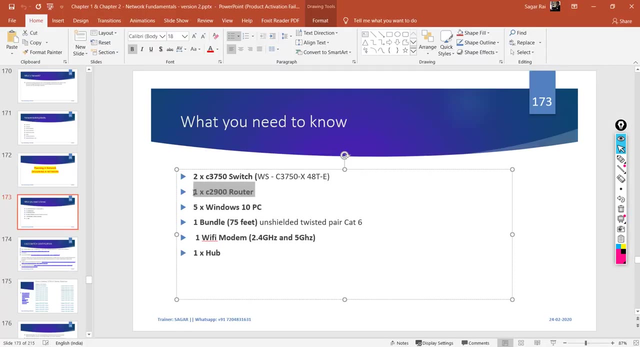 and then they have their own features, and then they have their own features listed here, listed here, listed here with all different types. okay, with all different types. okay, with all different types. okay, so customer has not given us any. so customer has not given us any. so customer has not given us any requirement. okay, he has not given us any. 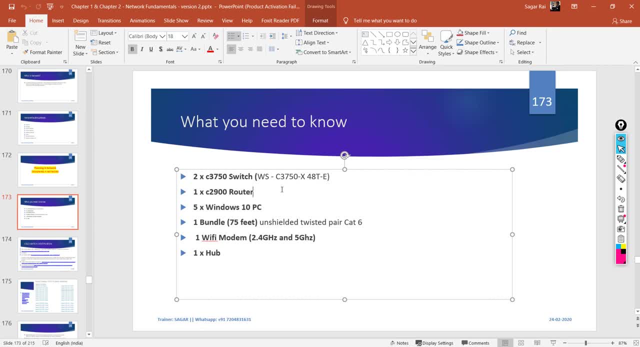 requirement. okay, he has not given us any requirement. okay, he has not given us any variant. so that means we are good to variant. so that means we are good to variant. so that means we are good to make our own wise decision. okay, which make our own wise decision? okay, which. 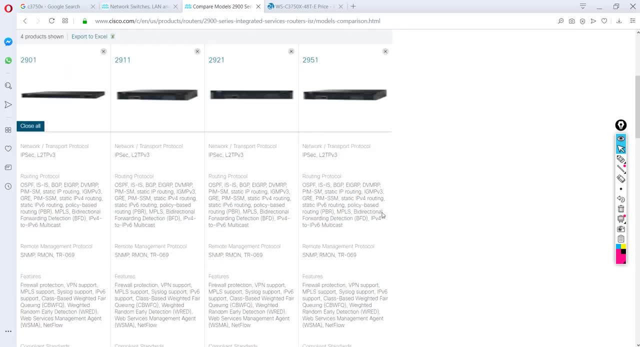 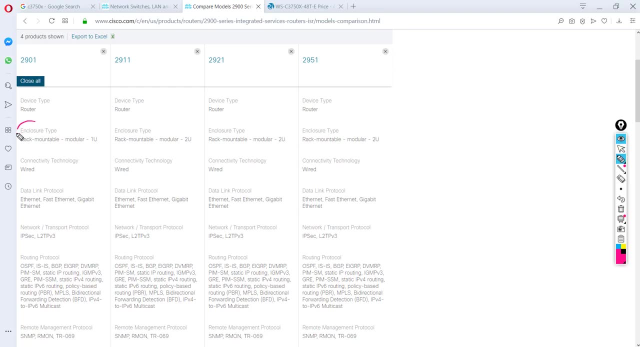 make our own wise decision. okay, which can fit into its uh. fit into its uh his can fit into its uh. fit into its uh. his can fit into its uh. fit into its uh his uh network. okay, uh network, okay, uh network, okay, so, so. so now we will check the things like: 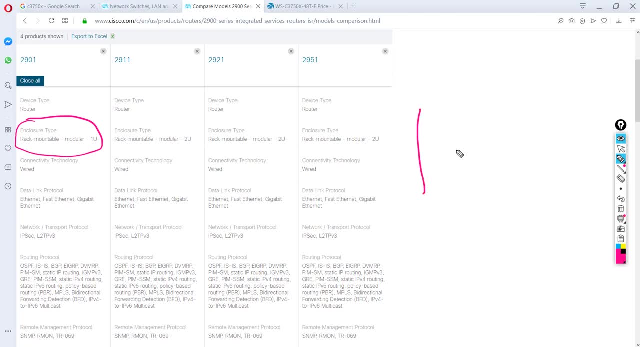 now we will check the things like. now. we will check the things like: what is it capable of? it's rack mountable? what is it capable of it's rack mountable? what is it capable of? it's rack mountable? that means if you have rack, you can plug. 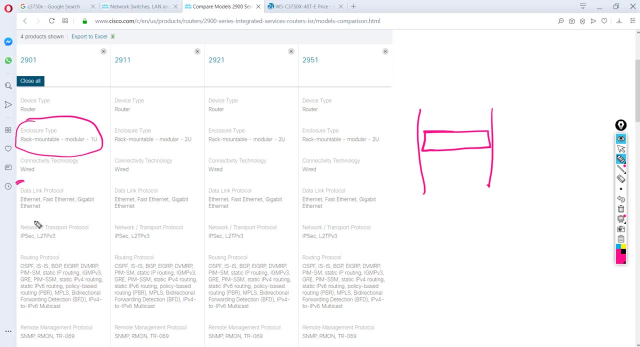 that means, if you have rack, you can plug. that means, if you have rack, you can plug it. okay, along with other devices. it's it okay along with other devices. it's it okay along with other devices. it's wired supported. it has fast ethernet wired supported. it has fast ethernet. 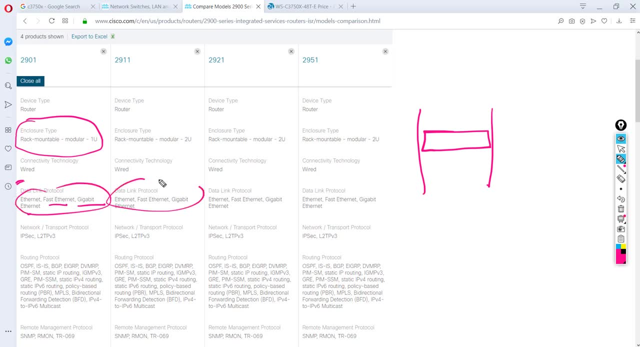 wired supported. it has fast ethernet, giga ethernet- okay, which is supported by giga ethernet- okay, which is supported by giga ethernet. okay, which is supported by all of them. so that is fine with me. okay, all of them. so that is fine with me. okay, all of them. so that is fine with me. okay, we have the transport protocol same. 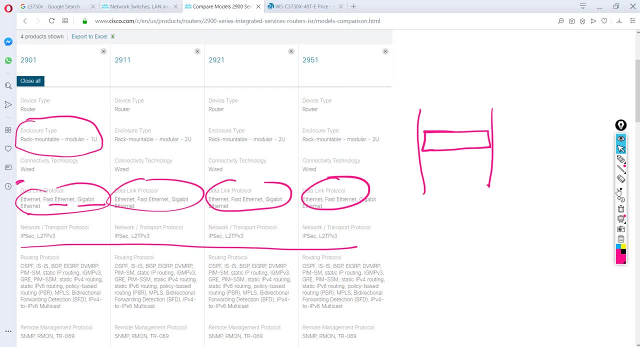 we have the transport protocol: same. we have the transport protocol same everywhere. it supports all the major routing. it supports all the major routing. it supports all the major routing. protocol, protocol, protocol. okay, so that is a good thing, so basically, okay, so that is a good thing, so basically, 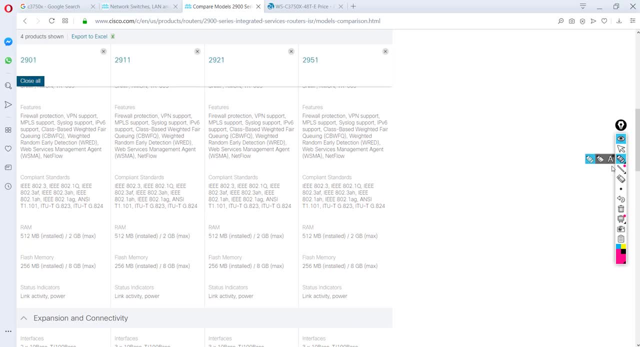 okay, so that is a good thing. so, basically, they are all with, they are all with, they are all with similar configuration. okay, so might be similar configuration. okay, so might be similar configuration. okay, so might be. there can be little bit of uh. there can be little bit of uh. 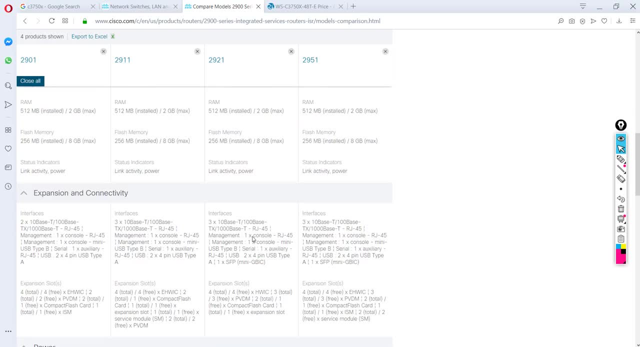 there can be little bit of uh hardware, um hardware, um hardware, um things which might change like for things which might change like for things which might change like. for example, here it says 2 into 10 base t. example: here it says 2 into 10 base t. 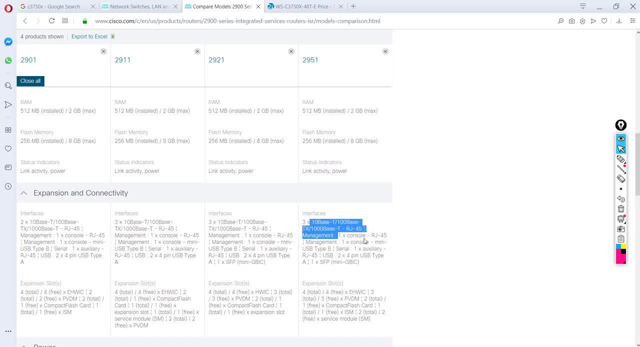 example, here it says 2 into 10 base t interface, whereas here it is three it's interface, whereas here it is three it's interface, whereas here it is three, it's three and it's three, okay, three and it's three, okay, three and it's three. okay, now expansion slot. so it's. 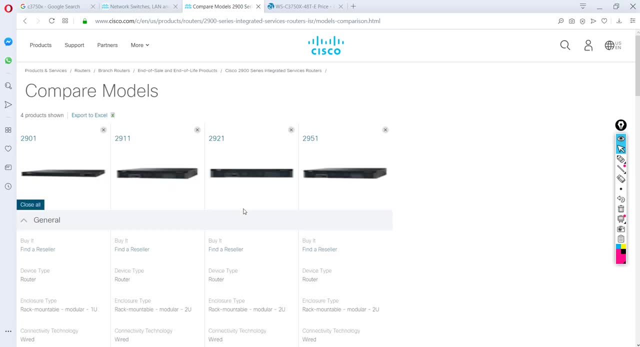 now expansion slot, so it's now expansion slot, so it's over here. so basically, depending upon over here, so basically depending upon over here. so basically depending upon the hardware. the things are different here, the hardware. the things are different here. the hardware. the things are different here. okay, the feature wise, it is going to. 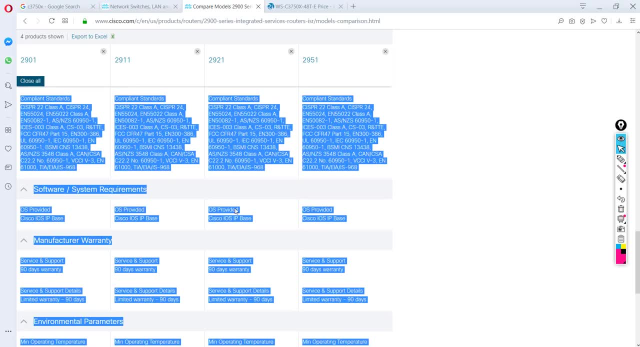 okay, the feature wise, it is going to okay, the feature wise, it is going to be same. so now, as a design engineer, it is be same. so now, as a design engineer, it is be same. so now, as a design engineer, it is all up to you if, if you are okay with. 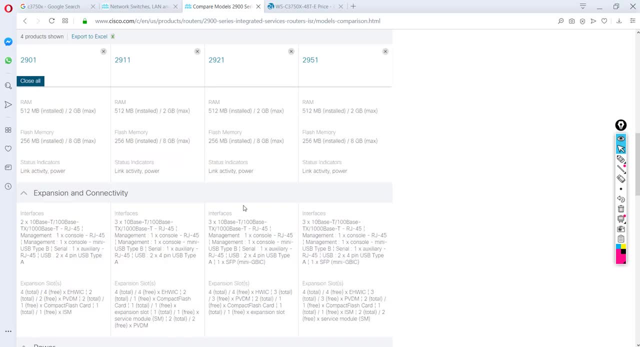 all up to you. if, if you are okay with, all up to you, if, if you are okay with the uh features and the hardware is the uh features and the hardware is the uh features and the hardware is really not mattering you or bothering, really not mattering you or bothering. 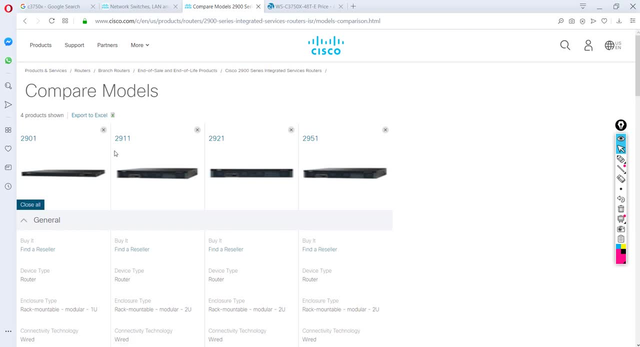 really not mattering you or bothering you. so then you are good with buying you. so then you are good with buying you. so then you are good with buying one of them. okay, so, whichever you're one of them, okay. so, whichever you're one of them, okay. so, whichever you're buying, but make sure that you learn. 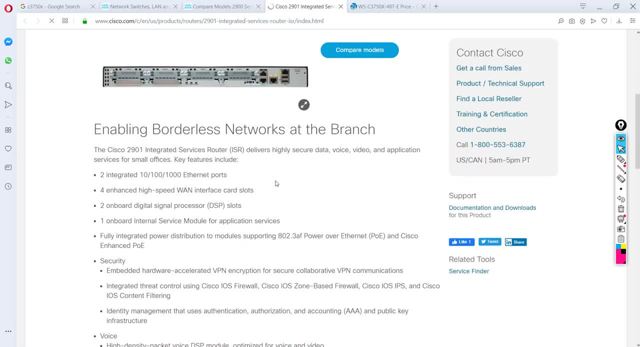 buying. but make sure that you learn buying. but make sure that you learn that okay, because next day, if something, that okay. because next day, if something, that okay. because next day if something breaks up, they're going to call you and breaks up, they're going to call you and. 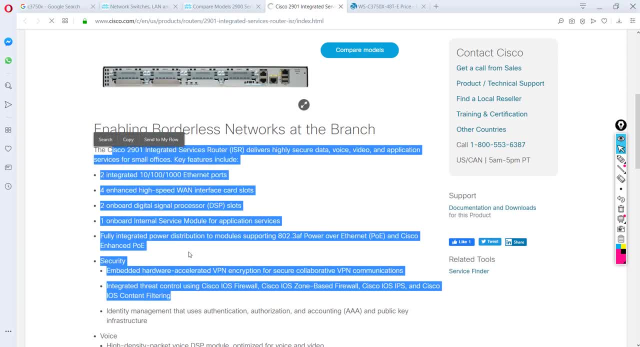 breaks up, they're going to call you and then you have to fix it. okay, so it is. then you have to fix it. okay, so it is. then you have to fix it. okay, so it is better. you read everything about that better. you read everything about that. 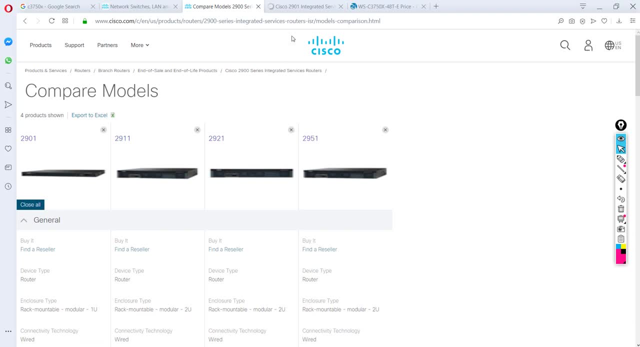 better you read everything about that particular model. you don't have to read particular model. you don't have to read particular model. you don't have to read all of four, all the four. okay if you're all of four, all the four. okay if you're all of four, all the four. okay. if you're trying to integrate two zero nine one. 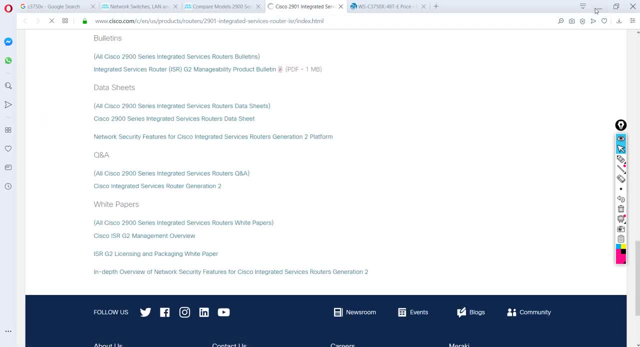 trying to integrate two zero nine one. trying to integrate two zero nine one. so then you should know what it is. so then you should know what it is, so then you should know what it is: supported okay, supported, okay, supported, okay, so, so, so, we are good with this, we are good with 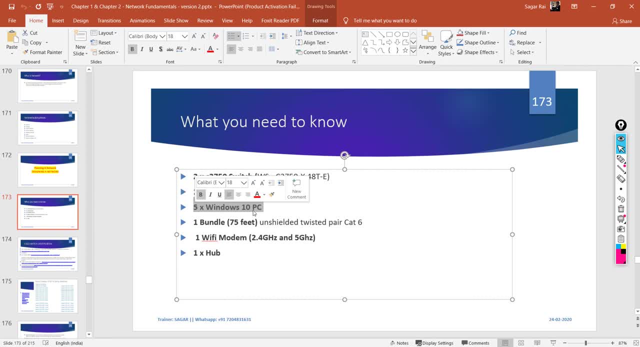 we are good with this. we are good with. we are good with this. we are good with the switch windows computer. you can just the switch windows computer. you can just the switch windows computer. you can just uh buy from amazon or something. okay if uh buy from amazon or something. okay. if 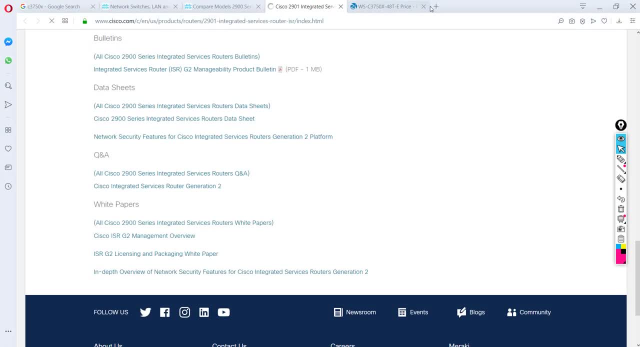 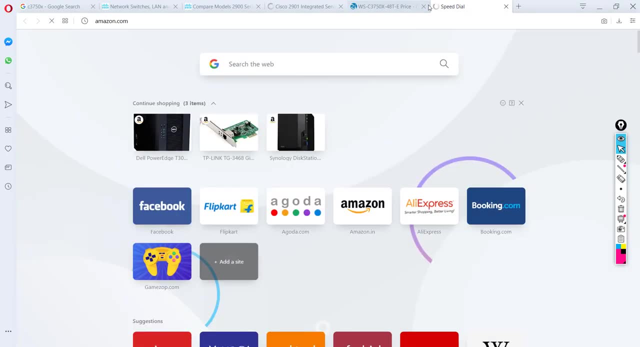 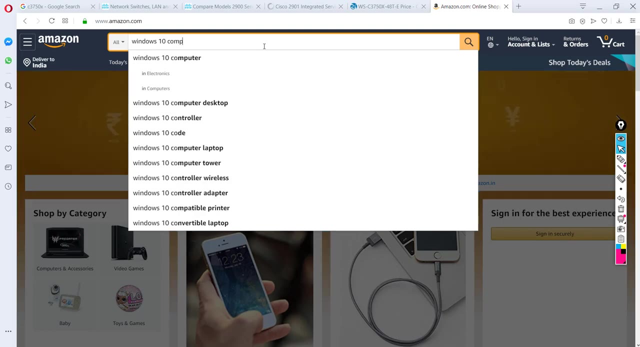 uh, buy from amazon or something. okay, if you go to amazon, you you can search for the best, uh, reasonable. search for the best, uh, reasonable. search for the best, uh, reasonable. computer, computer: computer okay, windows 10 computer okay, and then you can make a wise computer. okay, and then you can make a wise. 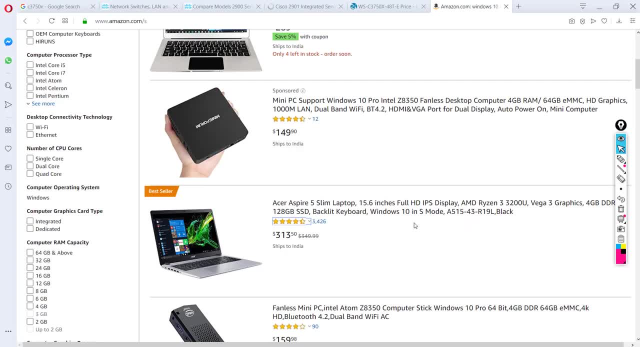 computer, okay, and then you can make a wise decision: what decision, what decision? what ram you want? what um ram you want? what um ram you want? what um features you want? what is the graphic features you want? what is the graphic features you want? what is the graphic card that you want and you can purchase? 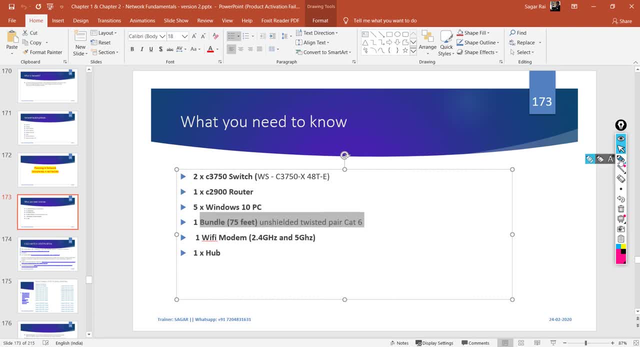 card that you want and you can purchase card that you want and you can purchase that, that, that twisted cable pair. you all know that twisted cable pair. you all know that twisted cable pair. you all know that there are three. there are three. there are three majorly used cables nowadays. okay, 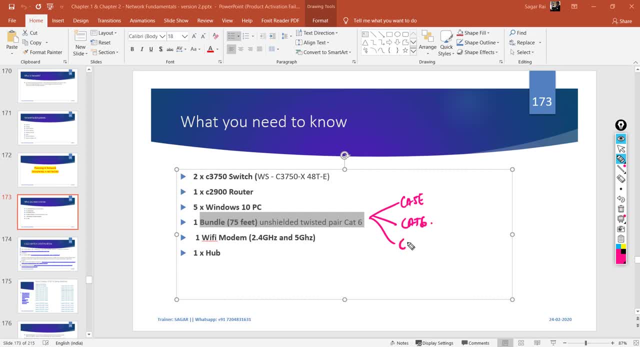 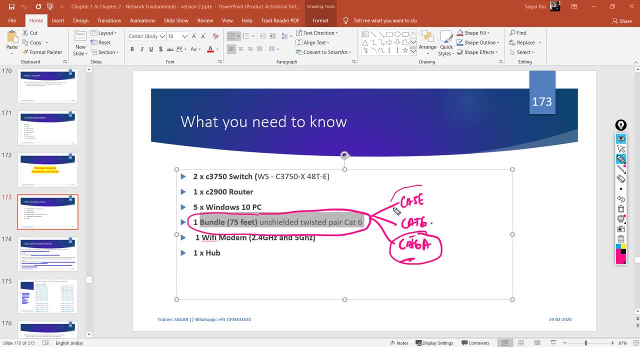 a. okay, so you can again go with the? a. okay, so you can again go with the latest one. okay, in case you want to save latest one. okay, in case you want to save latest one. okay, in case you want to save some money, then you can go with cat 5 or. 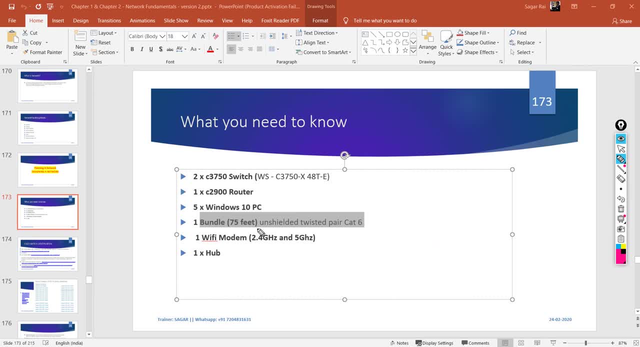 some money, then you can go with cat 5. or some money, then you can go with cat 5, or otherwise you can go with cat 6 a okay. otherwise you can go with cat 6 a okay. otherwise you can go with cat 6 a okay. and a Wi-Fi modem say: let's, we have a. 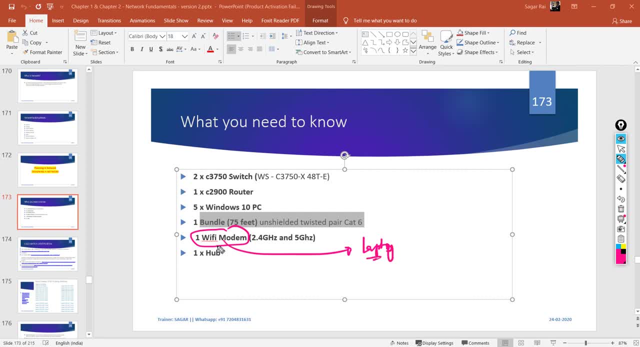 and a Wi-Fi modem, say, let's, we have a and a Wi-Fi modem say, let's, we have a laptop user who want to connect via Wi-Fi, laptop user who want to connect via Wi-Fi, laptop user who want to connect via Wi-Fi modem. so we need one Wi-Fi modem. so we modem. so we need one Wi-Fi modem. so we modem, so we need one Wi-Fi modem. so we can go with some Cisco Wi-Fi modem, or I can go with some Cisco Wi-Fi modem, or I can go with some Cisco Wi-Fi modem, or I can go with it TP link or Linksys, right, 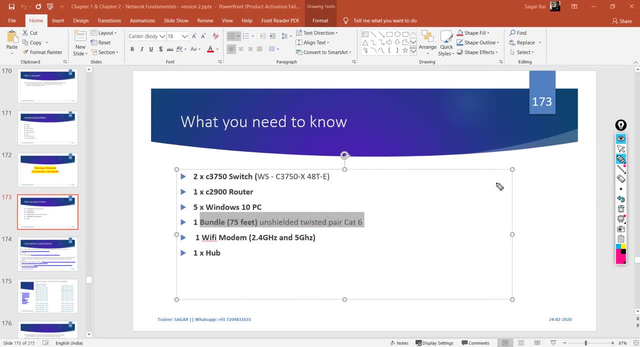 can go with it TP link or Linksys right can go with it- TP link or Linksys right, there are so many in the market and one there are so many in the market and one there are so many in the market and one hub. let's say we have a computer user. 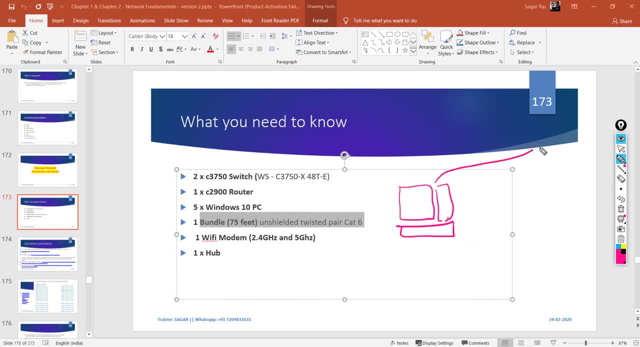 hub. let's say we have a computer user hub. let's say we have a computer user okay, who is connected to a switch. but okay, who is connected to a switch? but okay, who is connected to a switch, but he's having some other IP devices. let's: 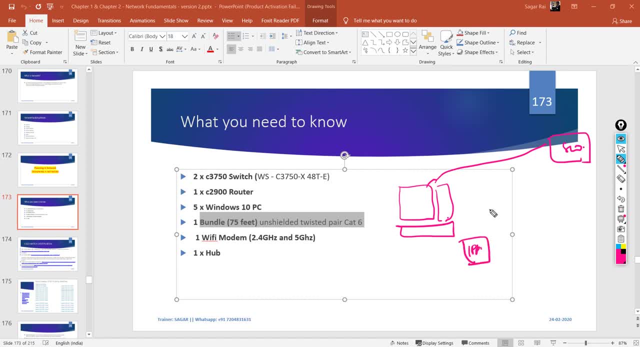 he's having some other IP devices. let's he's having some other IP devices. let's say he has IP printer on his desk, or a say he has IP printer on his desk, or a say he has IP printer on his desk, or a scanner, IP scanner. so basically he is. 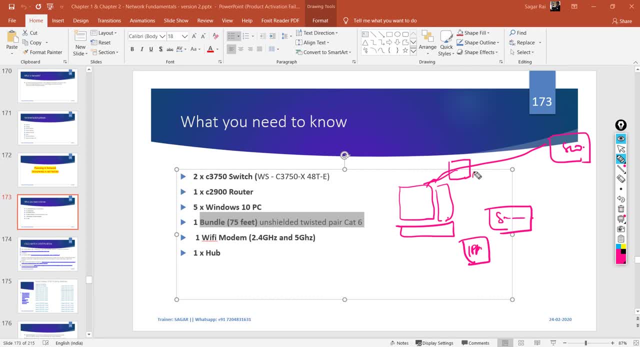 scanner, IP scanner. so basically he is scanner, IP scanner. so basically he is getting only one connection. so what? he getting only one connection. so what he getting only one connection. so what he can do is he can connect hub over here. can do is he can connect hub over here. 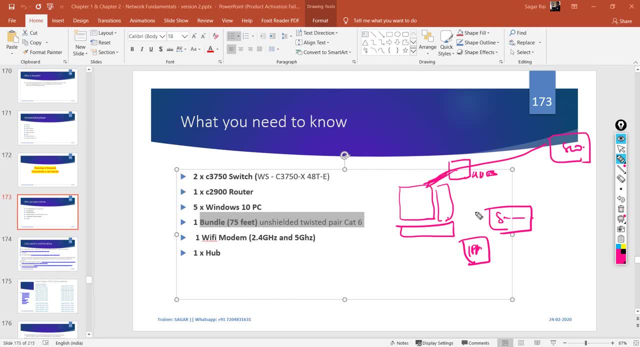 can do is he can connect hub over here and from hub. he can take one input to and from hub. he can take one input to and from hub. he can take one input to himself, one input to IP machine and one himself. one input to IP machine and one. 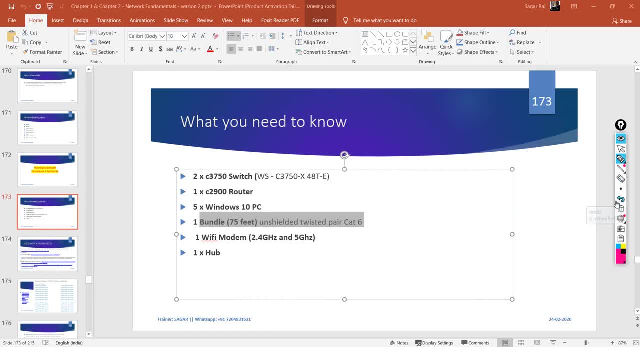 himself: one input to IP machine and one to the scanner, and that is how he can to the scanner, and that is how he can to the scanner and that is how he can connect it. okay, so now we know all the connect it. okay, so now we know all the. 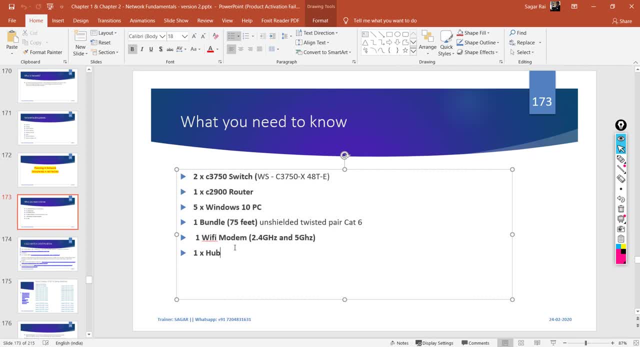 connect it. okay, so now we know all the hardware features and functionality: okay. hardware features and functionality: okay. hardware features and functionality: okay, so we should be good enough to design. so we should be good enough to design. so we should be good enough to design now. okay, we discussed this, we also. 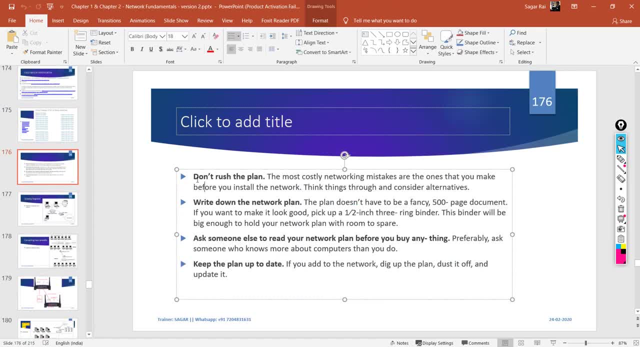 now, okay, we discussed this. we also now, okay, we discussed this. we also discussed about the variance. okay, now discussed about the variance. okay, now discussed about the variance. okay, now. regards to decision-making: okay, first regards to decision-making. okay, first regards to decision-making. okay, first thing, don't rush. okay, yo, you are. 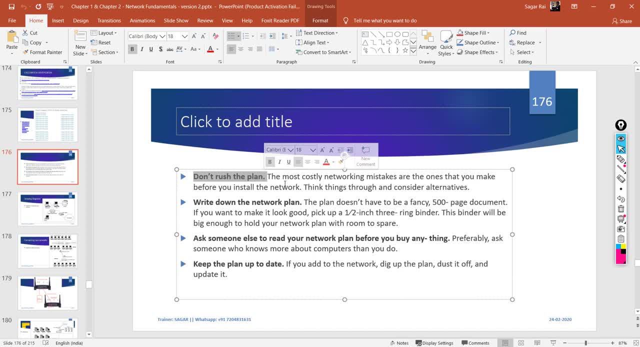 thing don't rush, okay yo, you are thing don't rush, okay yo. you are designing the network, which is going to designing the network, which is going to designing the network which is going to last for couple of years- might be for last- for couple of years, might be for. 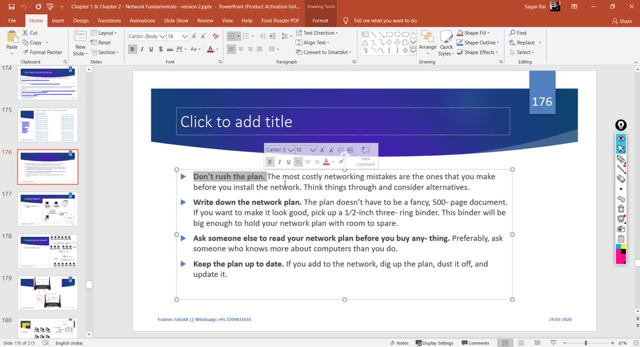 last for couple of years, might be for next 10, 20 years. so think of the future, next 10, 20 years. so think of the future, next 10, 20 years. so think of the future and then prepare a network design- don't. and then prepare a network design- don't. 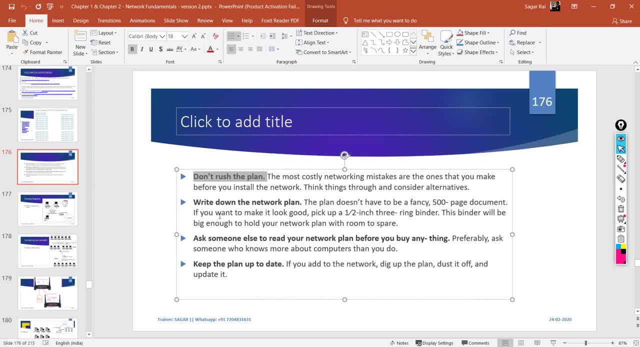 and then prepare a network design. don't, don't don't find out a shortcut. okay, don't don't find out a shortcut. okay, don't don't find out a shortcut, okay, document the network plan. whatever you document the network plan, whatever you document the network plan, whatever you are planning, draw it on on a paper or 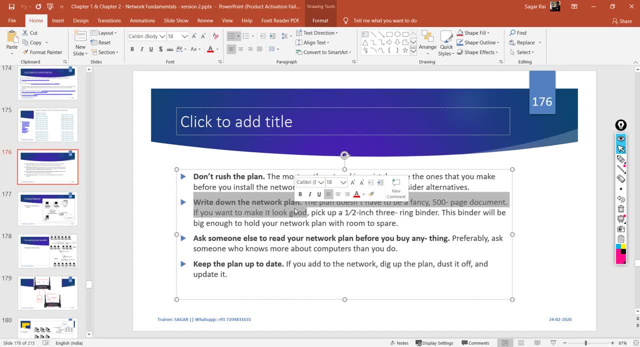 are planning draw it on on a paper or are planning draw it on some software so that you have a draw it on some software, so that you have a draw it on some software, so that you have a documented plan so which you can send, documented plan so which you can send. 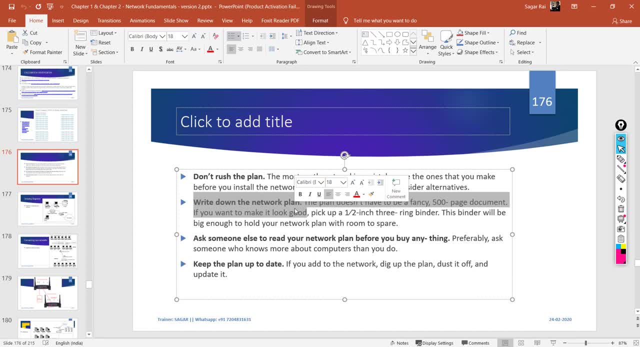 documented plan, so which you can send it to the floor engineers, or the cable it to the floor engineers, or the cable it to the floor engineers, or the cable vendors, because they are the one who is vendors, because they are the one who is vendors, because they are the one who is going to rack it, cable it and then give. 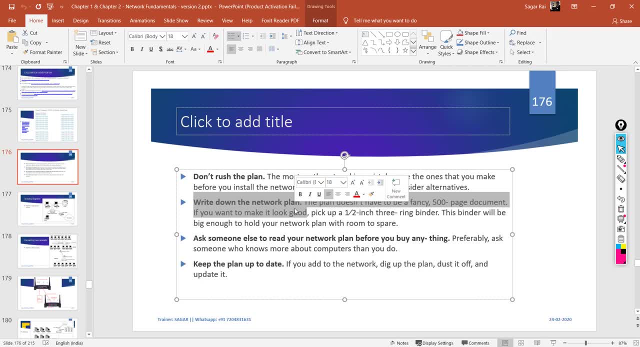 going to rack it, cable it and then give going to rack it, cable it and then give us the remote so that we can configure us the remote, so that we can configure us the remote, so that we can configure right, and once you do it, it's better. 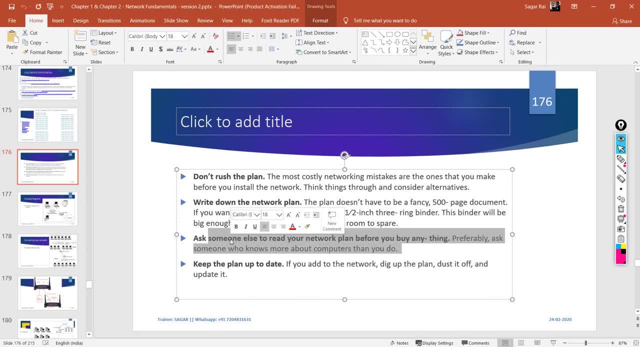 right and once you do it, it's better. right, and once you do it, it's better always to review the plan. okay, if you always to review the plan, okay, if you always to review the plan, okay, if you have any senior engineers or you have have any senior engineers or you have any network design engineer, better get. 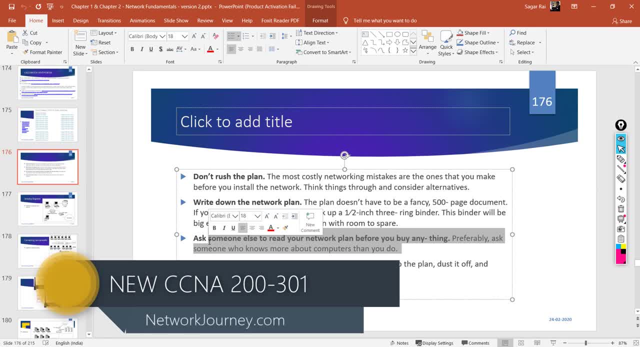 any network design engineer better get any network design engineer better get approved from them. okay, so, always, always approved from them. okay, so always, always approved from them. okay, so, always, always. it is advisable and keep it always it is advisable and keep it always it is advisable and keep it always updated. don't, don't go with some. 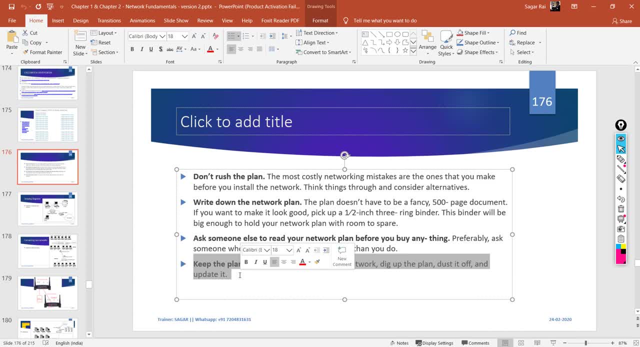 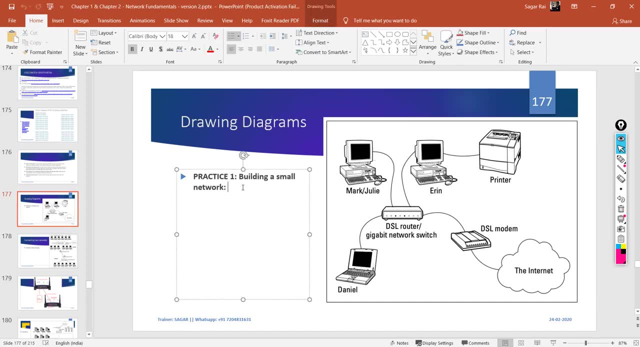 updated. don't don't go with some updated. don't don't go with some outdated things or something which outdated things or something which outdated things or something which upgradation is a complex process in upgradation is a complex process in upgradation is a complex process in future. and okay, fine. so this is the. 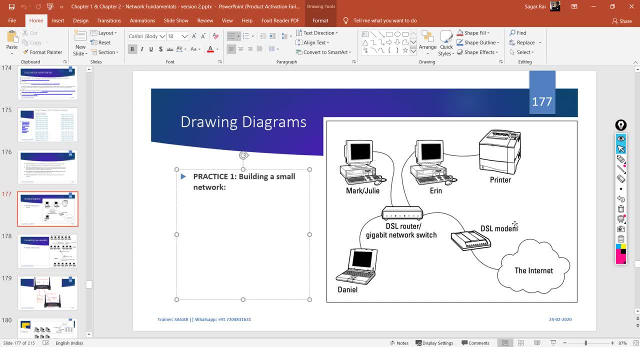 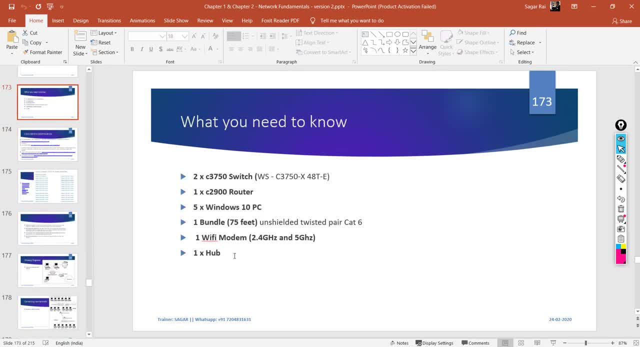 is the requirement which we have to do. it is the requirement which we have to do. it okay and same time. keep in the mind, okay, and same time, keep in the mind, okay, and same time, keep in the mind that these are the requirements two, that these are the requirements two. 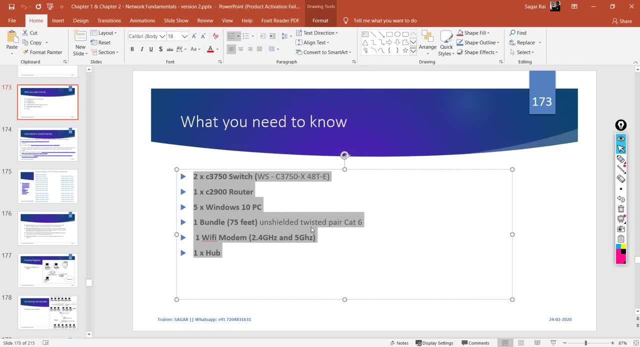 that these are the requirements: two switches, one router, five computers, 1k switches. one router, five computers, 1k switches. one router, five computers, 1k. one bundle of cable, one Wi-Fi model and one bundle of cable, one Wi-Fi model and one bundle of cable, one Wi-Fi model and one up. okay, so we can design a small. 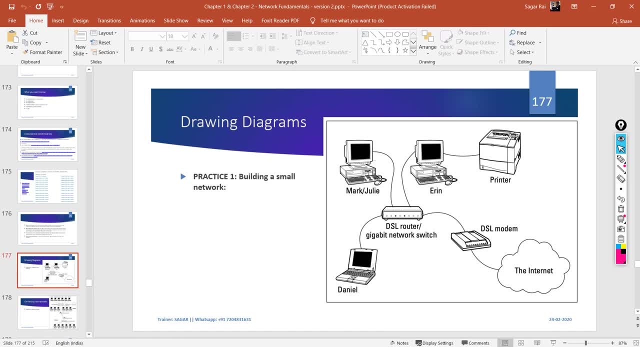 one up. okay, so we can design a small one up. okay, so we can design a small office. okay. so how can I design now? so office. okay. so how can I design now, so office. okay, so how can I design now? so there are plenty of software online. 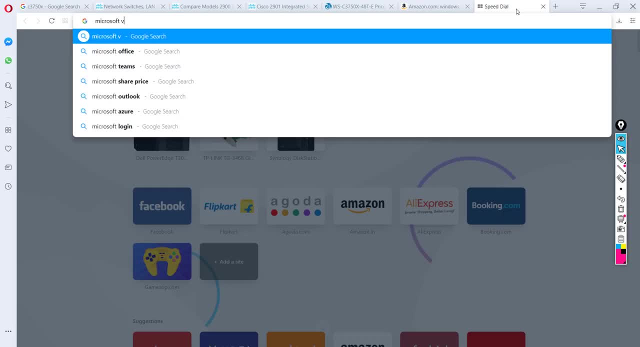 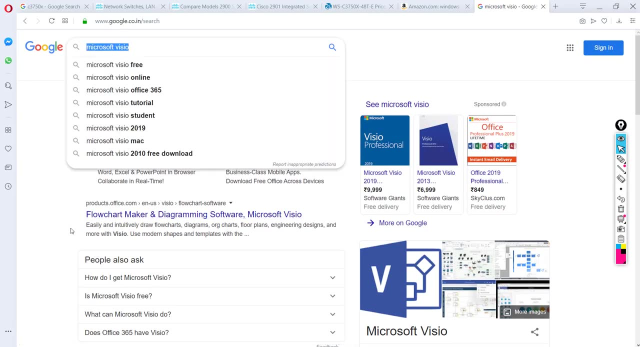 there are plenty of software online. there are plenty of software online. okay, like Microsoft vizio. okay, if you okay, like Microsoft vizio. okay, if you okay, like Microsoft vizio. okay, if you have Microsoft vizio, you can draw it. but have Microsoft vizio, you can draw it. but 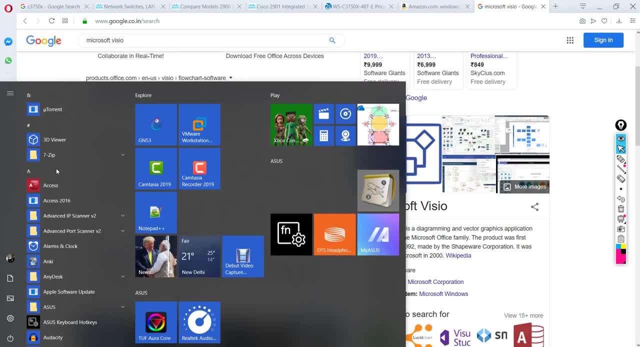 have Microsoft vizio. you can draw it, but it's a licensed version, so I have it. but it's a licensed version, so I have it. but it's a licensed version, so I have it. but since you guys might be stuck now, so since you guys might be stuck now, so 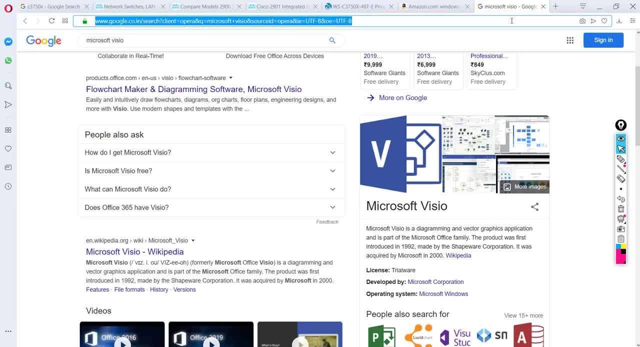 since you guys might be stuck now. so what I am going to do is I am going to. what I am going to do is I am going to. what I am going to do is I am going to make use of some free tool which you and make use of some free tool which you and. 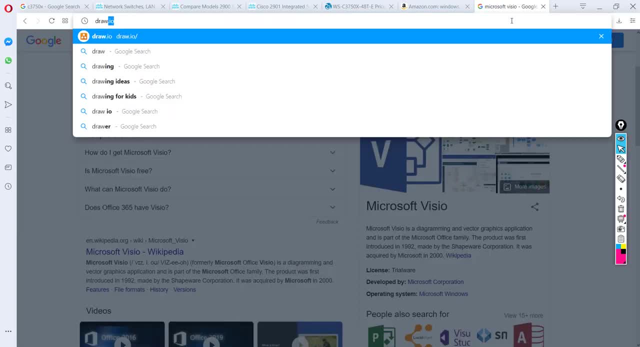 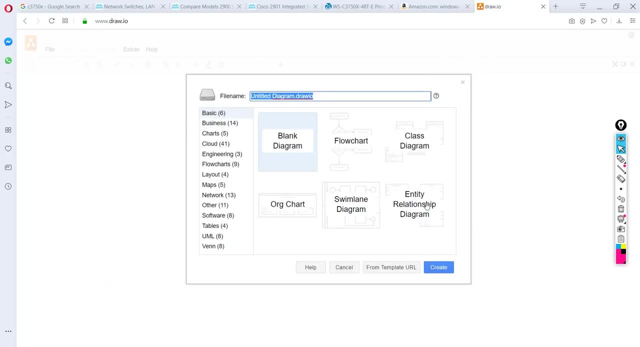 make use of some free tool which you and me can practice. okay, so that is me can practice. okay, so that is me can practice. okay, so that is drawio. so if you type this website, you drawio. so if you type this website, you drawio. so if you type this website, you can create some designs online. okay, so 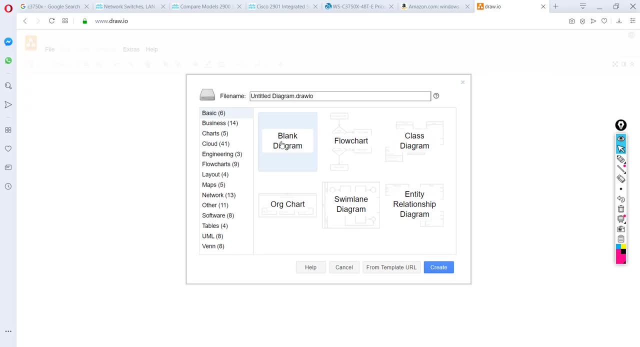 can create some designs online, okay. so can create some designs online, okay. so let's go with the blank diagram, click on. let's go with the blank diagram, click on. let's go with the blank diagram, click on create. and I am given this kind of page create and I am given this kind of page. 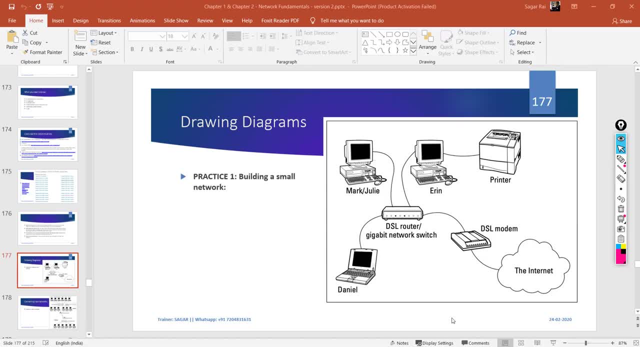 create and I am given this kind of page. now a blank page, okay. so what is my now? a blank page, okay. so what is my now? a blank page, okay. so what is my requirement? I'll first bring it up, so I requirement. I'll first bring it up, so I. 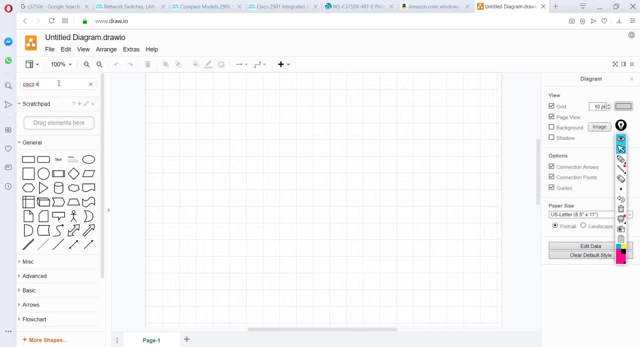 requirement. I'll first bring it up. so I need two switches. okay, so let me type need two switches. okay, so let me type need two switches. okay, so let me type Cisco switch here. so I am being getting Cisco switch here. so I am being getting Cisco switch here, so I am being getting something. so let me filter it out for a. 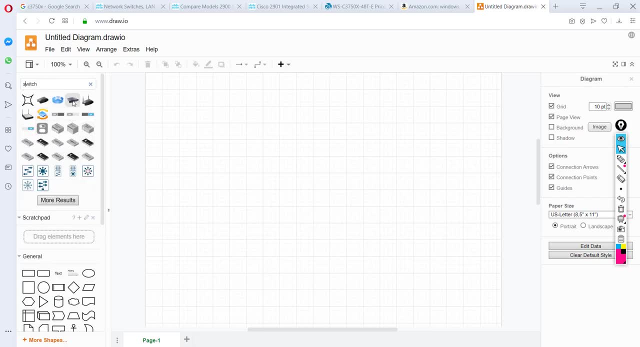 something, so let me filter it out for a something. so let me filter it out for a better result. okay, so I have few device. better result. okay, so I have few device. better result. okay, so I have few device, so let me bring it up. okay, so let's. 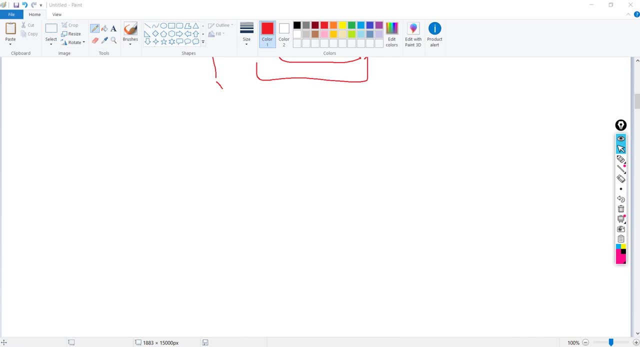 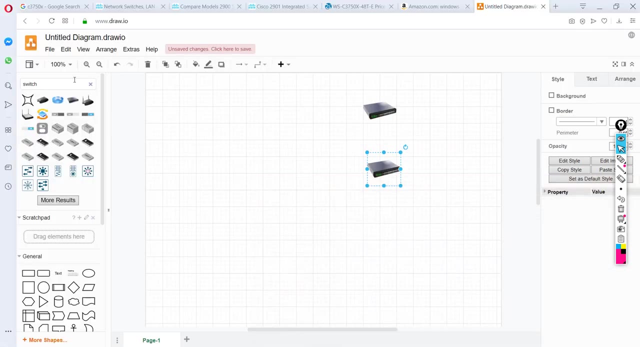 so let me bring it up, okay, so let's. so let me bring it up, okay. so let's consider: these are the 3750 models. okay, consider, these are the 3750 models. okay, consider, these are the 3750 models. okay, these are two Cisco 3750, 48 models. okay. 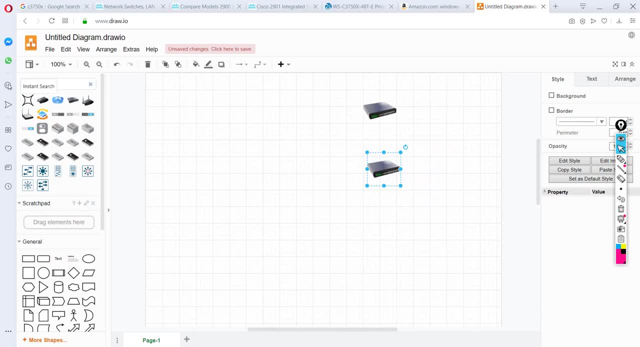 these are two Cisco 3750 48 models. okay, these are two Cisco 3750 48 models. okay, so we have that now. let's look for the. so we have that now. let's look for the. so we have that now. let's look for the router. okay, so I have a router. now the. 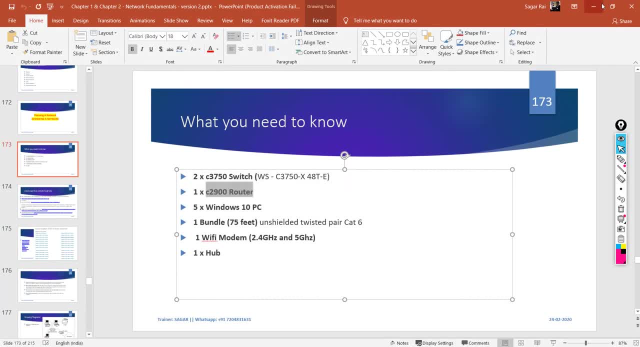 router. okay, so I have a router now the router. okay, so I have a router. now the router is going to act as 2900. okay, I IS. router is going to act as 2900. okay, I IS. router is going to act as 2900. okay, I IS. are integrated service router I need. 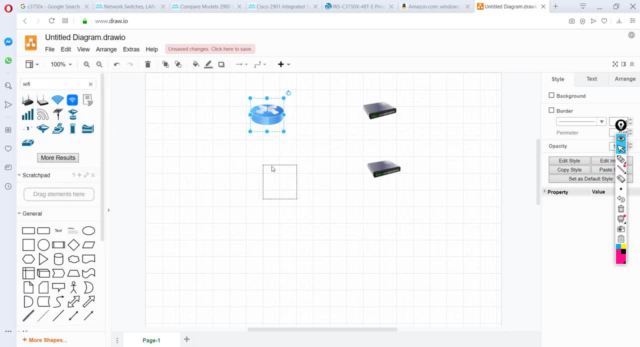 are integrated service router. I need are integrated service router. I need some Wi-Fi modem. so let me take one Wi-Fi. some Wi-Fi modem. so let me take one Wi-Fi, some Wi-Fi modem. so let me take one Wi-Fi modem also. I need computers, okay, so 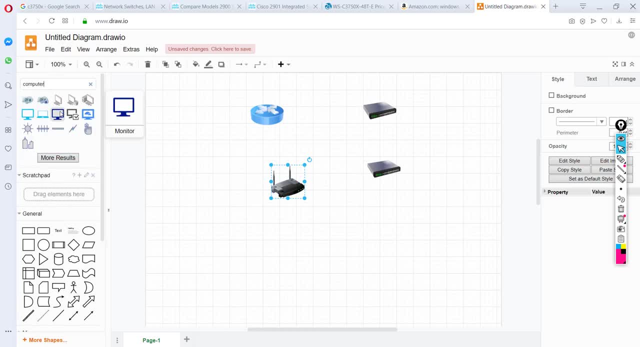 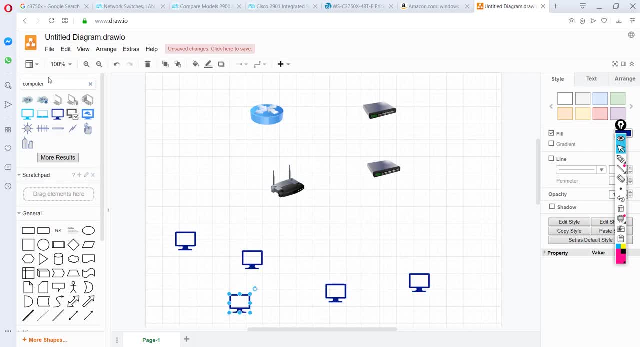 five computers- okay, that is the requirement. five computers- okay, that is the requirement that we have well, I need one that we have well, I need one that we have well, I need one hub. so let's say this is a hub okay, so I hub. so let's say this is a hub, okay, so I. 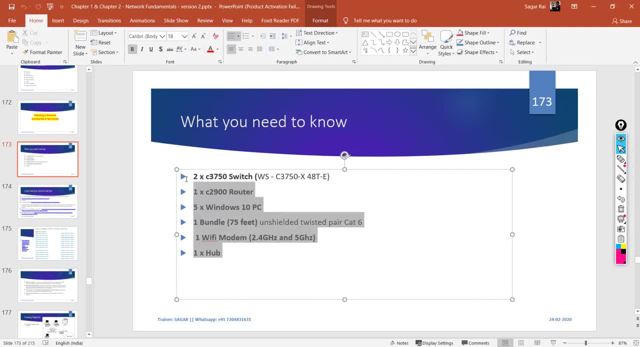 hub, so let's say this is a hub, okay. so I think we are all good the cables we can think we are all good the cables we can think we are all good the cables we can make use while designing. okay, so let let make use while designing. okay, so let let. 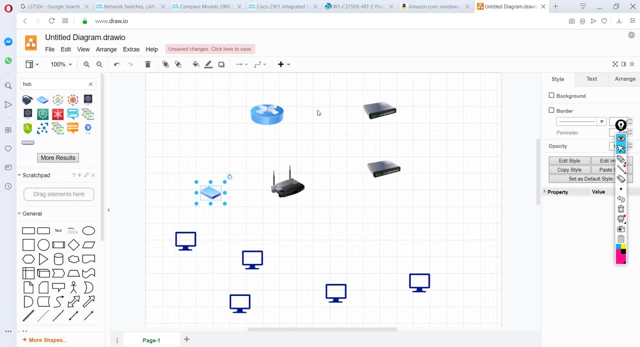 make use while designing. okay, so let let me orient now. let me do the orientation, me orient now. let me do the orientation, me orient now. let me do the orientation. so before that I'll also get something. so before that I'll also get something. so before that I'll also get something for internet, so that we 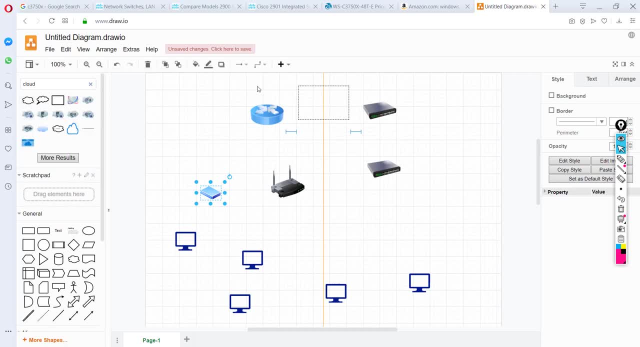 for internet, so that we for internet, so that we can understand what is happening. okay, so can understand what is happening, okay, so can understand what is happening. okay, so let's say: this is internet and these let's say this is internet, and these let's say this is internet and these are my users, computer users, okay, so 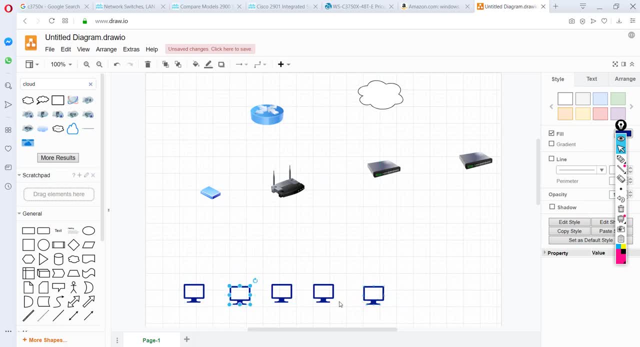 are my users, computer users- okay, so are my users, computer users- okay. so, basically, users will communicate to each. basically, users will communicate to each. basically, users will communicate to each other. okay, they can talk to each other other. okay, they can talk to each other other. okay, they can talk to each other and same time they also have to use. 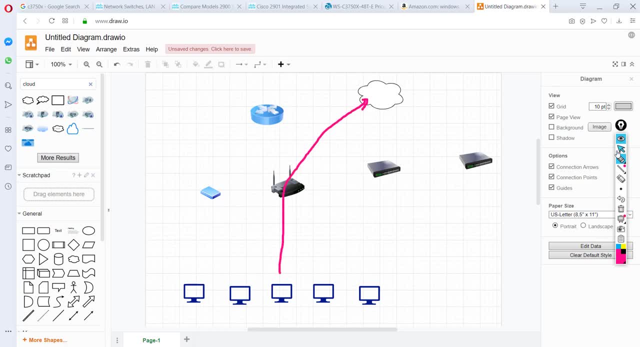 and same time they also have to use, and same time they also have to use internet for internet purpose. okay, so how internet for internet purpose? okay, so how internet for internet purpose? okay. so, how is the orientation going? is the orientation going? is the orientation going on? so we all know, computers are to be. 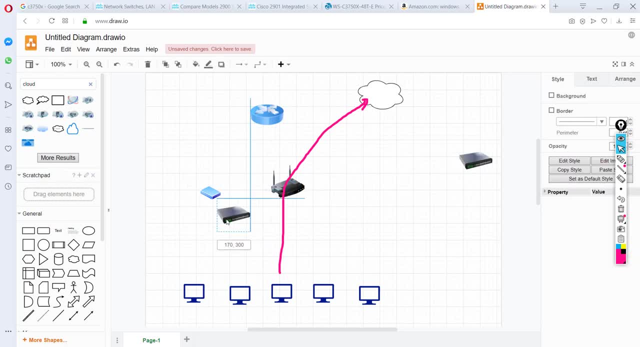 on. so we all know computers are to be on. so we all know computers are to be connected to a layer 2 switches. okay, so connected to a layer 2 switches. okay, so connected to a layer 2 switches. okay, so the two switches. I am going to keep over. 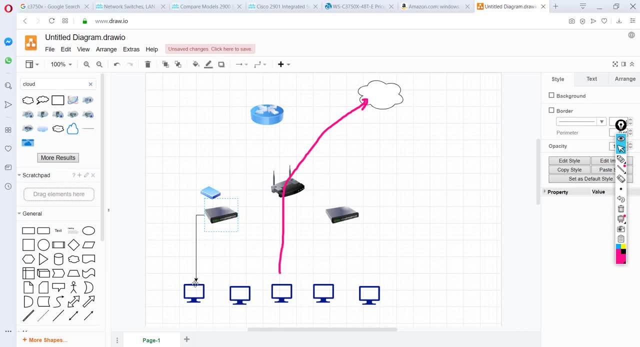 the two switches. I am going to keep over the two switches I am going to keep over here. okay, so let's give the connection here. okay, so let's give the connection here. okay, so, let's give the connection now. so let me do a cable connection. so 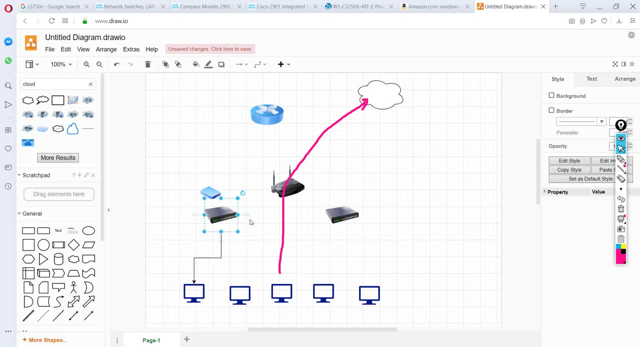 now. so let me do a cable connection. so now, so let me do a cable connection. so this is going to be RJ 45 connection. this is going to be RJ 45 connection. this is going to be RJ 45 connection. okay, so this is a cat6 cable which I am. 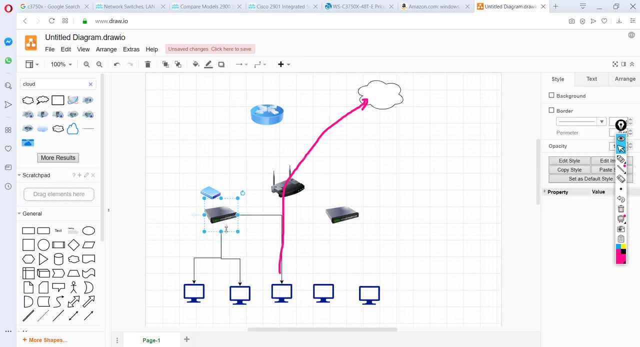 okay, so this is a cat6 cable which I am. okay, so this is a cat6 cable which I am laying across. let me make use of this to laying across. let me make use of this to laying across. let me make use of this to connect another two computers. okay, so my. 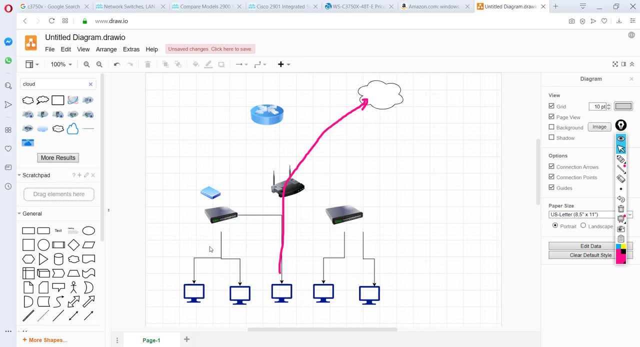 connect another two computers. okay, so my connect another two computers. okay, so my computers and the Cisco switches are computers and the Cisco switches are computers and the Cisco switches are going connected. okay, rest are not going connected. okay, rest are not going connected. okay, rest are not connected. yet I have not connected. 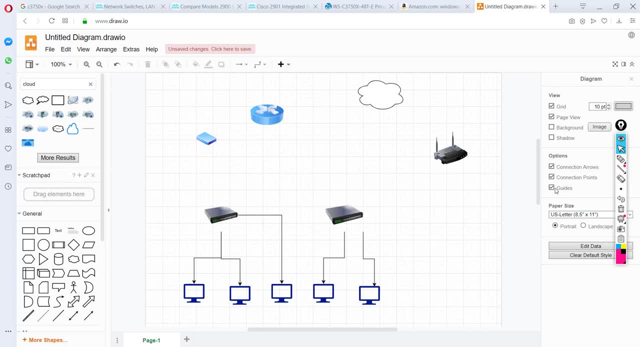 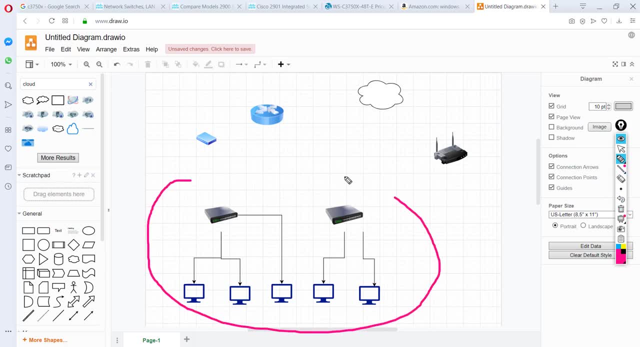 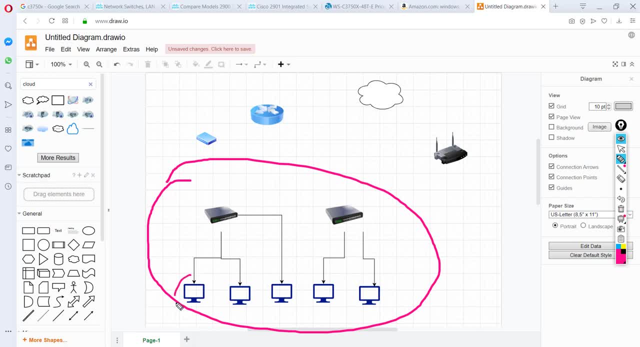 area network. okay, so basically, user from area network. okay. so basically, user from this machine can communicate with user. this machine can communicate with user. this machine can communicate with user of this machine. okay, because they are of this machine. okay, because they are of this machine, okay, because they are only connected to a switch. and if you 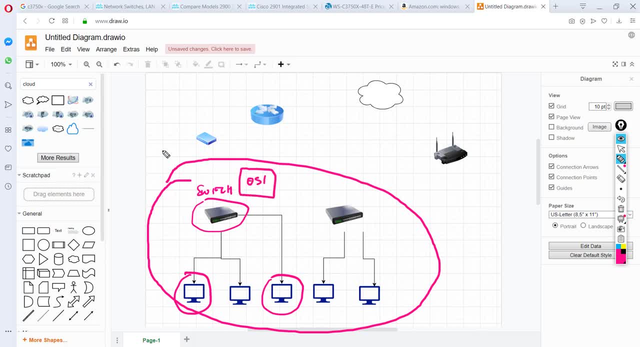 only connected to a switch and if you only connected to a switch and if you remember the OSI layer we talked about, remember the OSI layer we talked about, remember the OSI layer? we talked about data link layer. okay, if, if, if I have data link layer. okay, if, if, if I have. 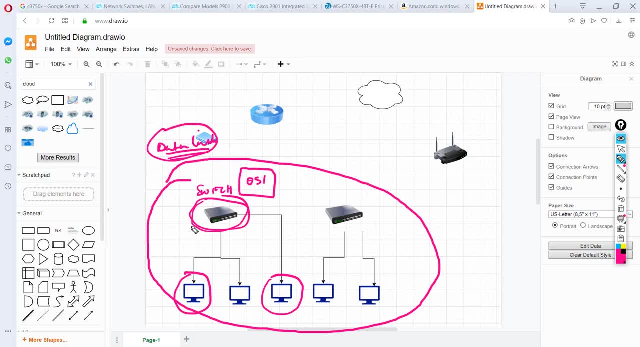 data link layer. okay, if, if, if I have a layer 2 switch which is a part of data, a layer 2 switch which is a part of data, a layer 2 switch which is a part of data link layer, and if I have a computers, then 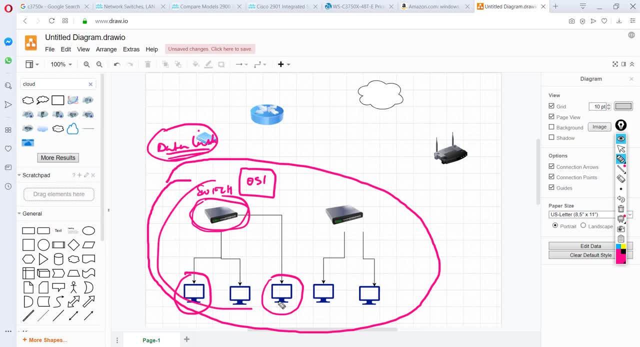 link layer, and if I have a computers, then link layer, and if I have a computers, then they can talk to each other because they, they can talk to each other, because they, they can talk to each other because they are in one network. okay, okay, fine, so now. 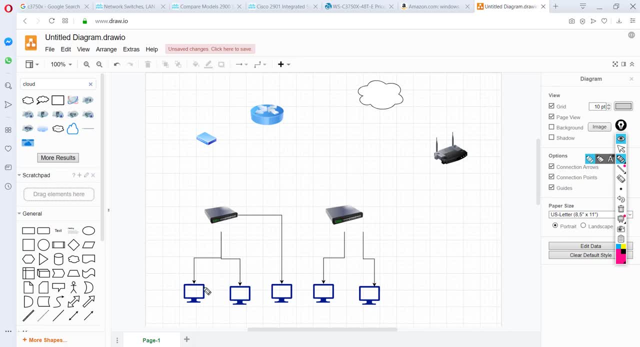 are in one network. okay, okay, fine, so now are in one network. okay, okay, fine. so now the switches has to be connected to a. the switches has to be connected to a. the switches has to be connected to a router, because the requirement is now to router, because the requirement is now to: 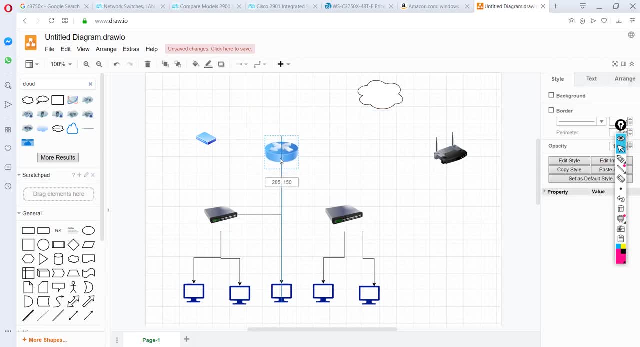 router because the requirement is now to reach internet. okay, so I am bringing my reach internet. okay, so I am bringing my reach internet. okay, so I am bringing my router here. I'm laying a cable from this router here. I'm laying a cable from this router here. I'm laying a cable from this router to this router. okay, and from the. 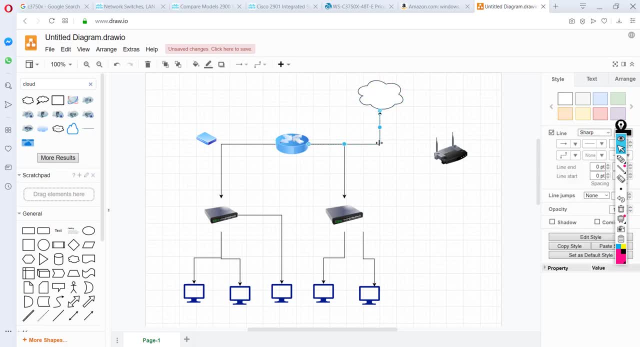 router to this router- okay. and from the router to this router- okay. and from the router to cloud- okay, fine. so now my router to cloud- okay fine. so now my router to cloud- okay, fine. so now my requirement can serve all all the in. requirement can serve all all the in. 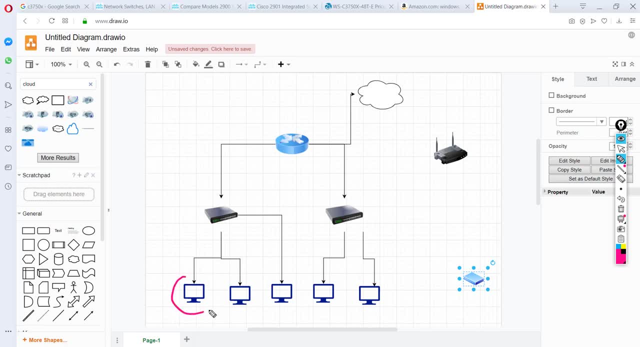 requirement can serve all all the in internet connect connection also, if this internet connect connection also, if this internet connect connection also, if this is a user is a user is a user if he wants googlecom, if he wants to, if he wants googlecom if he wants to. 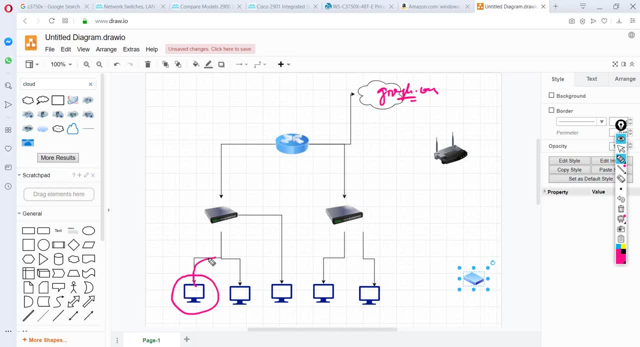 if he wants googlecom, if he wants to browse googlecom so he can type browse googlecom. so he can type browse googlecom. so he can type wwwgooglecom. his packet will go to wwwgooglecom. his packet will go to wwwgooglecom. his packet will go to switch. switch will take it to router and 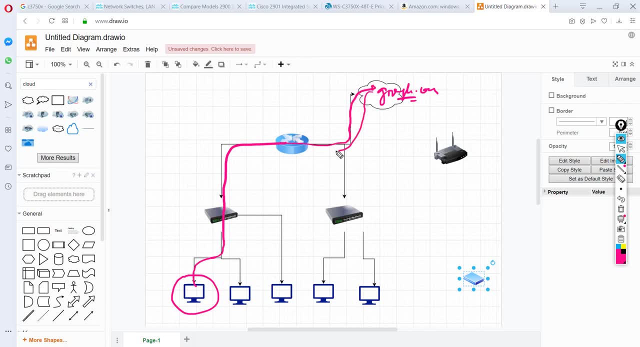 switch switch will take it to router and switch switch will take it to router and router will take to googlecom and the router will take to googlecom and the router will take to googlecom and the written traffic will also come in this. written traffic will also come in this. 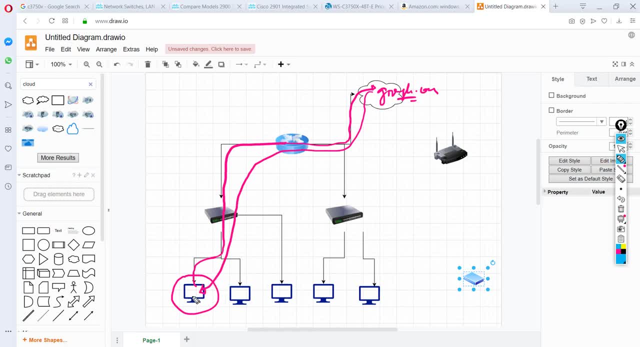 written traffic will also come in this direction. okay, same same time. if he wants direction, okay, same same time. if he wants direction, okay, same same time. if he wants to send some file to this user pc, to send some file to this user pc, to send some file to this user pc number uh three, okay, so in this case his 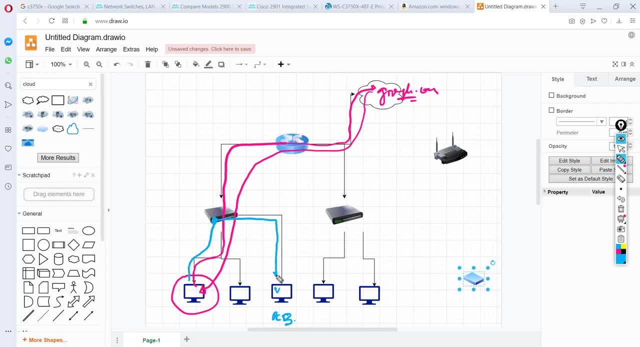 number uh three. okay, so in this case his number uh three. okay, so in this case his traffic will go to switch and switch. traffic will go to switch and switch. traffic will go to switch and switch will directly send to this. okay, it, it will directly send to this. okay, it it? 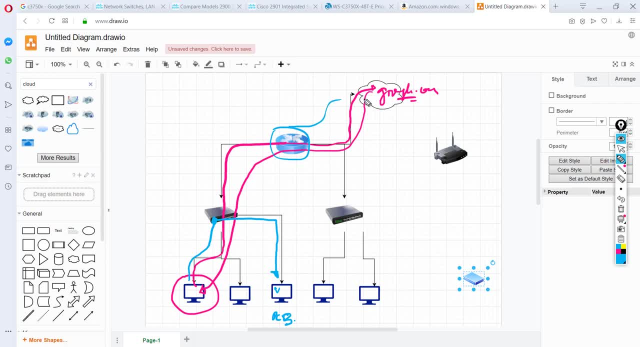 will directly send to this. okay it, it doesn't have to go to uh, doesn't have to go to uh, doesn't have to go to uh internet. or it doesn't have to go to internet, or it doesn't have to go to internet or it doesn't have to go to cloud because switch knows. how are these? 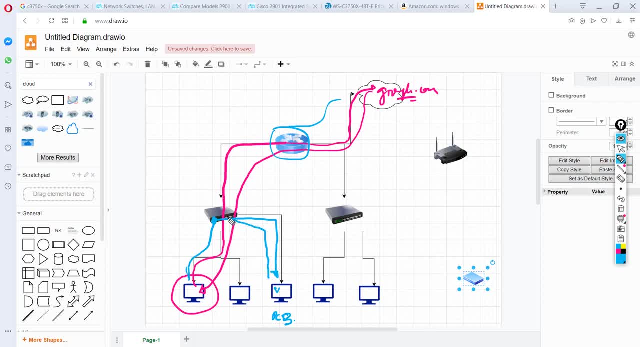 cloud, because switch knows how are these cloud. because switch knows how are these three computers connected and same way. three computers connected and same way. His return traffic will go to switch and from switch it will come back to this. Okay, So there are two things we can achieve here. 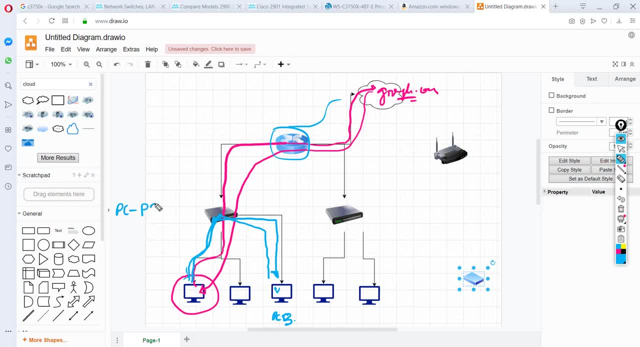 One is a PC to PC connection and one is PC to internet connection. If you want to browse Google, if you just want to play counter strike, imagine you have counter strike installed here and you have counter strike installed here. Okay, So if you're playing in a LAN connection, so your packet is going to switch and switch. 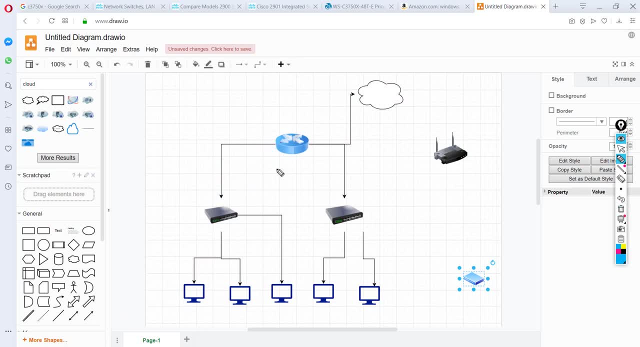 is sending back to this. You don't need internet, Okay, fine. So now let's say we also wants to communicate from this to this? Okay, So what I can do is I can connect one cable between these, Okay, So that my traffic can directly go in this direction. 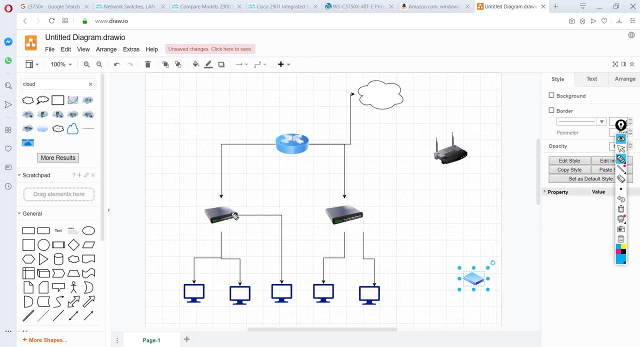 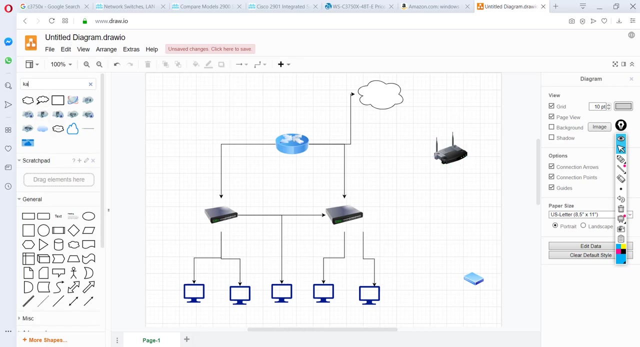 Okay, So let me connect one cable here. Fine, So I can have now different PC to different PC connections. Now let's say I have one laptop user who don't want to be connected to cables. Okay, I have a laptop user here. 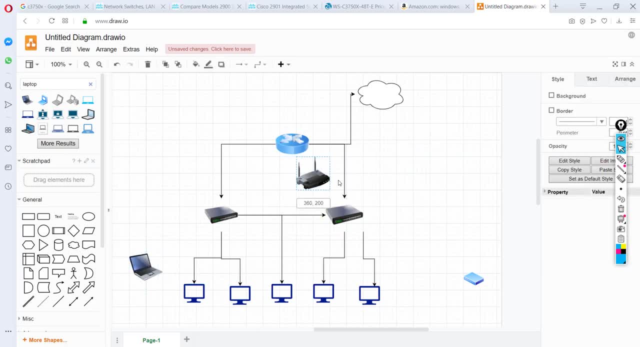 Let's say, laptop user here. So what I'm going to do is I'm going to introduce a modem, a wifi modem, And wifi modem Is again connected on a switch. Okay, So always remember all the end devices like wifi modem servers, okay, computers, PC. 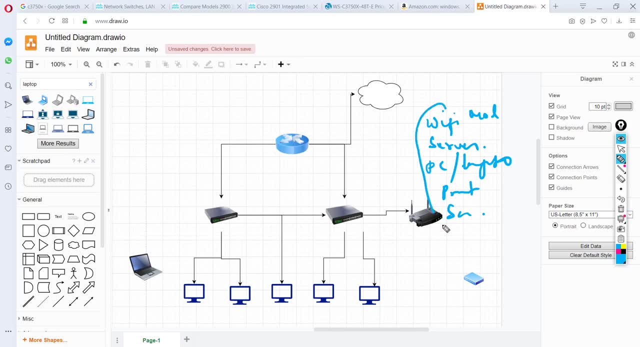 laptop printer scanner. These are all called as end devices and they are always connected to a switch. Okay, So that is why I connected to this switch. Now, This wifi modem can support 10 meter of radius. That means the wifi modem can support up to 10 meters. 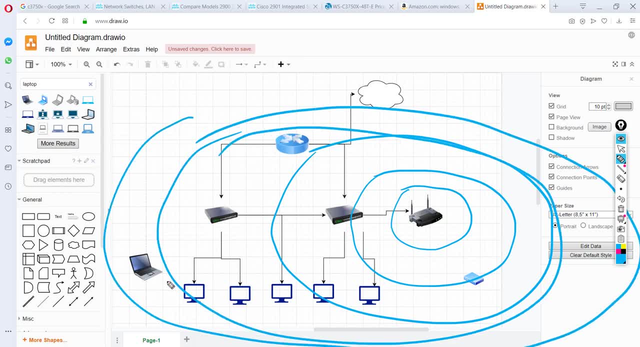 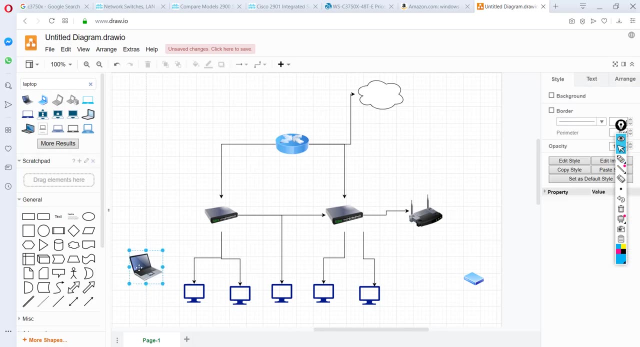 So if this user is within 10 meters- okay, the distance is 10 meters- then this user can get connected to this wifi modem. Otherwise, we have to ask this user to sit somewhere closer to this. So let's say I will say I will just ask him to sit. 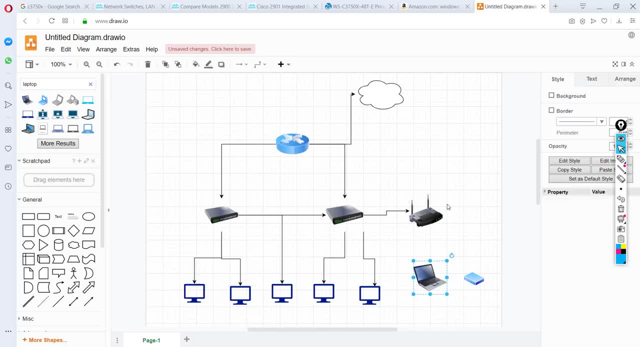 Okay, Okay, I will just ask him to sit closer to this modem so that he can get access, Okay. So where is this modem getting the input? It is getting the input from the switch, Okay, And between them they have their wifi signal. 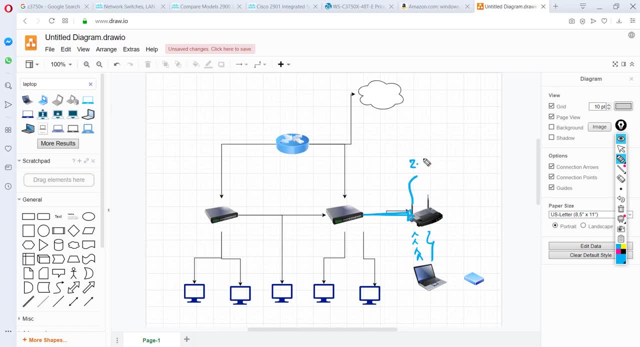 Okay, So there are two different type of wifi signal. One is 2.4 gigahertz and second one is 5 gigahertz. Okay, So it depends which one you're going to configure. Okay, So basically, if a user is typing googlecom, okay. 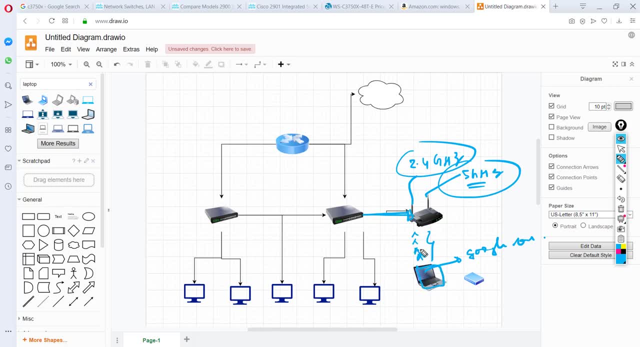 So what is happening? His laptop is sending wifi signal, wireless signal to the modem. Modem is connected with the help of cables, Then this is going to the router. router is then sending it to googlecom. Okay, So this is how the network connection happens. 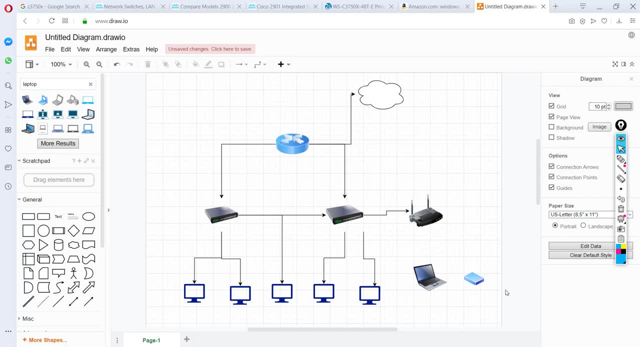 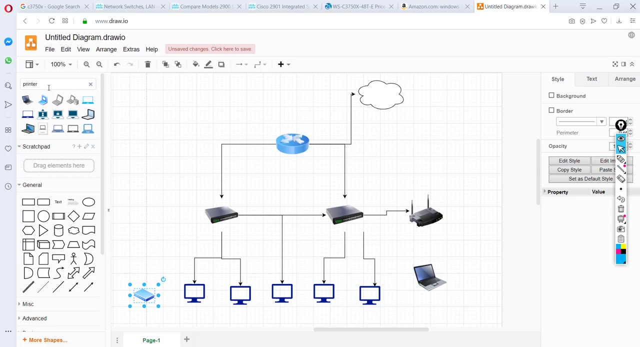 Fine. Okay, Now we have a hub Which is just kept unused. Let's say I have one user here. Okay, User has some scanner with him or some printers on his desk, So I'm going to get some printer on his desk. 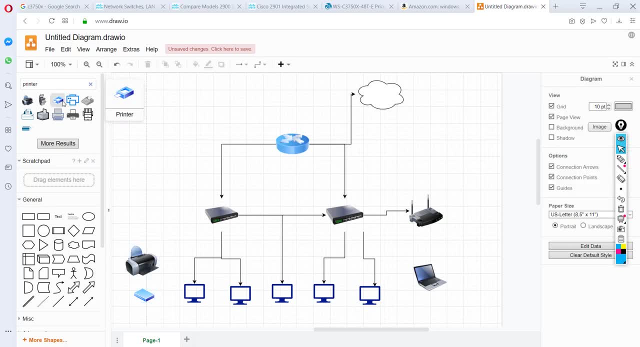 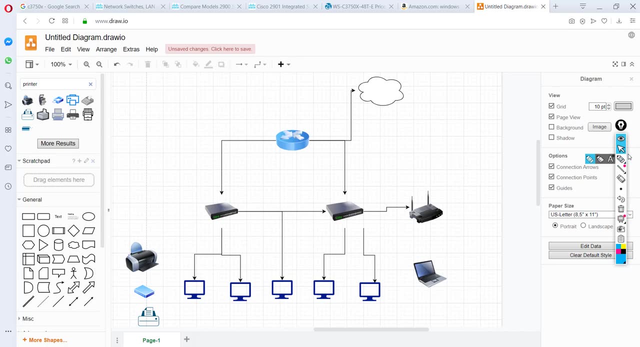 Okay, And let's say he has some fax machine- Okay, But he has just one printer, Just one cable, One cable, Right, And I need all these to be connected. So what I'm going to do is I'll take out this cable from here. 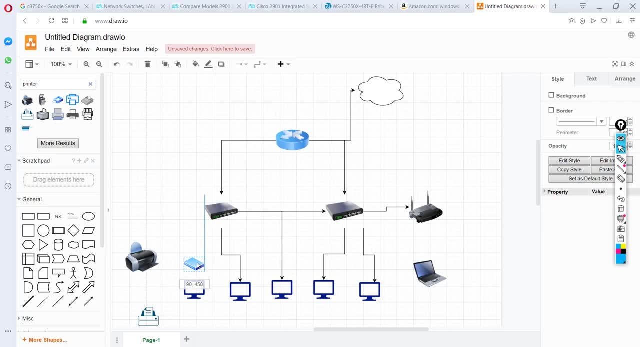 Let's delete this. bring the modem here, the hub here, Okay. Now what I'm going to do is my hub will connect to switch, Okay, And then hub is going to get connected to rest of things. Let's say, Uh, from here to here, and let me bring here. 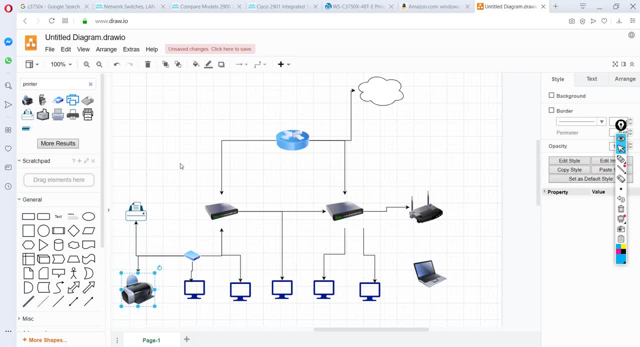 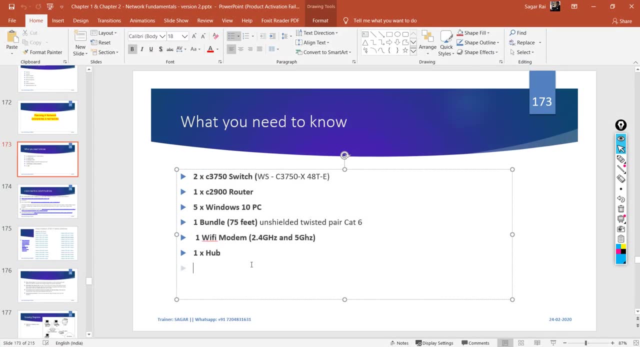 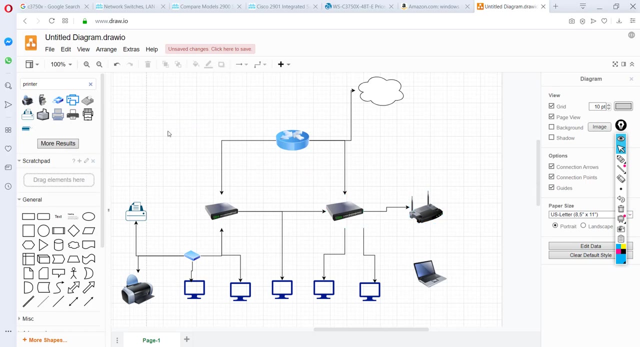 Okay, Something like this: So we are utilizing all the network components for one thing. Okay, Whatever my customer has given me the requirement, I'm going to make use of all the network components. I have given the design Okay To the customer. 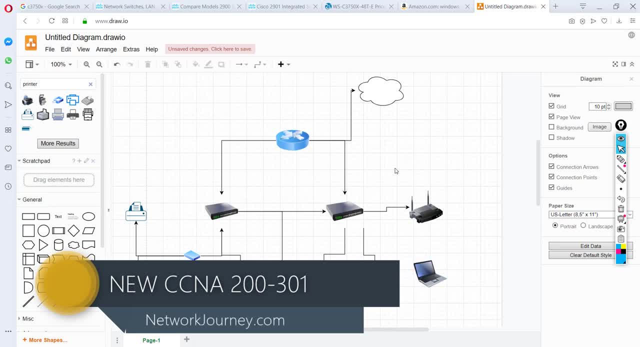 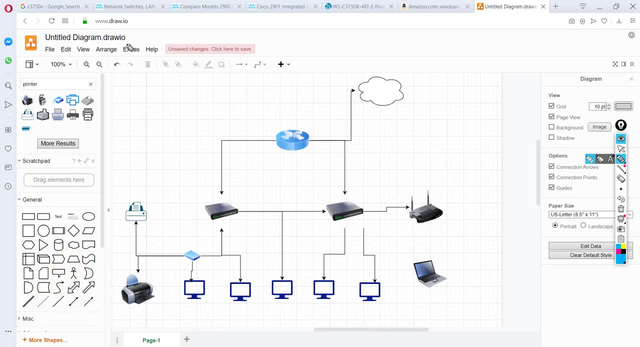 Now the customer will check this. He is doing, He is okay with this. He is saying: it is a perfect design without wastage of anything. Now the design will be sent to the vendors. Okay, Uh, vendors, who is in that office? might be, might be, you're sitting in Bangalore. 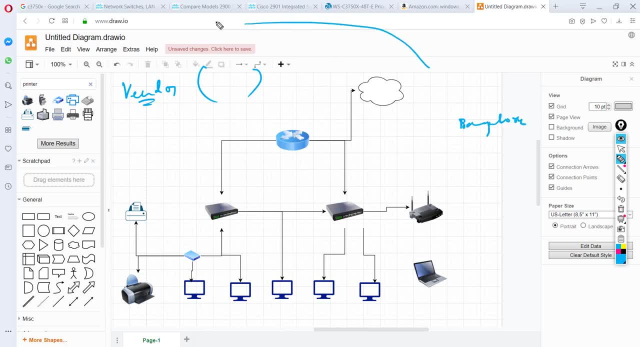 Okay, The customer requirement is coming from us. Okay, And this actually has to be deployed in Australia Right now. You cannot go Okay To Australia and deploy it. Okay, You are, you are giving the remote support, So who is going to deploy? deploy in Australia. 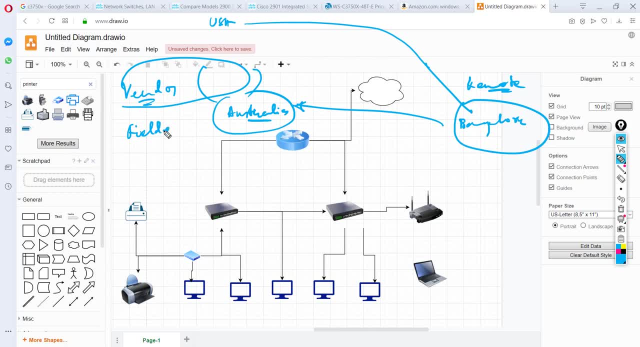 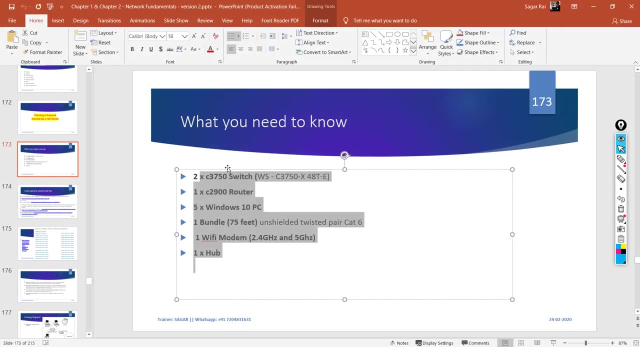 It is the vendors. Okay, We call them as field engineers. Okay, So we are going to send the documents, all the documents. we are going to give him the design, We are going to give him, uh, these network components, Okay, 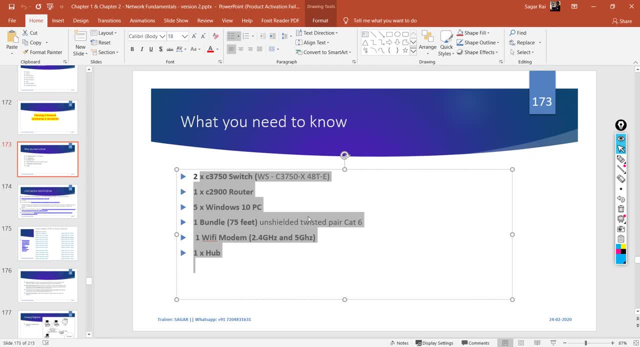 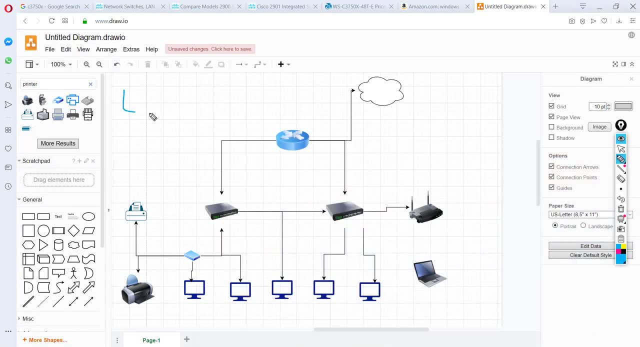 We can do the purchase on behalf of the field engineer Directly. We can place the order on Cisco website and Cisco website. They will uh the the Cisco. Cisco team will ship the materials to the site. Okay, Australia site. 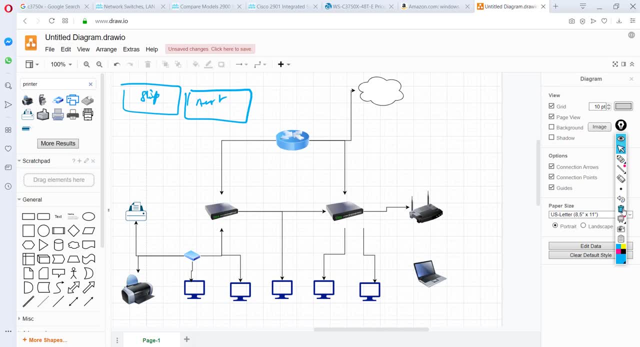 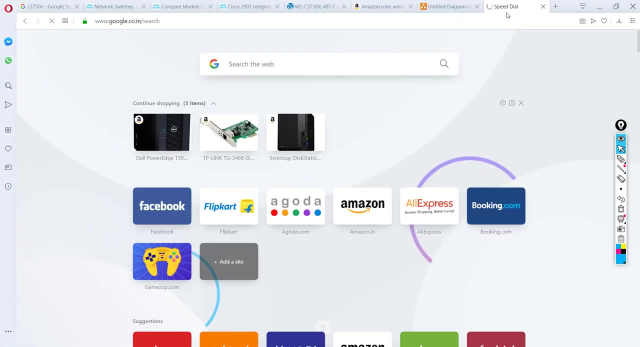 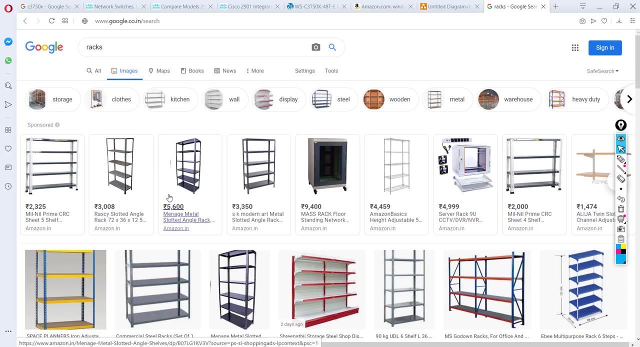 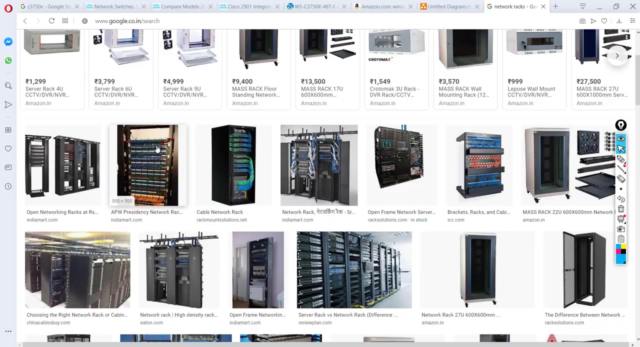 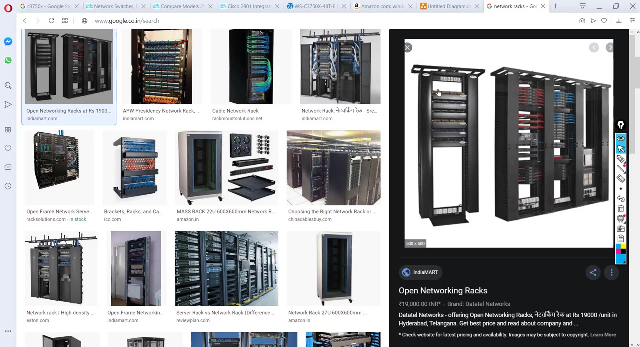 Now the vendor will go and buy the racks, Okay, So basically these are called racks, Okay, Okay, Okay. So let me look for, uh, the network racks, So something like this: the vendor will purchase it, He will mount it on the uh floor and he all the devices. 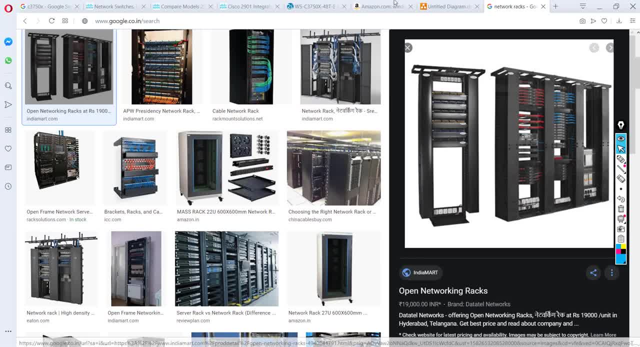 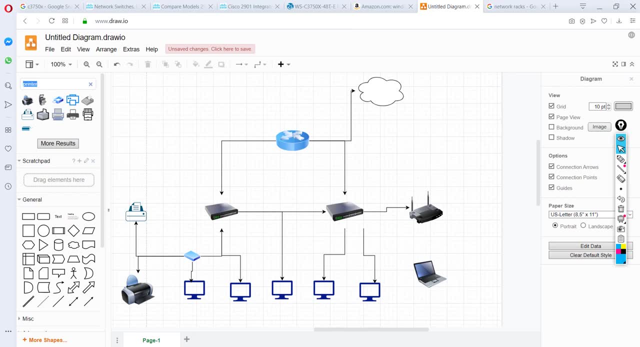 So, basically, the design which you are seeing over here. Okay, They might look like in vertical and horizontal things, Right, But in real they are going to place one below one. Okay, So let me show you over here. let's say, I'm going to take one rack and show you the things. 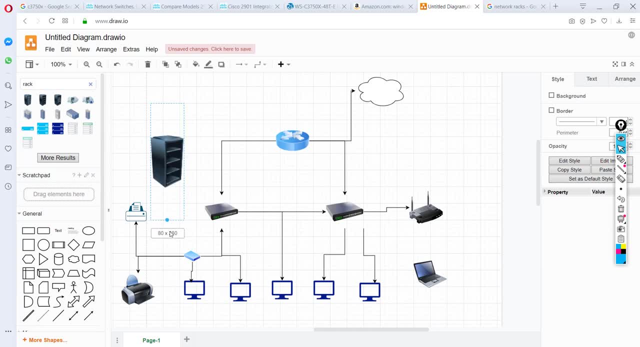 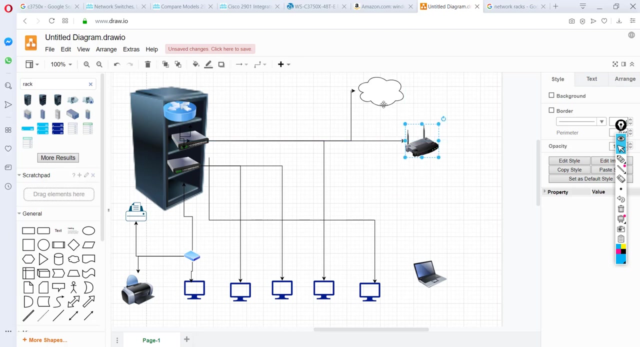 Okay, So this is my rack, Fine, So let me just try to find. So this is a rack Now. this will be placed here. Okay, This is placed here. The switches are placed here, Okay. Okay, Modem will go to somewhere on the ceilings. 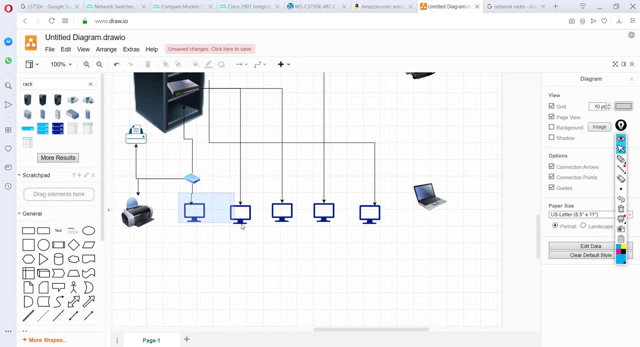 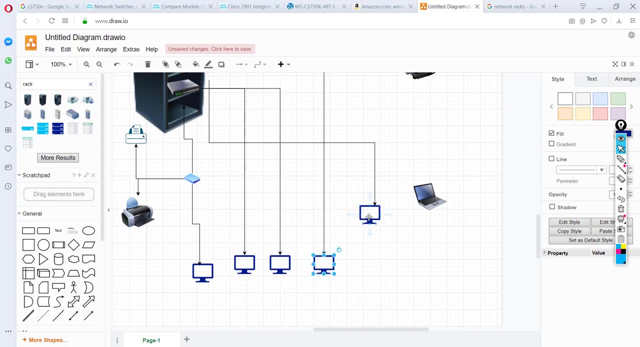 Cloud is somewhere on the top, Okay, And the computers will be placed on the real office, like where you sit, actually on the floor. Okay, Let's let me bring it down, And this is also on a floor printer. as I told you, it is on his desk. 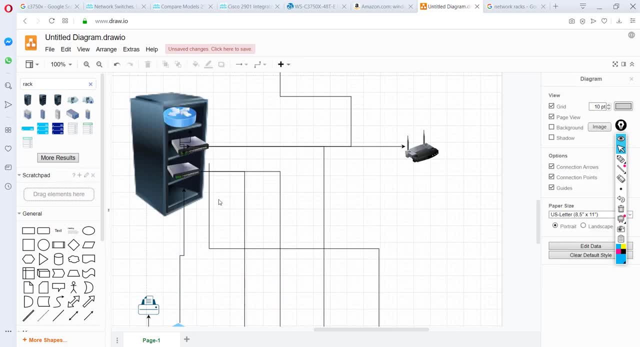 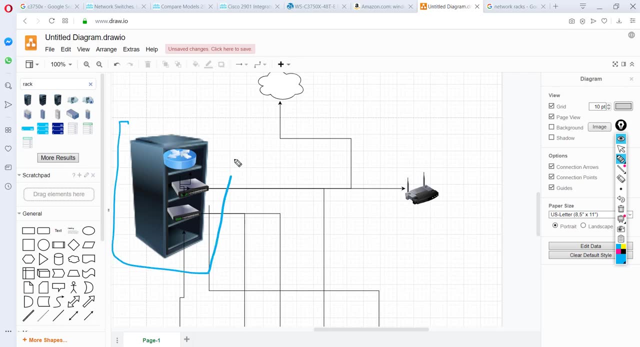 So let me keep it here and modern is again on his desk. Okay, So this collectively is called as it room. So basically, you will see the it room will be placed. It will be placed somewhere in a, in an isolated place, like it room. 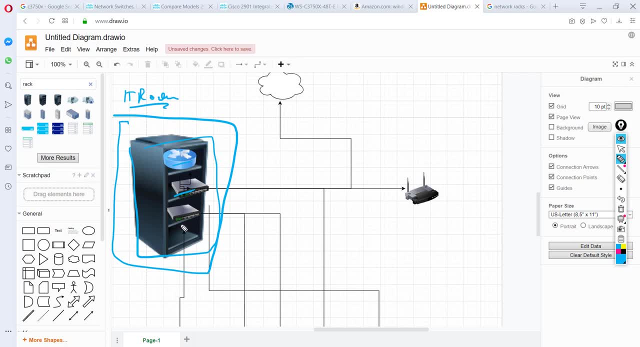 And this is a rack where you are going to keep the devices, one below one. You're going to cable them as I showed you. Okay, Like if you go back? so I just done the cables right. So, similarly, you are going to do the cabling and then you have the perfect office setup. 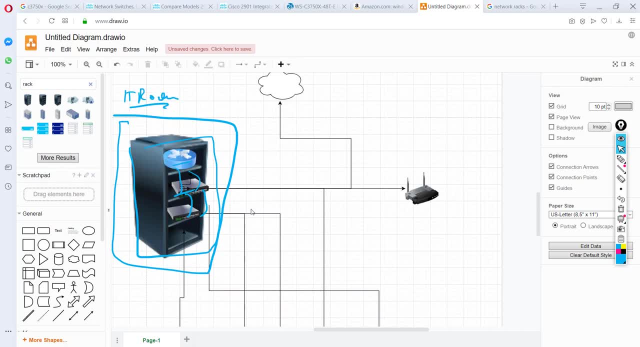 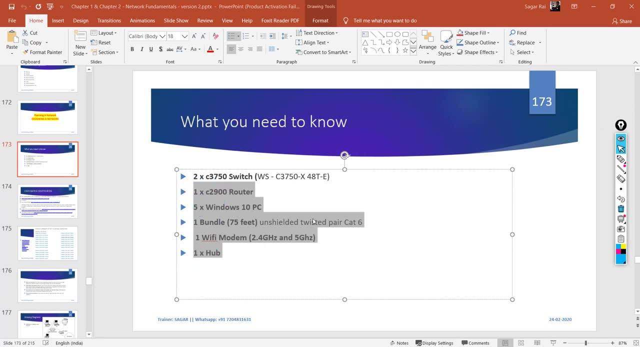 created up, Okay, Okay, So that's been done And that is how, uh, you guys are gonna make a wise decision: by by all the components that he has given you. you cannot buy any new components on your own, Okay. 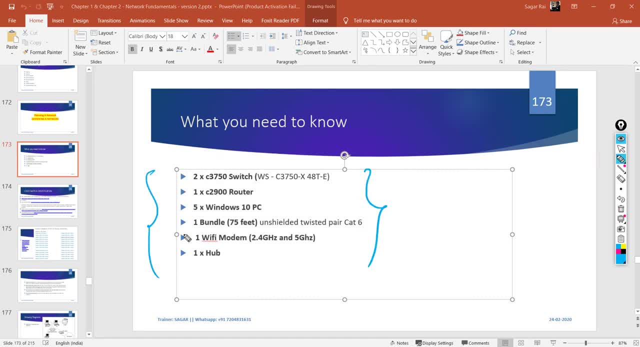 So basically, uh, whatever he has told you, you have to invest on that. at the same time, you have to make sure that design can be upgrade, upgradable in future. Your design should not be, uh, old enough design Okay. 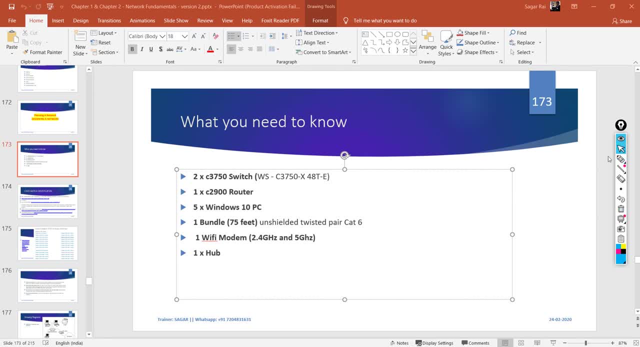 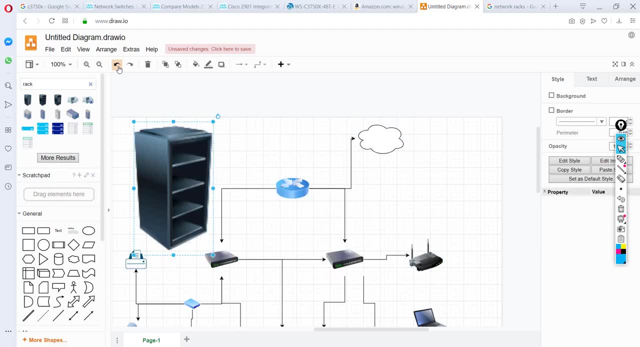 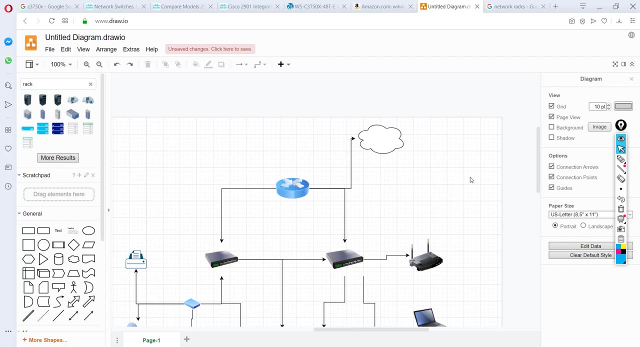 Fine, So any doubt, guys. anything which, uh, is not clear: What is the difference between this 2.4 GHz and 5 GHz? Okay, So, regards to that, we will come later. Okay, So that is a wireless technology which we have to cover in theoretical. Okay For a just in short form, 2.5 GHz has a longer radius, Whereas 5 GHz has a longer radius, Okay, So both have their plus and minus, so which we will check out in in in the wireless. 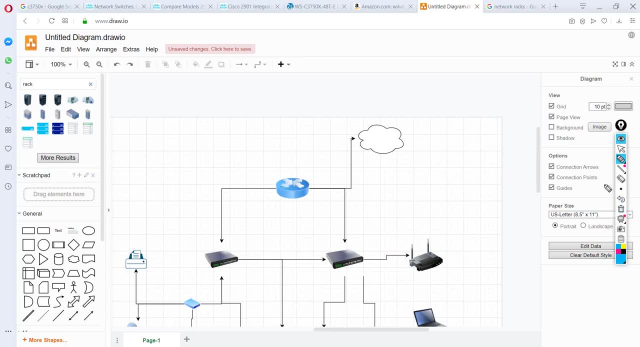 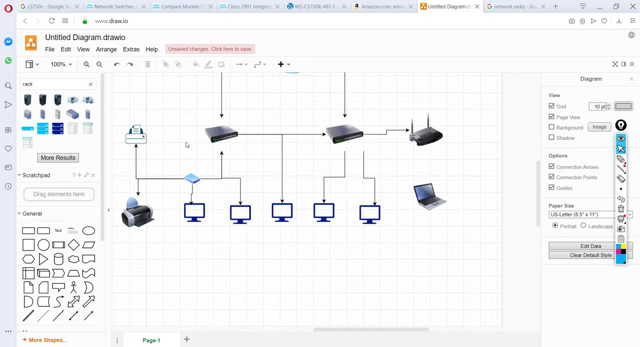 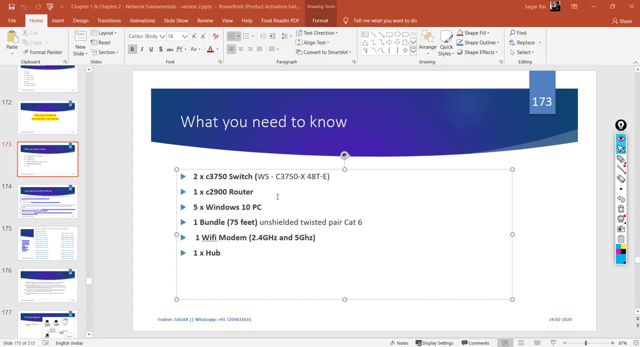 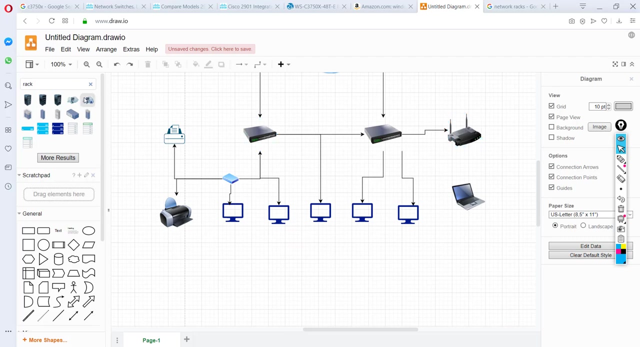 technology. Okay, Okay. Then if you have five computers, that is just for an example- I have showed you. Okay, I told you that this is a requirement coming from customer, so there is chances might be. customer has a plan of increasing the users, right, so he is not trying to invest eight ports if he is investing on eight. 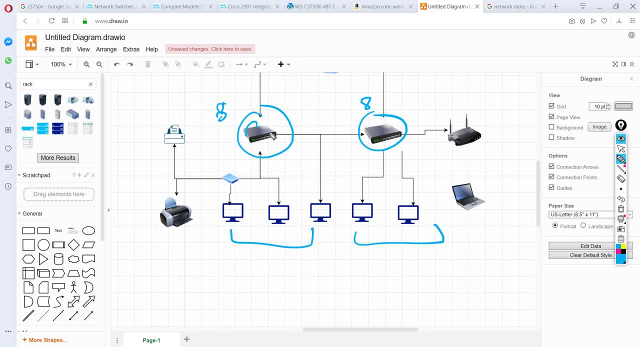 ports might be. next, when he have lot of users, he has to discard this and place new device. so that is what i told you: when you are designing network, always think of future. also right might be. his requirement now is to start with five users and later on increase to like 50 or 100. 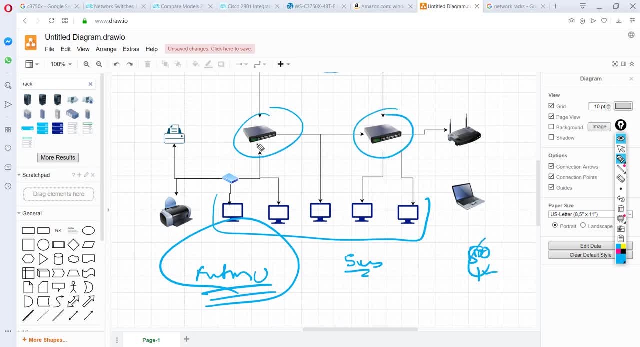 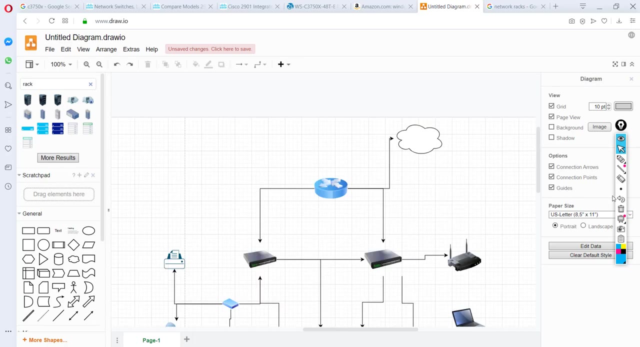 users. so that is what it is going to serve the purpose. fine, why we need to connect router to one switch. again one more cable from router to one switch. you need to connect your router to one switch and router to switch to switch. one cable, that's enough, right see? 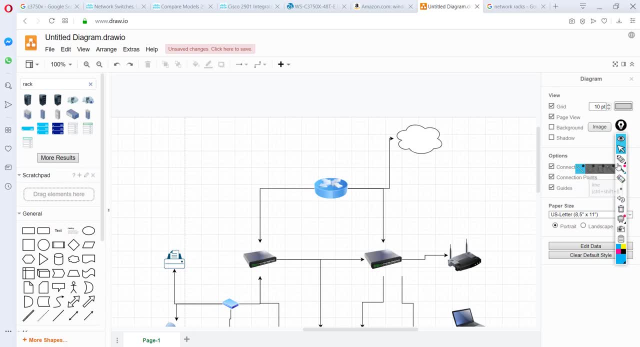 we can connect the way from two switch to one, but since in this it is really little difficult, okay. so basically what i can do is, let's say i have one router here and i have two switch here, okay, switch number one and switch number two. and if they're interrelated, 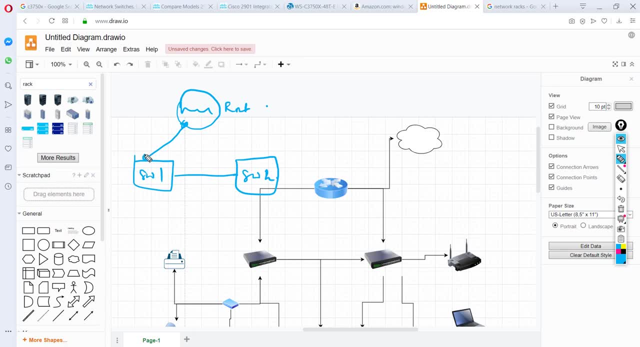 so i connect one interface to one interface here and i connect one interface to one interface so i connect and i log two devices under one interface. i can include domain and i can force one interface to one interface and sorry, because two devices together. so i can use one interface if i want to change messages after the twogang generation and via the dm. 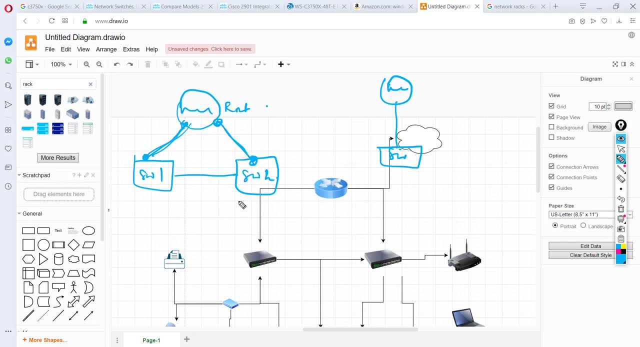 i will have to perform the same task. i will start off the other laptop again. after driver and Hydra. one more upward crossing like this, step by step. okay, that's free, cool, then you know the cable from the router to switch right, so one already switched to switch is connected. 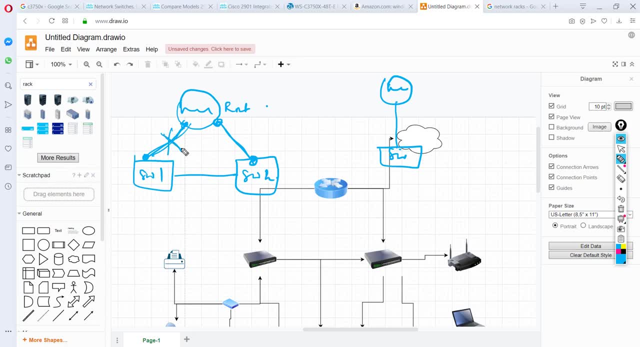 already switched to, switch is connected. so what if? what if this is going down? what if this is going down? then you will reach you, you will have an outage right? yeah, yeah, yeah, okay. so see this, this design is very, very basic, okay. just to serve five employees. i have not even. 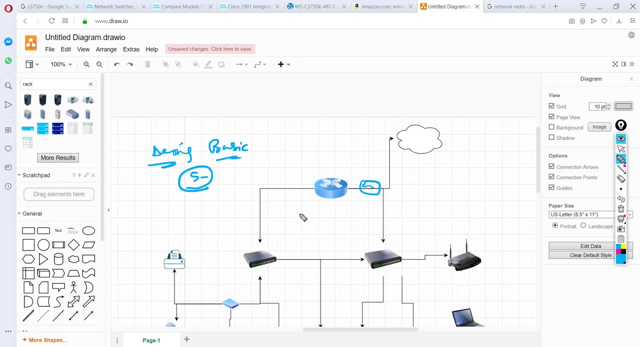 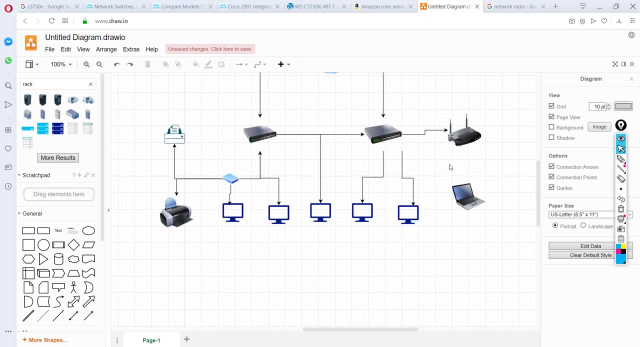 configured any redundancy uh routers. okay, this is very basic, just so that we don't end up with any uh outage and at the same time we have some future rooms for uh development. okay, say, one is like how uh? we had a question today like why 48 port for just a five user? okay, 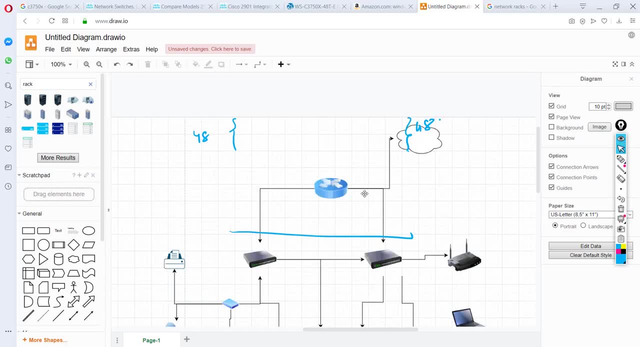 i could have taken that example over here on a router as well. i could have taken an example of 48 port. okay, but i only took it on switches, because on a switch we have end devices connected. so in future there can be many printers coming in, many wi-fi modem coming in, many users getting. 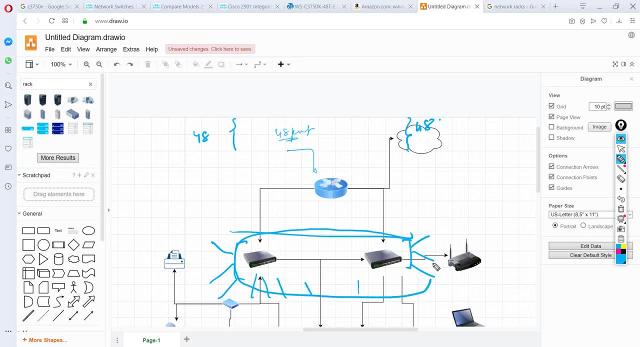 connected in. okay, so basically all of them are going to get connected to a switch at the same time. all of them like hundred users. for them, one router is more than enough just for uh internet, okay. so that is why i said we will go with the basic router design, which is good enough to. 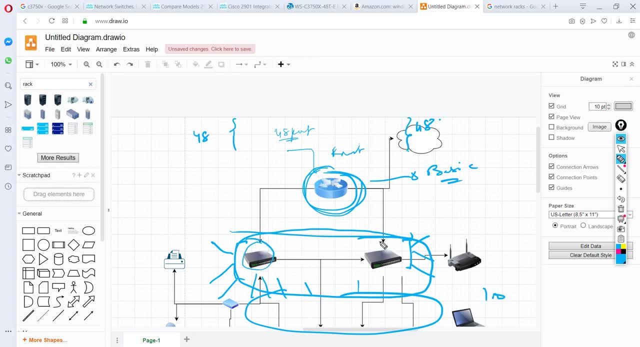 connect to internet. rest we are focusing, or rest we are going- with a good 48 port so that we have uh future rooms to develop. okay, same time, like as you were asking, like why two cables? so that is because if one is down we have one still working okay as a redundant uh path. 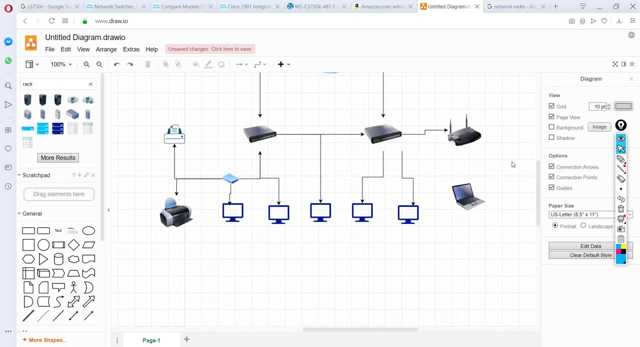 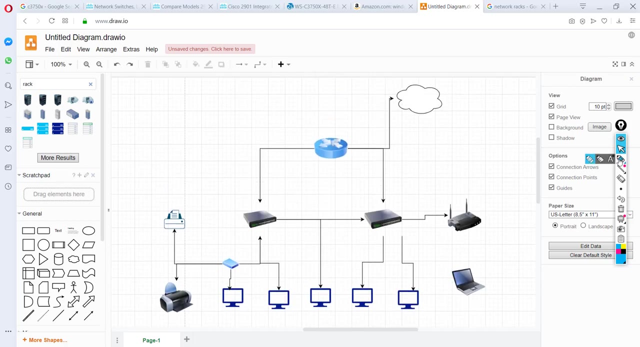 so guys who joined uh late might be after like few days or might be. who is joining for the first time, uh to the networking class. so i just want to make sure that you know that this is the orientation. okay, this is the orientation of the device, because we had a question put up like how the switches. 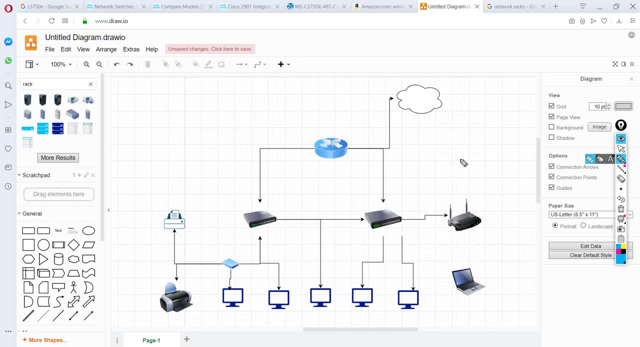 router, computers, modems, are really placed one, one after one, like how, how are they going to be placed? so this is how they are going to place. okay, and we have already discussed about three tire architecture, two tire architecture. okay, so this act as our core. okay, this is going to act as the 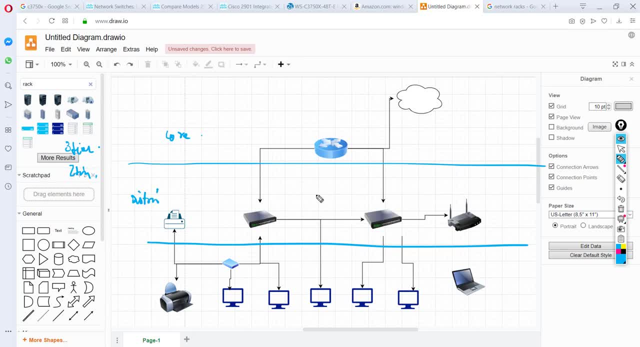 distribution. okay, so in this case, this is distribution and this is access. we don't have any other switches. okay, so this is going to be distribution and access and this is called a score. so core is something where we see the routing things happening. okay, distribution and access is nothing, but where you are distributing. 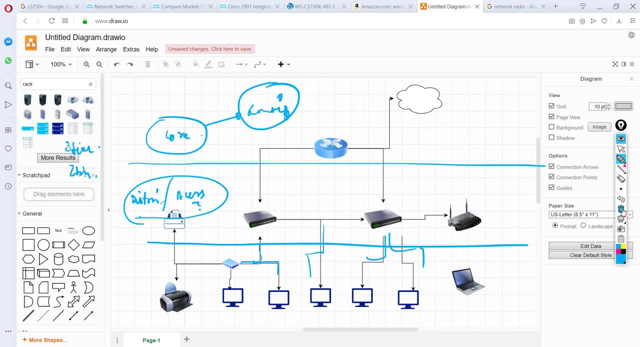 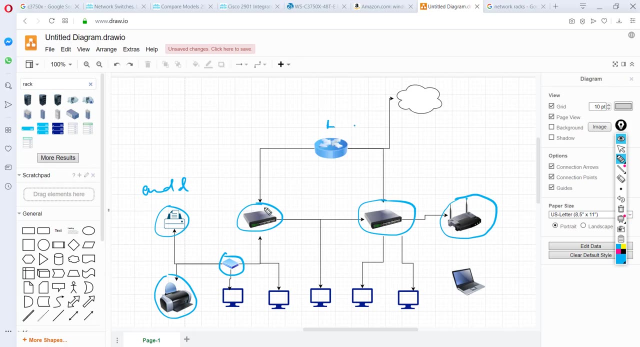 to different uh users or computers. okay, and if you see the orientation of wi-fi modem hub the other devices which are end devices. they are always connected to a switches. okay, they are not connected to a routers. if you connect to router, you can connect to router, but thing is then. 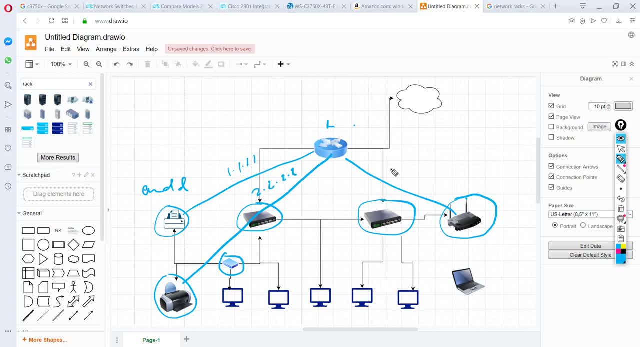 you have to serve now IP addresses, which is name and then address. okay, because there is a lot of 走 around the world about one network, okay, which is called IP file interface. okay, and same with local network, okay, so this is a local IP and one network. this is to one network, this Is one network. 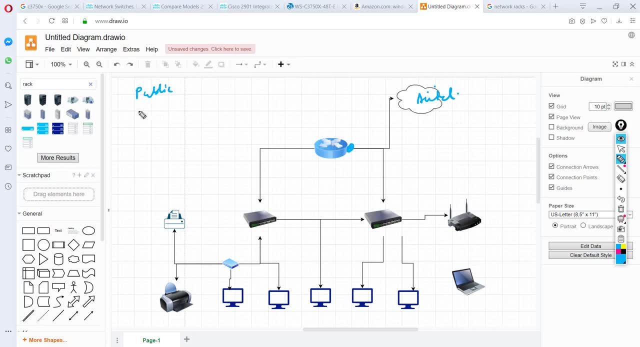 this is one network. this is one network. you will end up with so many ip wastage, okay, private, Okay. So public is seen very close to internet and private is seen very close to land. That is, these are going to be private IPs, okay. 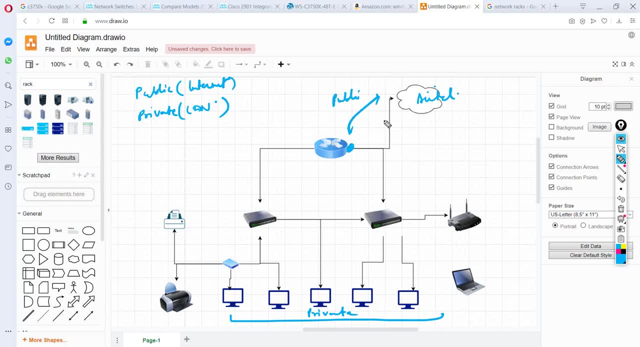 And this is going to be public IP, fine. So Airtel has given me public IP, Airtel has given something, this okay, And on their side they are going to configure this. okay, And now we have to make the connections okay. 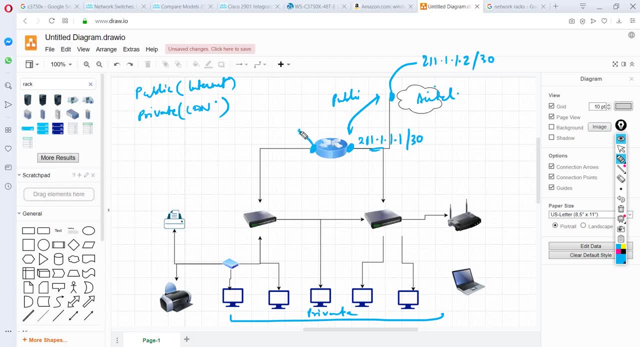 So what I'm going to do is I'm going to take one IP here, okay, Like any private IP. let's say 192.168.1.0, slash 24.. Now what happens? I'm going to create some see router understand IP address. 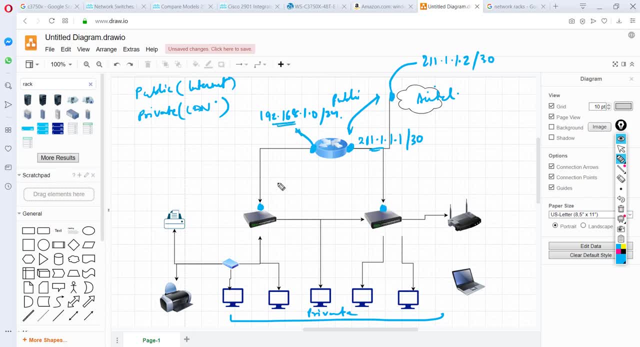 Okay. Whereas switch doesn't understand IP address, switch understand MAC, okay. So how is MAC or the IP address going to communicate? We are going to create some VLANs, okay. So we are going to create some VLANs over here. similar way, some VLANs over here, okay. 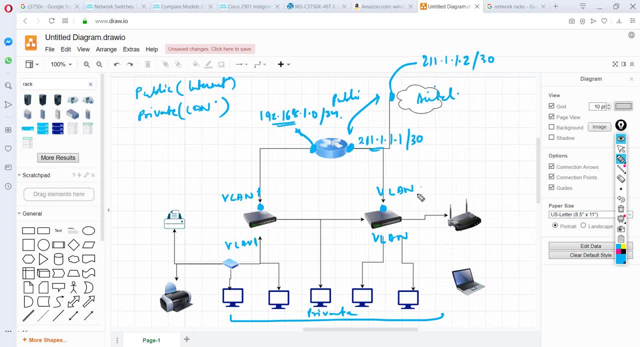 Now let's say, this is VLAN number one, This is also VLAN number one, This is VLAN number one, This is VLAN number one. So basically, this is completely one network. now, okay, And on the computer side, I have two ways to give them IP. okay. 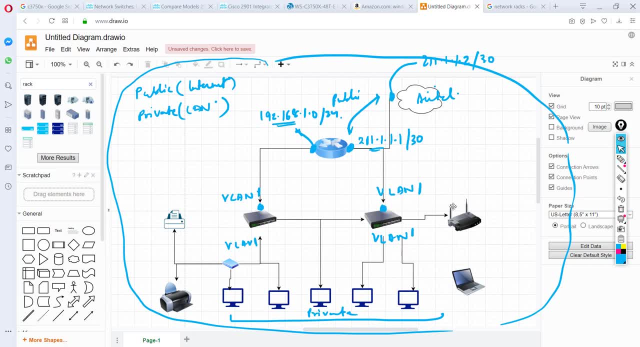 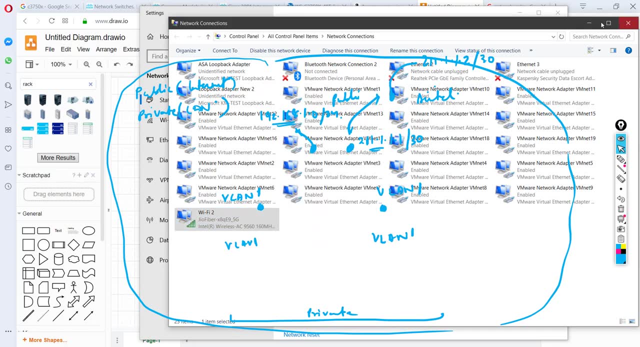 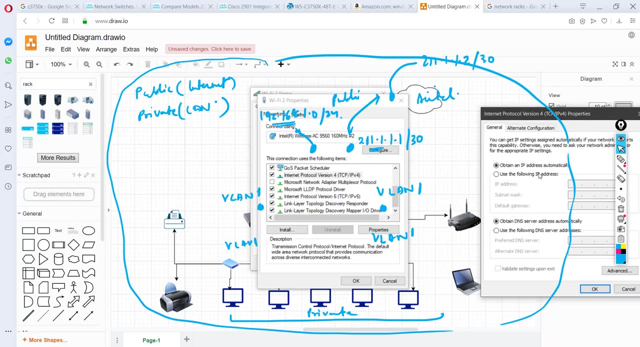 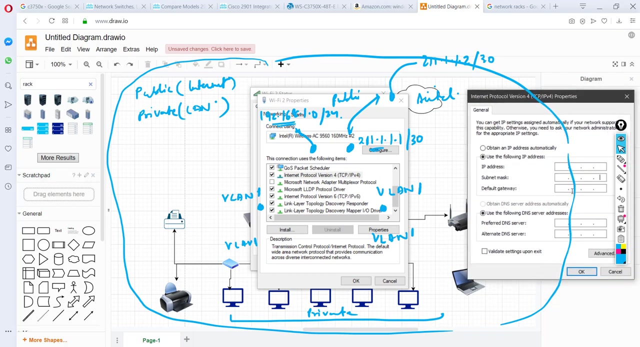 So let me show you what are the two ways. If I open up the adapters, if this is my wifi modem or a NIC card, okay. So the two ways are static way. okay. Static way is If I type the IP address myself, subnet myself, and I configure: it is called IP, it is called. 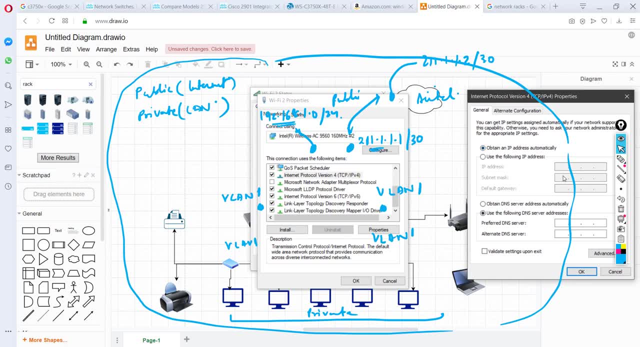 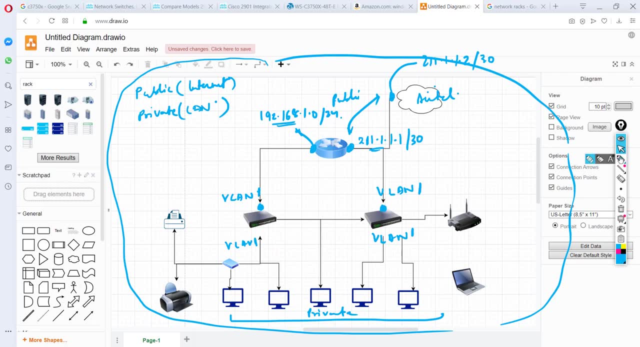 static IP address or to get directly from the DHCP. okay, So both can be done and both will be shown up in the later on labs. okay, For now, let's consider we are going to give the static IP, So I'm going to give static IP 192.168.1.1.24.. 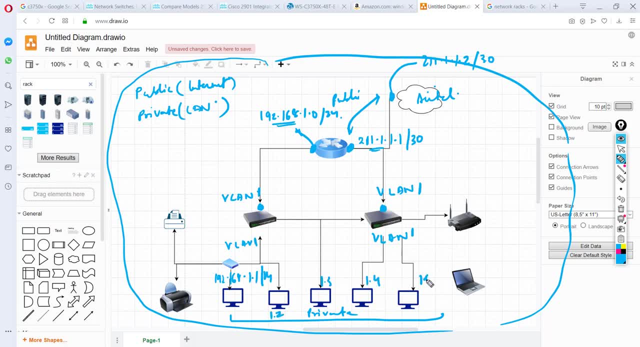 This is 1.2.. This is 1.3, 1.4,, 1.5.. This is on 1.6, 1.7,, 1.8, 1.9.. So we are now one single office, okay. 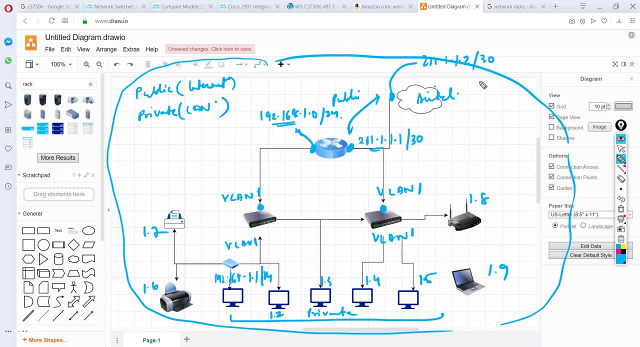 We all users- are falling under one single network. okay, So this is how we are going to communicate and this is how we are going to design the network. okay, So this is very basic thing. We can see few more Examples, okay, where we can have two different networks or we have interconnections of network. 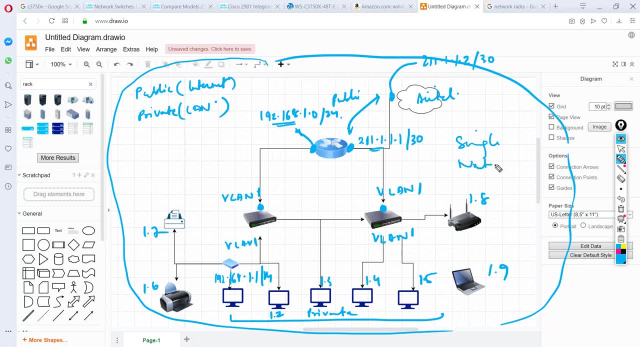 So basically, this is single network. okay, Single network, Sir. Yeah, Sir, you have given a ISP to the interface, to the router, then to the suite. you have given a private IP, both of them. So why we can't give the real IP to the router? 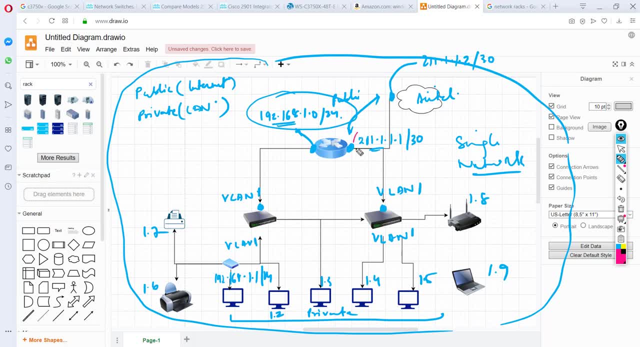 Okay, So it switches in this range, In this range. Yes, sir, See, actually you mean to say this range. you want to give it over here everywhere? Yes, sir, Okay, so thing is, public IPs are in very scared city. okay, For example. see, we have not started up IP address. but let me just brief you the population. 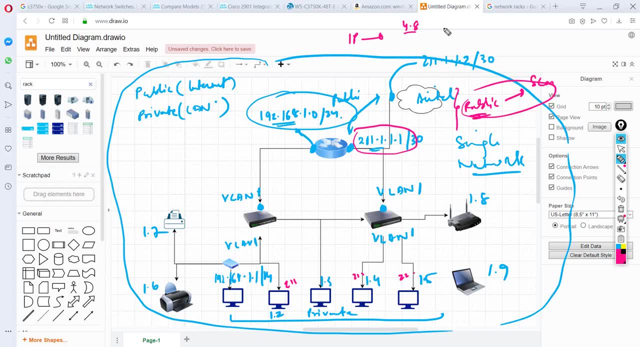 all over the world is around like 4.8 billions okay, 8 billions okay, whereas your ipv4 address are only 3.8 if you count even one ip address to one person. this should have been exhausted by now, but you know that everyone has one. 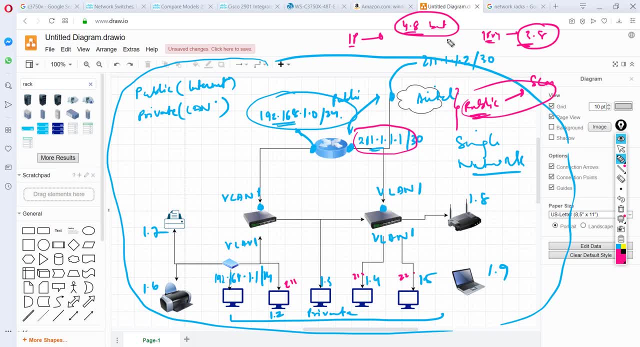 one laptop, one mobile, one uh tab, maybe some has two systems, right, so there is scarcity of public ips. okay, so isp is not going to give you 10 public ip, they are going to give you only one public ip. okay, every company will have only one public ip. we internally have to make use of our. 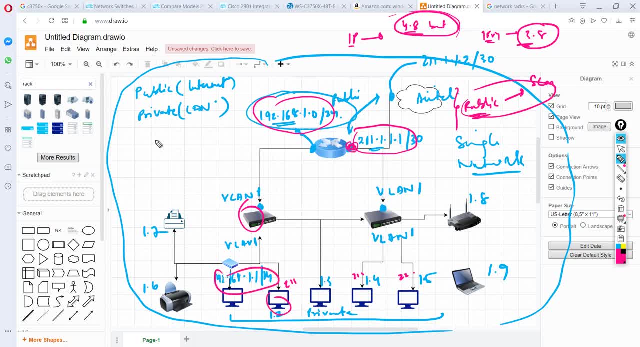 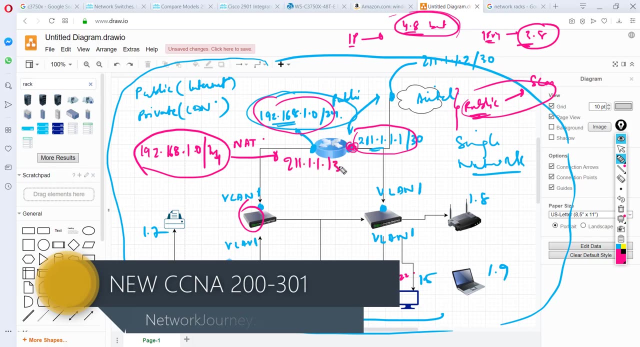 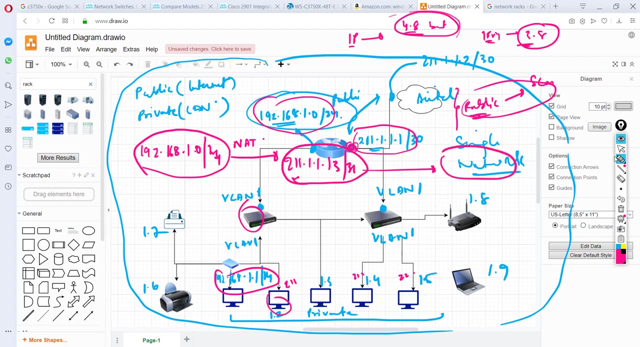 internal or the private networks, okay, and then this private network, whatever we have designed, we have to make use of technology called natting. natting is nothing, but our private network will be mapped with public ip, okay, and this public ip will be taken forwarded. i'll give you one small example now. uh, so, let me, let me erase this, okay. so if you, 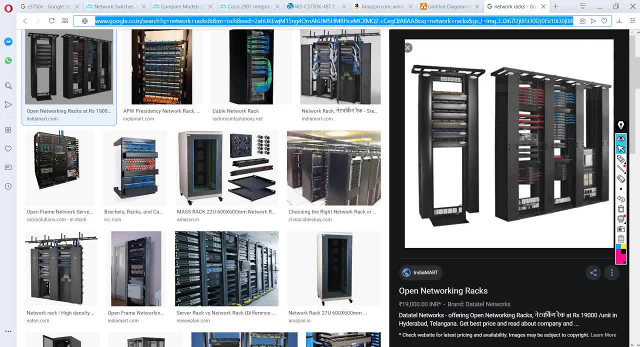 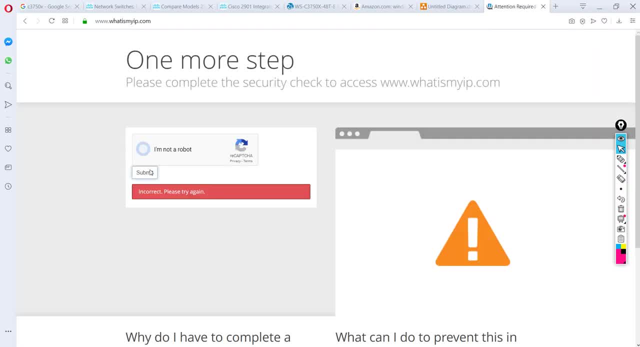 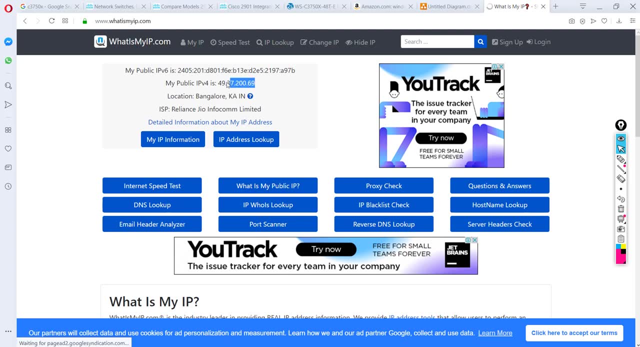 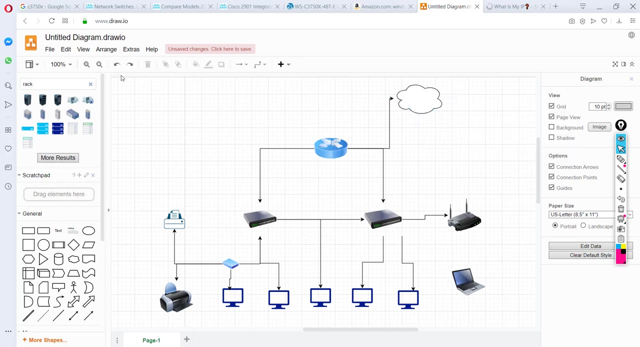 see from my uh laptop point of view. let me check what is my ip, which my isp has given to me. okay, so my isp has given me, uh, some public ip. this is my public ip. i'm going to take this and put somewhere here so that i can explain you. 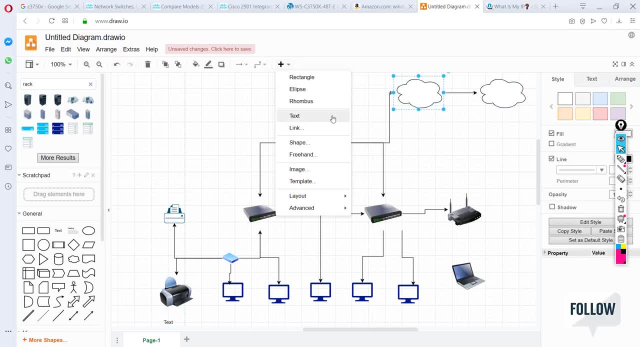 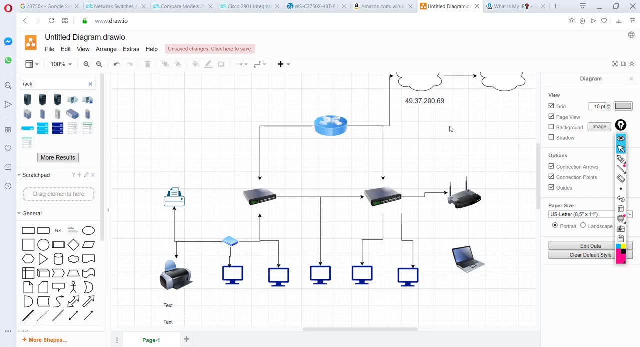 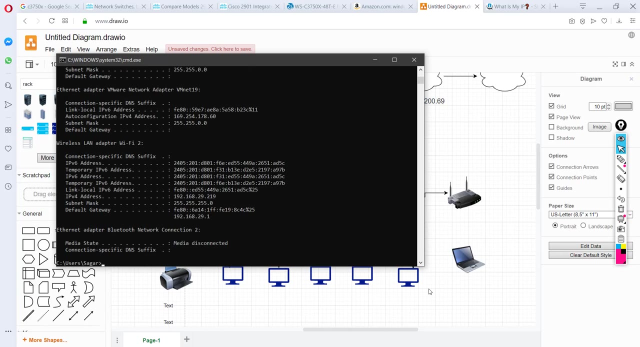 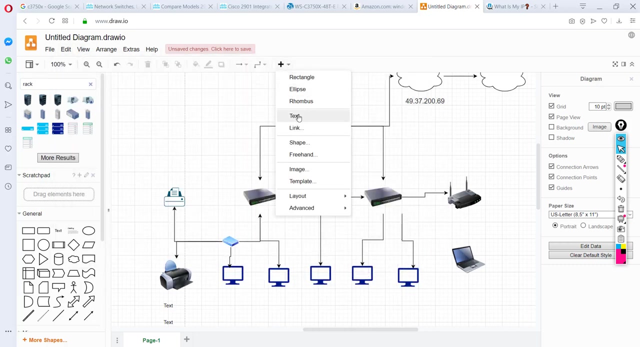 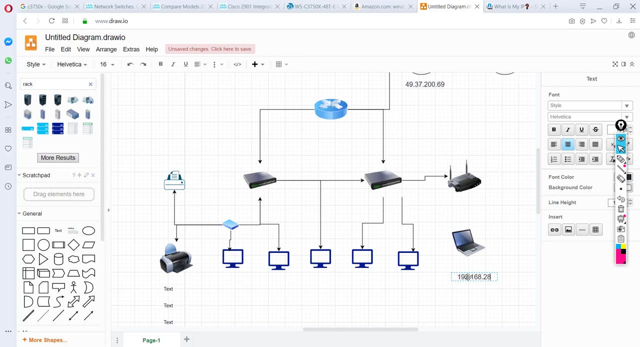 let's say isp has given me ip address of this over here, okay, but in real, what is my laptop? arc laptop, ip, let let's see that on. so this is my ip address. it is in private network, okay. so let's say, over here, this is my laptop and I'm going to run on 192.168.28.219. okay, the reason is ISP cannot give a single IP address to every users because of the scarcity of public IP. okay, so what ISP is going to do is ISP is going to give one public IP to all the users. okay, so we users have to make use of. 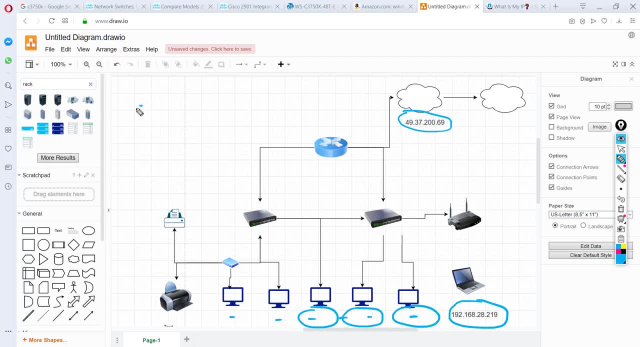 some private IPs. this is because of the scarcity of IP v4. that is why we have in new concept of v6. okay so IP v6. if we, everyone have IP v6, then for next 50 years we don't have to worry. okay, so these are. these are some topic which we 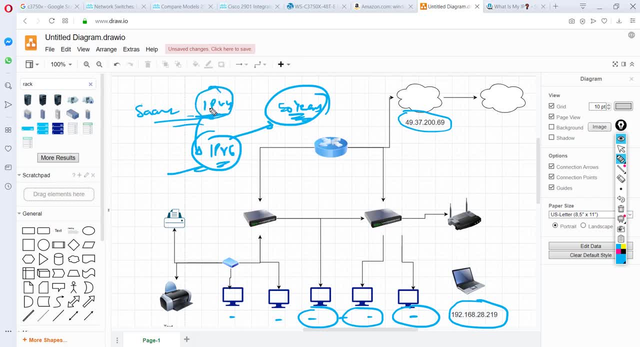 will check out later. okay, you like how we are still using IP v4. we should have been completely moved on IP v6, but that is not true, right, we still make use of IP v4. okay, why, why? so what is the reason? okay, so those things we will check out later, but for a fact just. 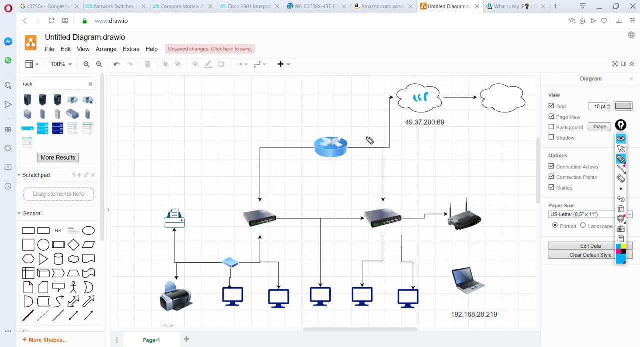 remember, ISP is going to give us one IP, or two IP at the most. okay, so this is one IP which is used by all the users, different users, to go internet. okay, and we make use of a concept is called NAT. okay, yes, so we can use any, any private of any class, if it is class a, class B, class C. we. 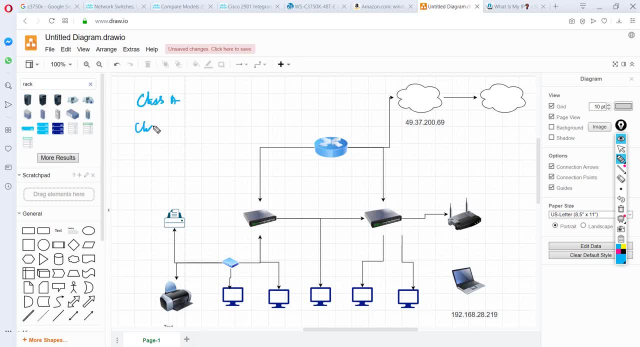 go with- yeah, we go with different classes okay: class A, class B, class C. okay. so for especially if classy are used for users, okay, because we get a lot of users: 254 ips in class c. okay, so 254 users are like number of users, which are, uh, okay. okay for us. 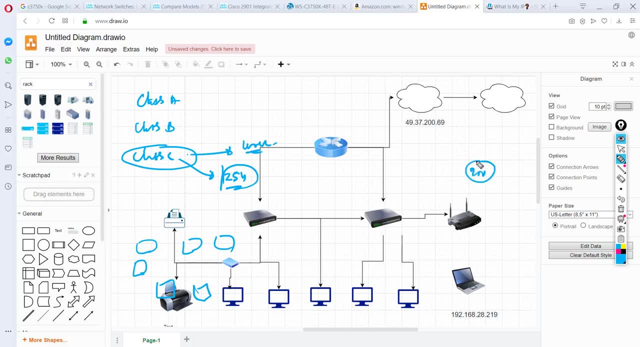 if for a, like a small company of 20 users or 200 users, class c is okay. if imagine i have some servers like vmware or all those things where might be, i have the requirement of thousands vms, so in that case i can go with class a okay. so yes, we can go with any. 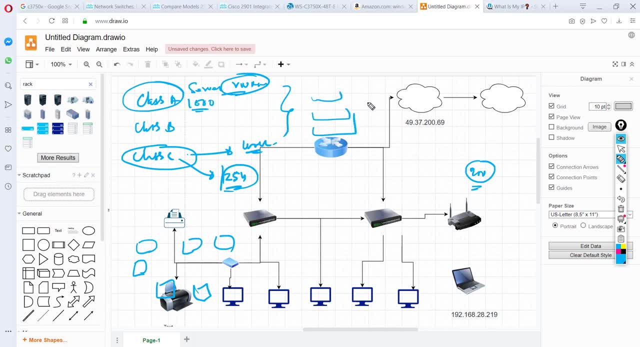 private ips, depending upon our network requirement. okay, thank you. thank you, sir. okay, fine. so so any other doubt uh on setting up this, or uh, or or anything is also okay, fine, okay, there is the doubt that these switches are compatible like ip servicing, which is uh know. 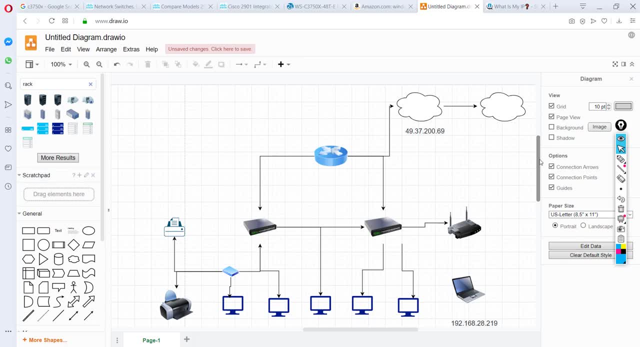 the routing and all. then if we know the routing, then why do we need separate outer? actually, the thing is, these are full-fledged routers which which are used for running the protocols like bgp protocols, okay. so the thing is, these are full-fledged routers which which are used for running the protocols like bgp protocols, okay. 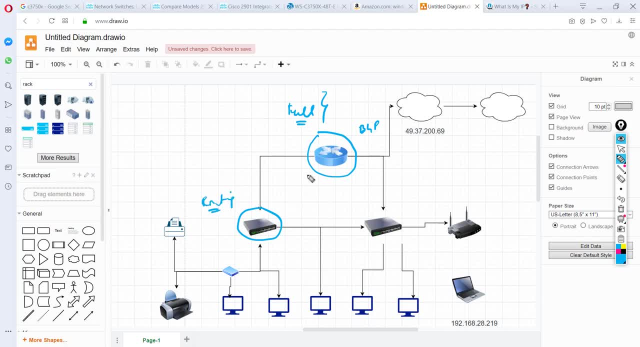 Whereas these routing features are not meant for the routing protocol. These are meant, let's say, to define some default gateways. What is default gateway? Like I told you, if this is an IP address 1.1, if I'm setting up subnet mask and if 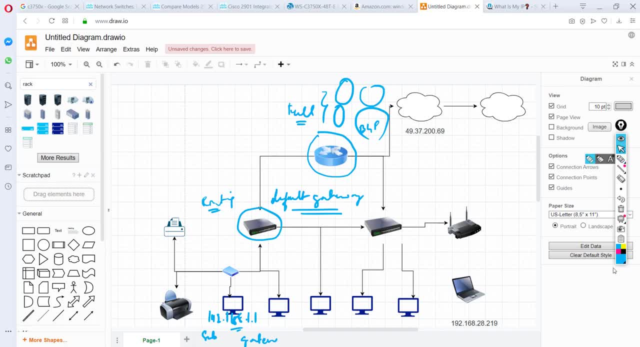 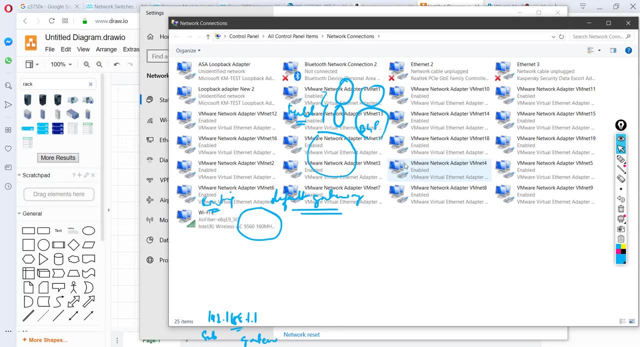 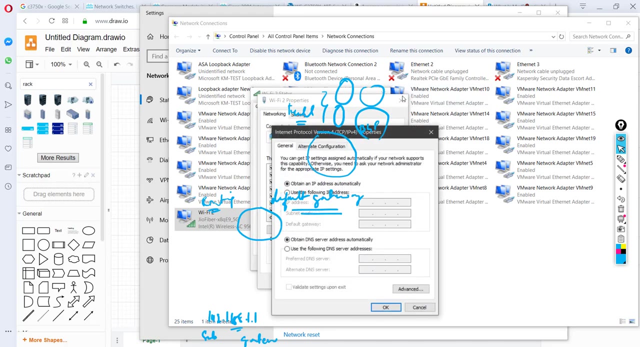 I'm setting up default gateway. let me show you once again If I go to adapters, when I'm setting up static IP, there are three fields which I have to fill it up. Then only it comes to know who is the gateway. 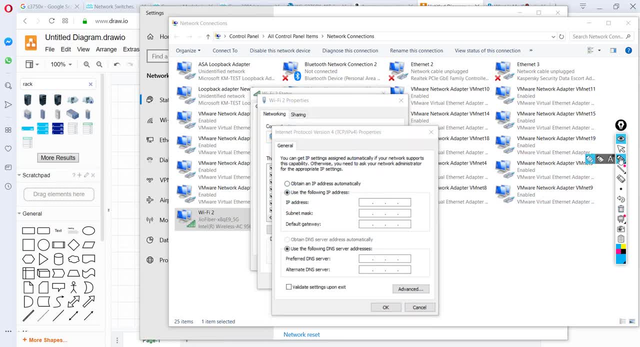 Let me click on static. So if you see, now I have to give one IP- This is my user IP- Then I have to give the subnet mask. This is that routing which we are talking about in IP services. So your switch should be capable of knowing us a little bit on routing so it understands. 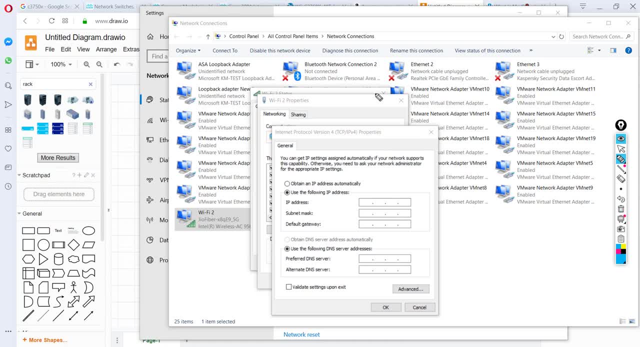 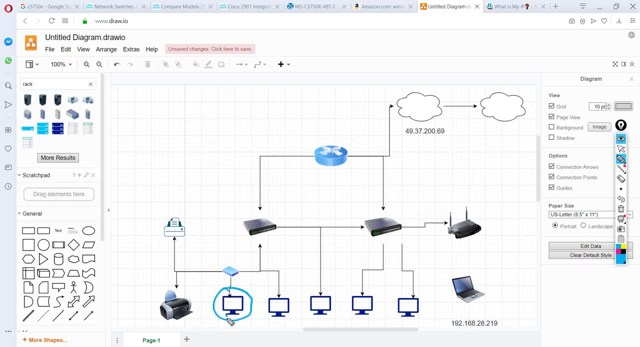 the meaning of gateway. So in our example, in our diagram, let's say: this is our diagram, So when I'm configuring default gateway, that is IP address of this. So basically it's a gateway. It is going in this direction. 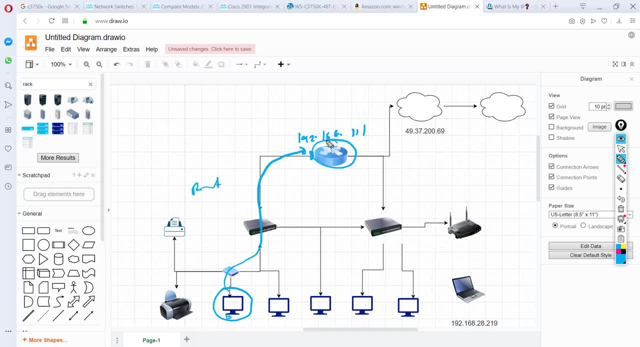 So that is the routing we are discussing, whereas a full fledged router, we are talking about OSPF, We are talking about BGP or any other routing that we can enable, like MPLS, like VPNs, which we cannot do on this. 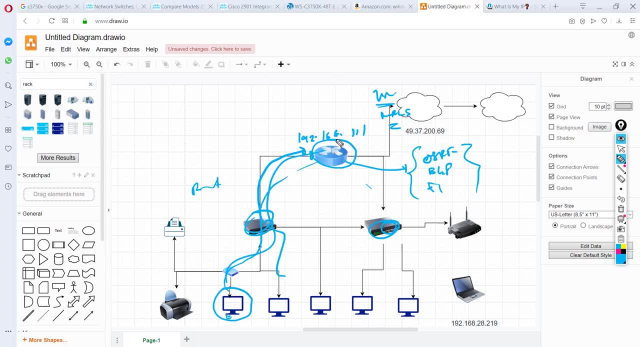 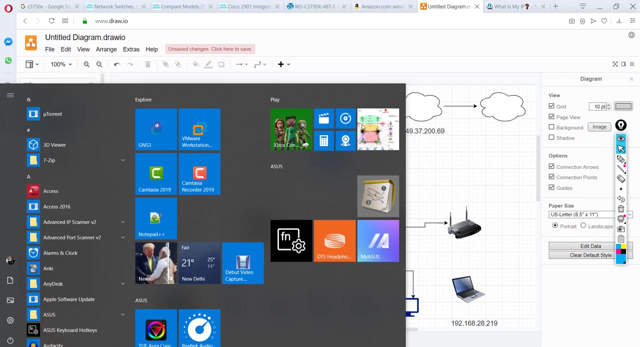 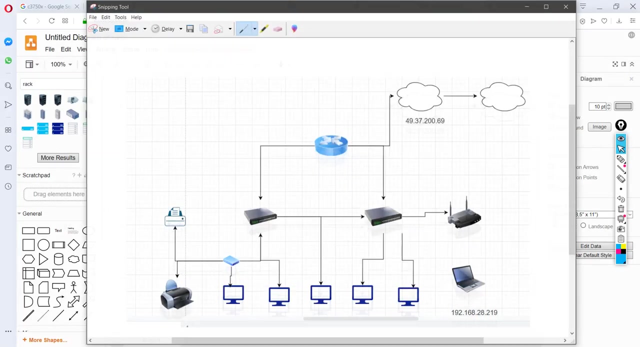 These routings are very basic, like for a user level of routing or something. Okay, So any further doubt here in the orientation or placement, So I'll just take the screenshot so that I can send it over on WhatsApp. Yes, The default gateway should be the interface which is attached to the switch or the interface. 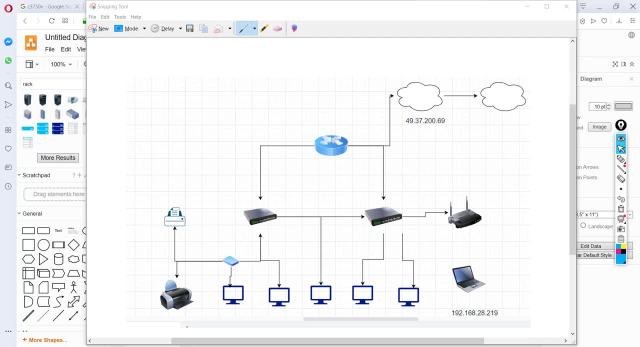 which is the What do you call router? right, Yeah, Yeah, Default will be on the router. Okay, Say, for example, the router has an IP one ninety two, one sixty eight, one dot one. So this is the default gateway, not not this, because this is working on VLAN concept. 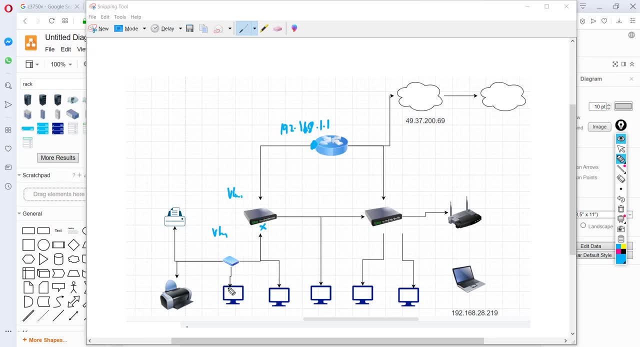 Okay, So normally what happens is, let me tell, in packet level. So once you're initiating some data, Okay, Data is called as Ethernet here. So Ethernet is going over here. The switch, what does which do it? do It does the work of flooding or broadcasting. 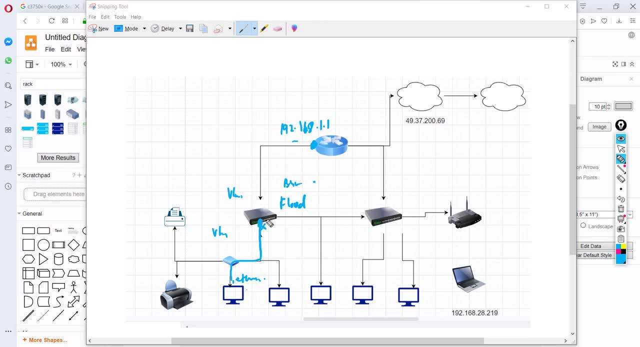 Okay, It doesn't understand IP. What it does is whatever switch port we can see connected, like this is connected and this can in this example, and this is connected. It is going to broadcast on both. Okay, Now, this is also traveling and this is also traveling. 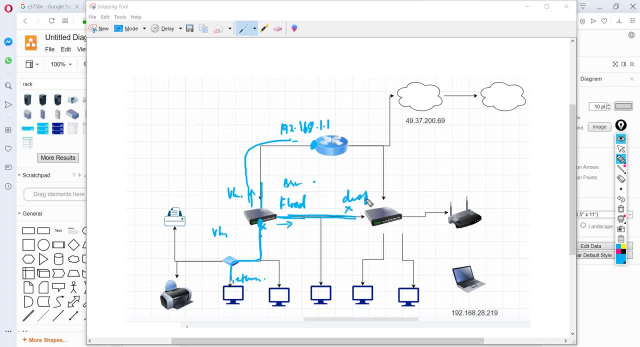 But unfortunately This one will get dropped, because IP is one dot one which is mapped over here. So this packet is going to survive and then this is going to respond back, whereas this is going to drop. Okay, So the default behavior of a switch is like: let's say, this is a switch. 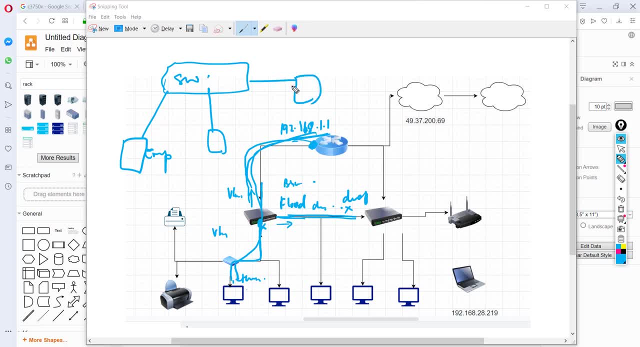 This is a computer. I have multiple computers. Okay, So I'm I'm sending a ping message. So, basically, this is going and hitting up on this. The switch is doing broadcast on all the available connections. Okay, Might be. I'm pinging this person. 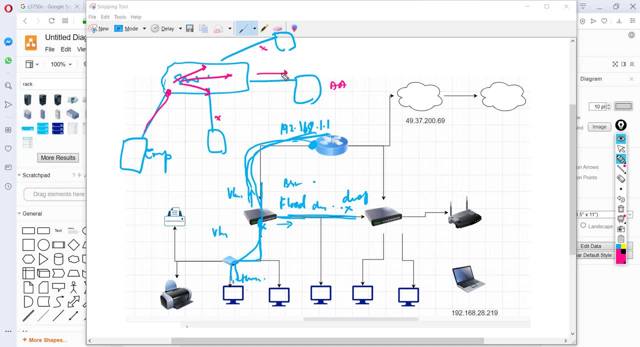 So rest of them are going to discard and this is going to respond and it is going to reply back and that is going to be sent back. So that is how the switch understand uh, the ARP. Okay, So we will see this in the uh switch configuration like how switch learns the Mac address. how. 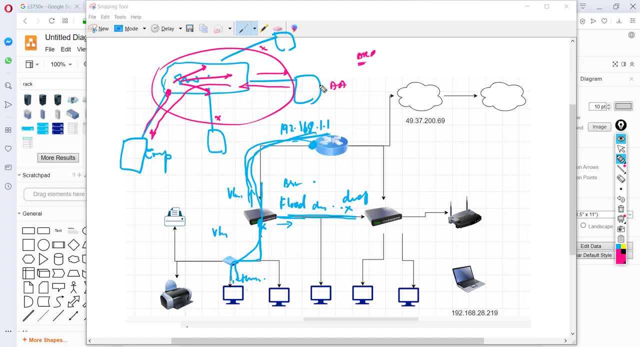 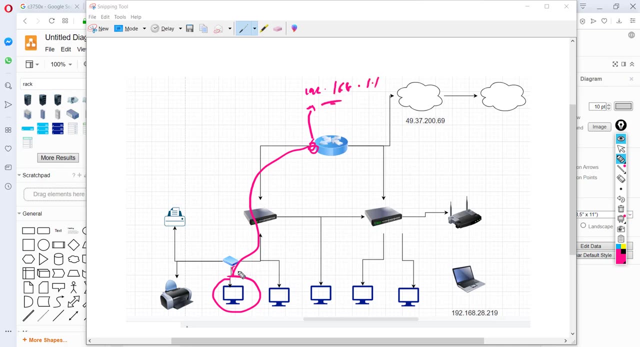 what happens within the switch. Okay, So that we will see, uh, in the switching topics. Okay, So for your question the gateway is this: on on this, like 192, 168, 1.1, because if you want to go out, so basically this should be hit and then router should send back. 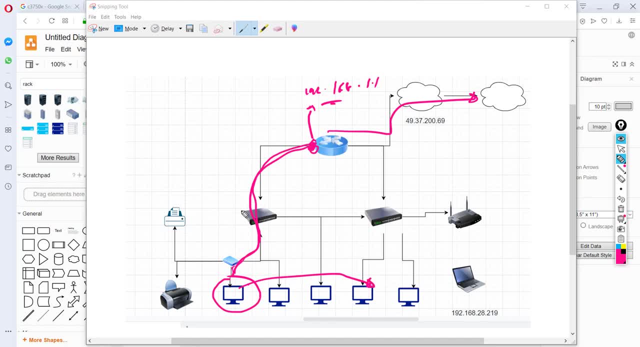 Whereas if you're just communicating between two computers, then IP is of no use, because they are part of data link layer. In data link layer, VLAN is a constant. Okay, If they fall in one VLAN, let's say this is VLAN one. 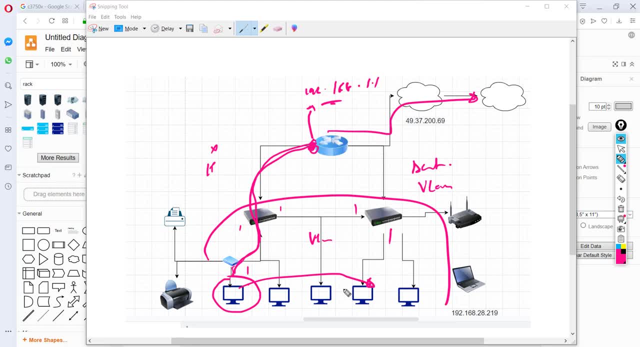 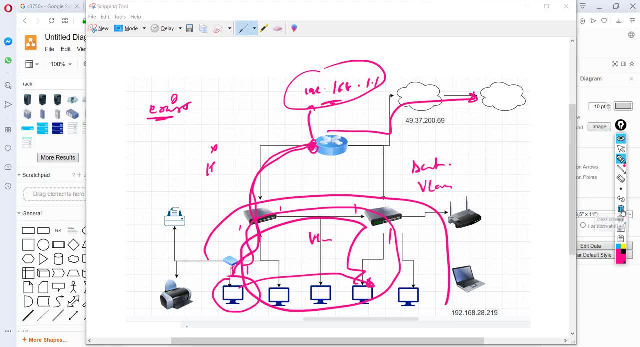 Yes, We have two interface to this. Right, Right, Yes, Which is given by private? Okay, Which is given by private IP, Different IPs, Just like 192.168.1.1 for one switch and 192.168.1.4 for another switch. 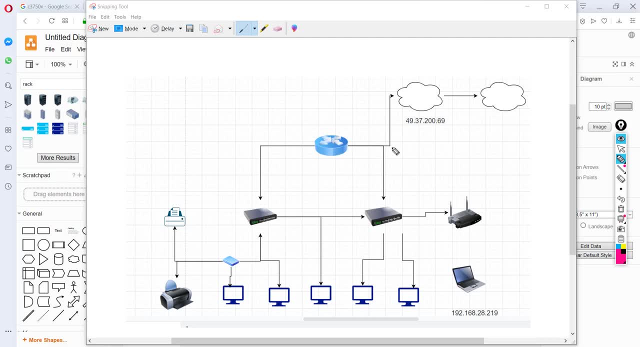 Yes, For example, Yes, If you did for one switch submitting and another for not submitting, that these two switches get communicated. See when. imagine, like what you're telling now, 192.168.1.1 on this side. Okay. 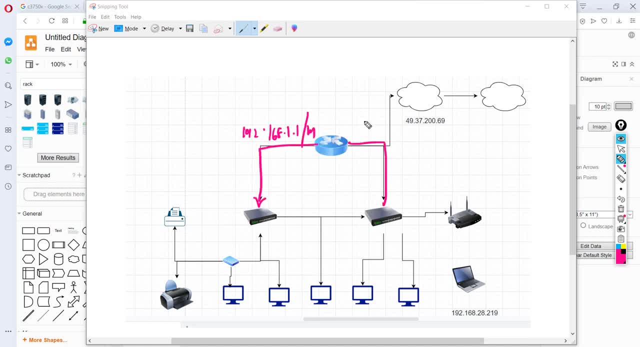 On on the other side, let's say, some different network. So this is what you're telling, right? Two different networks. Yes, Yes, Okay. So in this case, we have a concept of inter VLAN, Okay. So, basically, if I want to communicate between two different networks, I need to have L3. 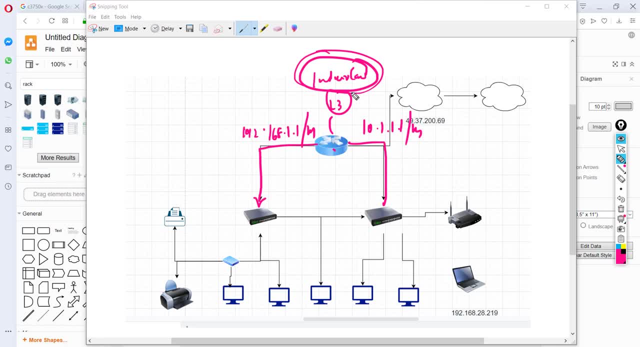 capable router and then the concept is called as inter VLAN. Okay, So we will check this in all switching uh topics, How we communicate between two different uh subnets. Okay, But yes, it is possible with the help of inter VLAN. 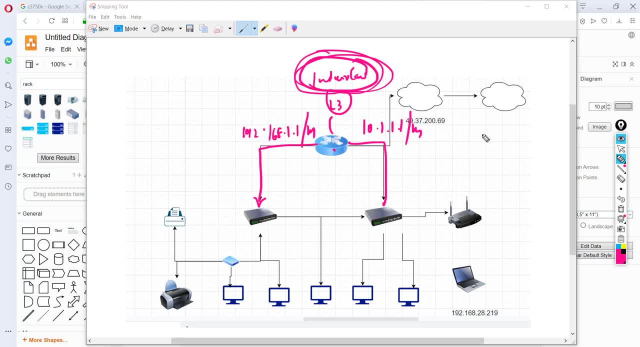 Yes, Yes, So the default gateway we have to configure on the switch, that we have to give the default gateway to 192.168.1.1 on the switch itself we have to configure. No, no, This is on this router. 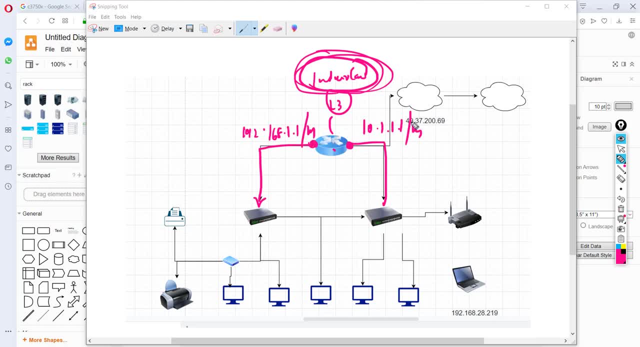 Interface of router. Yeah, Do we need to configure? Yes, Do we need to configure? No, no, no switch. They are all part of VLAN VLAN concept, like VLAN one. So we we don't have any thing to be configured in this switch. 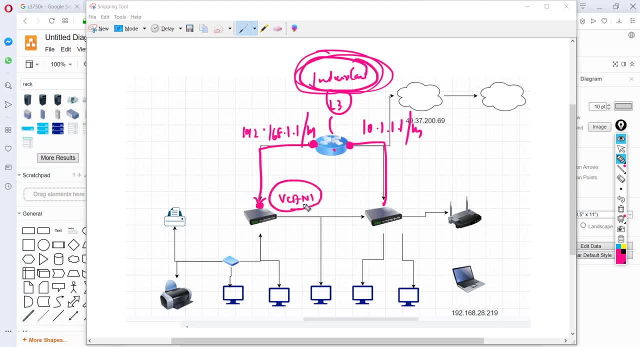 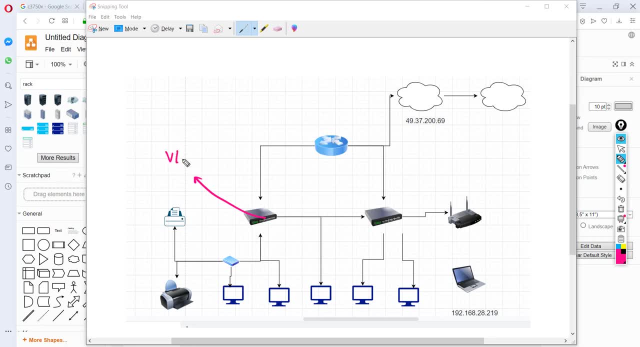 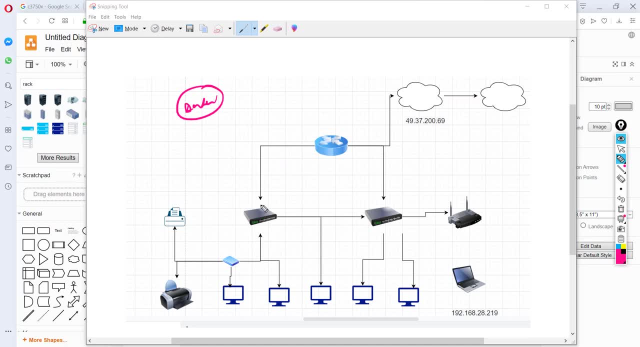 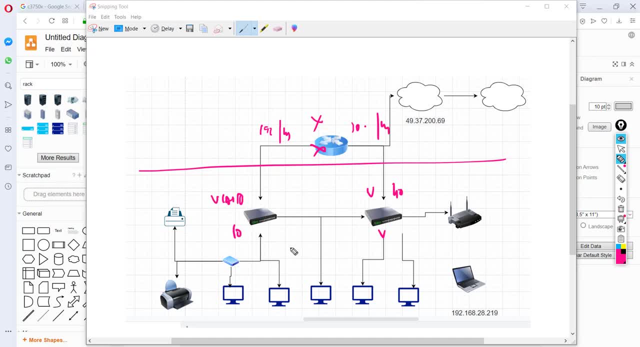 if you exclude router, then these two will not communicate. okay, they are going to be two different things. this is separate and this is separate. okay, now, in order to communicate between two different subnet, I am going to place one router and then I am going to allow inter VLAN. okay, when I allow. 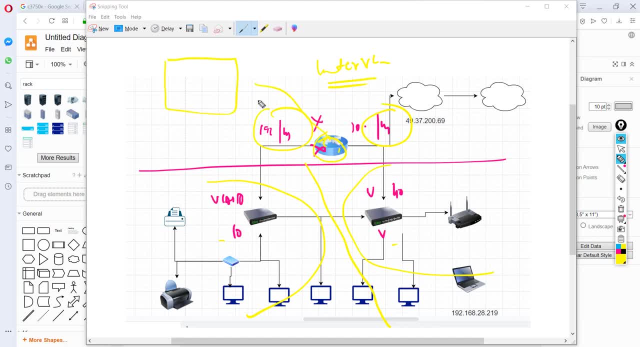 inter VLAN router will understand the routing table and all the things are going to get placed within the routing table and then your div. two different networks can communicate each other. okay, let's say, if this is communicating to this, so it has to go via this direction, okay. 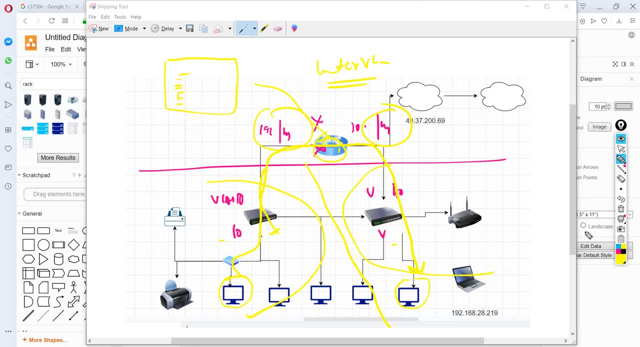 this is in case of two different VLANs, two different networks. okay, don't worry, we have lot of labs while we are doing these things. okay, so we will cover up everything and that in the switching labs. yes, you mean to say from this which to this, which? see, yeah, I already answered that lock long. 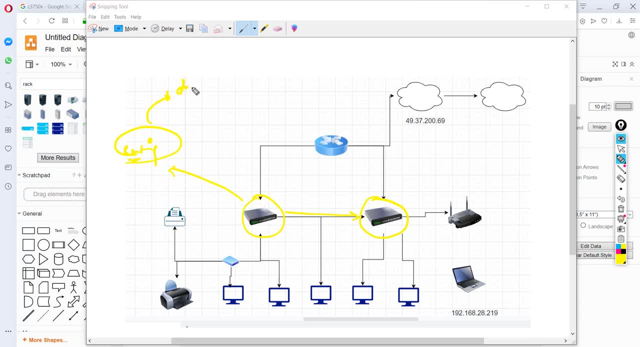 back. okay, the routing here is routing related to default, to gateways, okay, whereas the routing that have over here it's all eigrp, bgp, mpls, all those things. okay, so that routing is different and the default gateway is different, okay, yeah, so see again. one more thing: the switches comes in two. 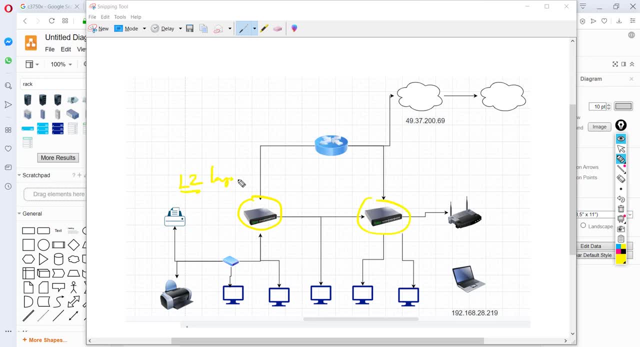 different flavor. one is called l2 layer which only understand l2 technology. there are some switches which is capable of l3, also l2, okay. so imagine if i take this router out and i plug that switch which is capable of l3 and l2. okay, so now, in this case, this can understand all bgp, all those things. 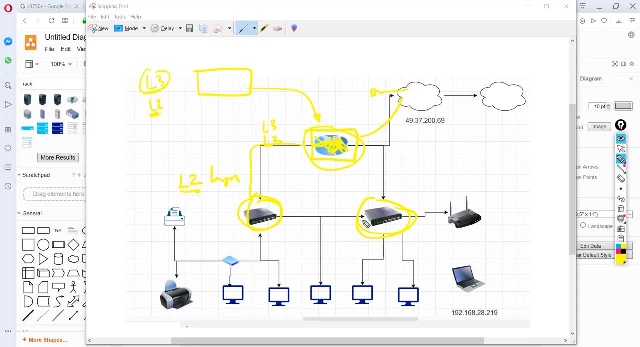 and same time, it can also understand the internal subnets- okay. so again, it all depends on the network design. this is designed in terms of cost cutting- okay, l3 plus l2 switch is going to cost you a very high amount, whereas a simple router can cost you like two hundred dollars. okay, yeah, so that is, that is what. 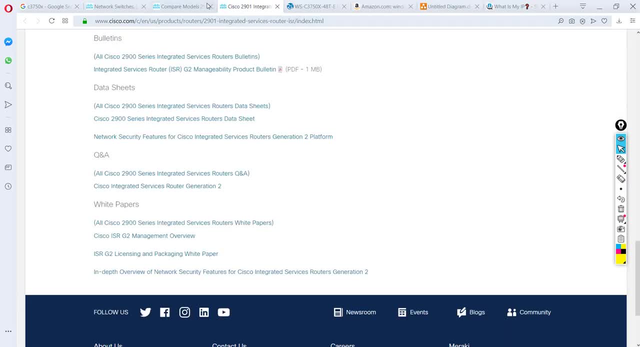 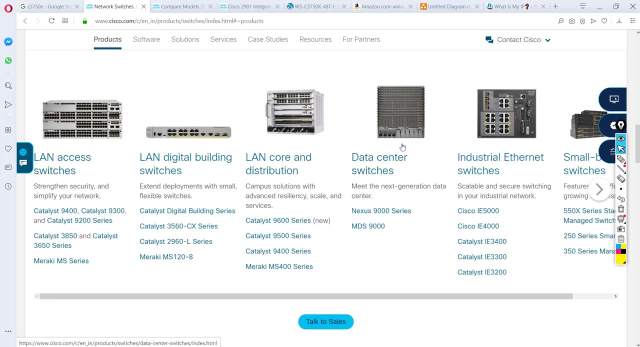 i was trying to show over in the cisco website. okay, if you see different variants like like this: okay, so these are all defined in terms of some cost cuttings. okay, we picked up device from this which is very less in cost. what you were recommending is something in this. okay, the 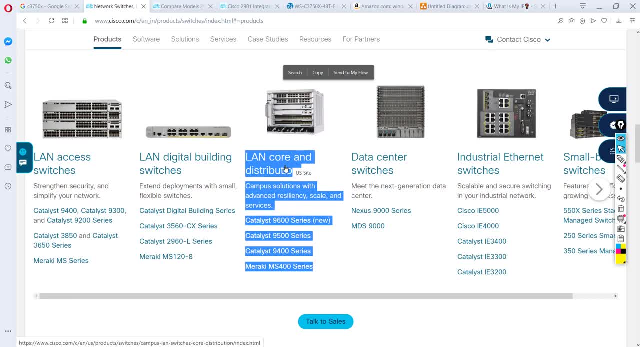 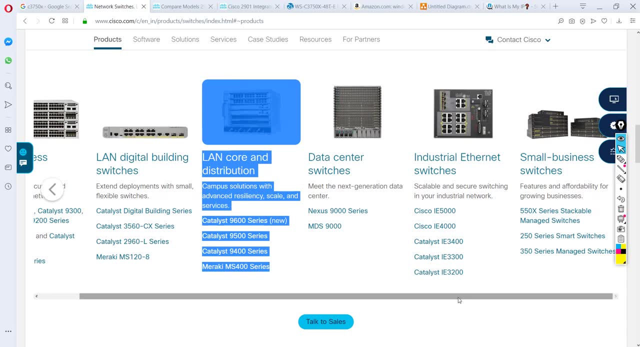 core which can do both the work- l3 as well as L2. these are very costly devices. we we place them in data centers where we need high throughput, like more or more packet transfer. so you can see, here for this we picked up and saved allária devices. okay, and now with this you can see everyone asked well. do you need a programmable left device? when do you need a mk2? right right now it is not. does that mean you actually need a mk2 device, like you could doUC right now? these are some thing here in the Joomla bevels. yeah, this is ok. so you do what we are doing, that is, will, when you want 105 things, we will have. 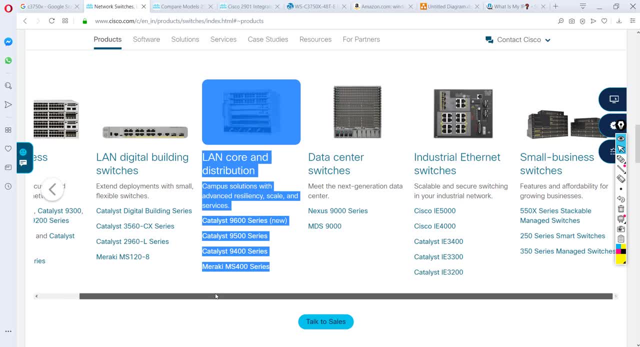 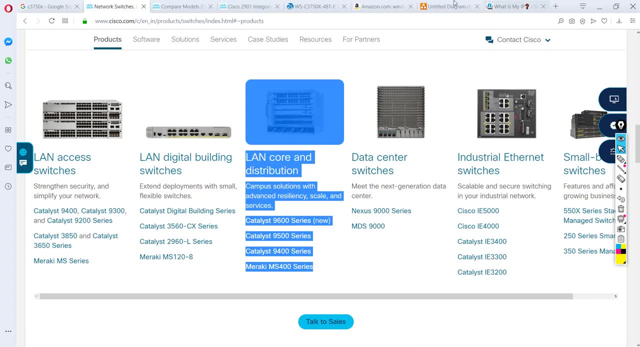 to increase the cost. now it is absolutelyен. i mean, if Teampoint links over, you can just do 100 models, transition or all those things, okay. so like, depending upon the cost, you can pick one of them, okay. so I I went with this design, just thinking of a concept. 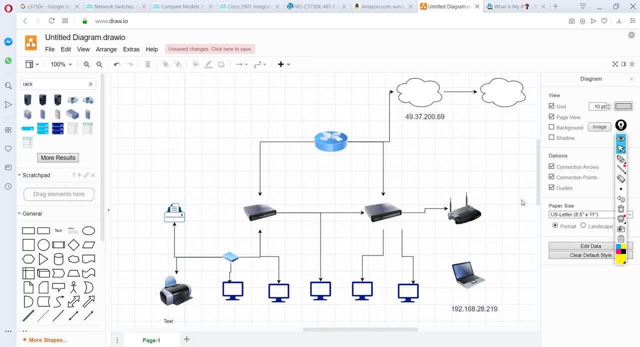 of small network or small network for a startup company, where, with this very minimum resource, I can build up my network. okay, so this is very simplest. you can do like n number of customization on this design to enhance this, to get it into like more advanced topology. okay, so let's go to slide once. 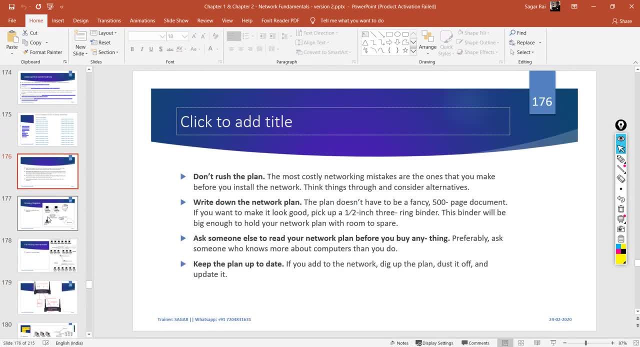 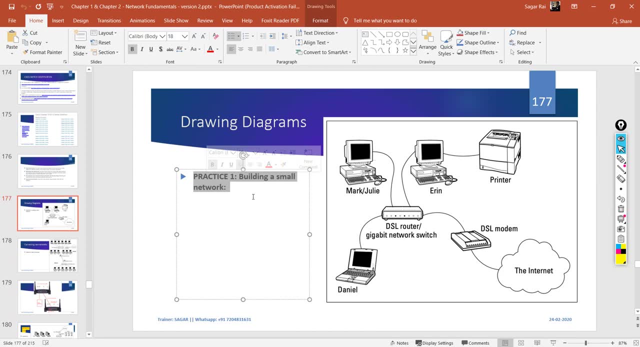 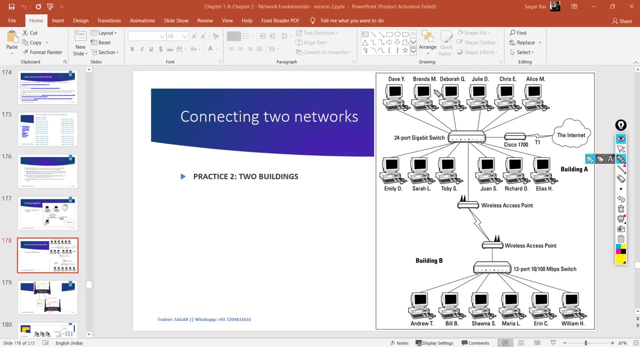 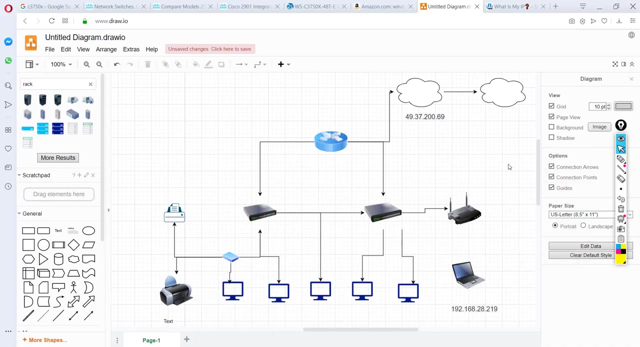 again. so we just did our first network design, okay, a very small network design where I considered only one building. okay, now let's say I have two different buildings. okay, with two different buildings and like more things coming in. let's say the network which we have here, okay, is getting expanded. we have more, more. 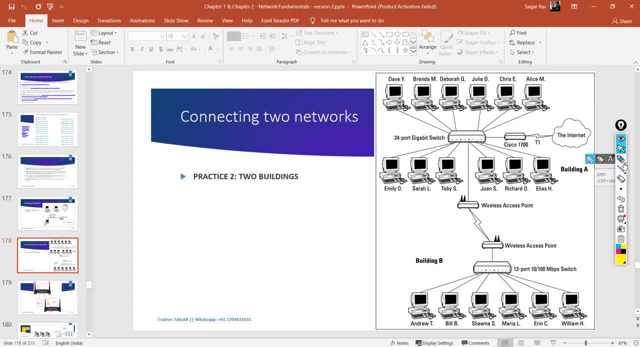 things coming in. okay, so you can just think that this is one building which we designed already. okay, now I have a requirement of another building, so I am deciding on a building and I want to design all the buildings building. okay, so, as per this design, what i can do is i can plug one wi-fi modem to another wi-fi. 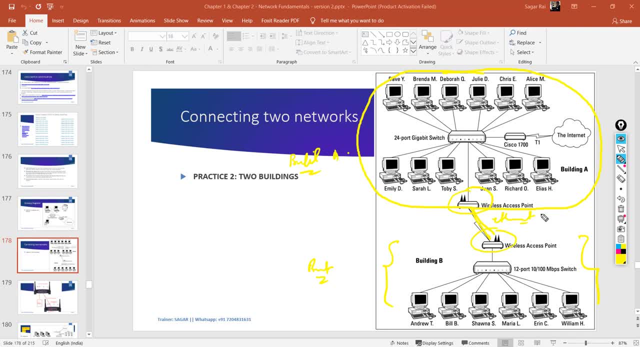 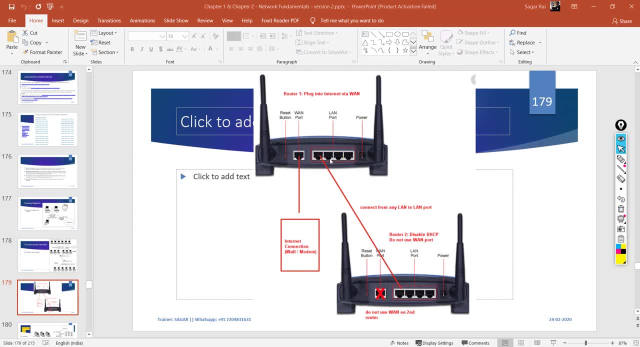 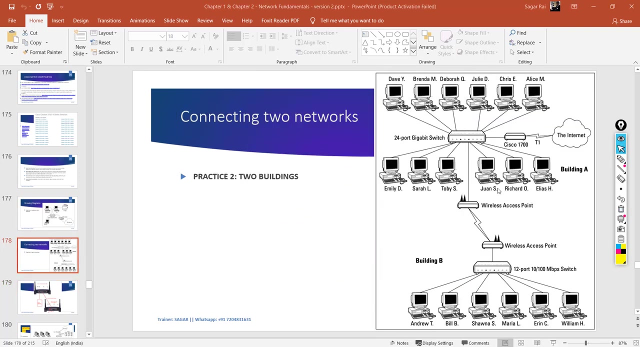 modem. i can connect one ethernet cable, okay, so something like this: one wi-fi modem to another wi-fi modem, i can connect a cable, a normal rj45 cable, and i can extend the network. okay again in terms of cost cutting. i'm talking about okay. there, there could. 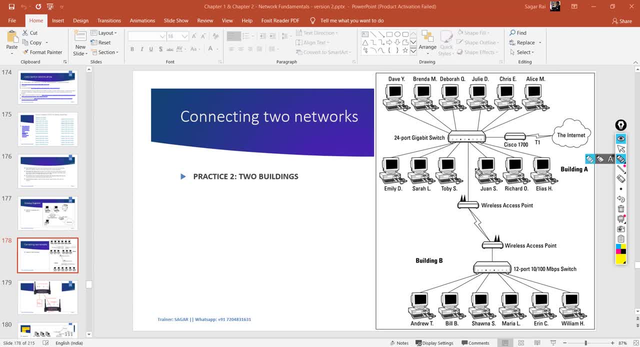 be there. there can be n number of uh things that we can do here. okay, instead of a modem, i can connect a switch. i can connect a switch, i can connect it. but in terms of cost, the modems are much more um lower in price rate. right, so i can just connect a cable, i can connect a layer to. 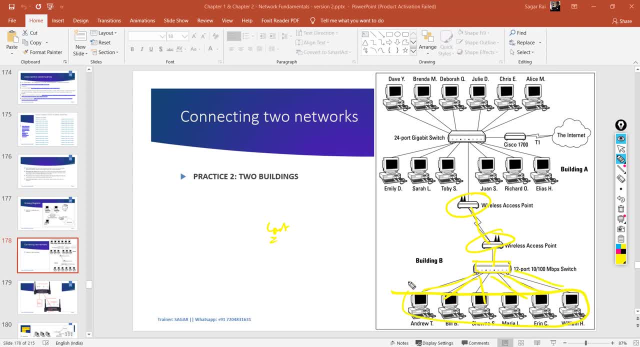 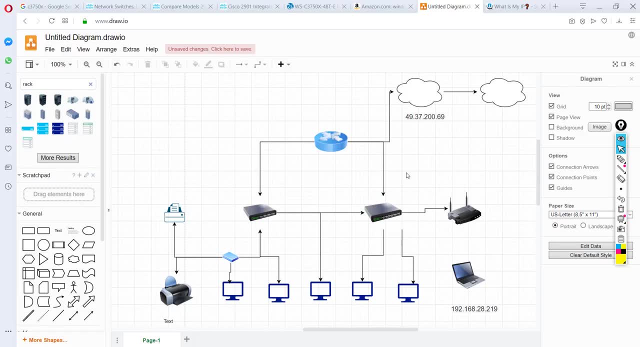 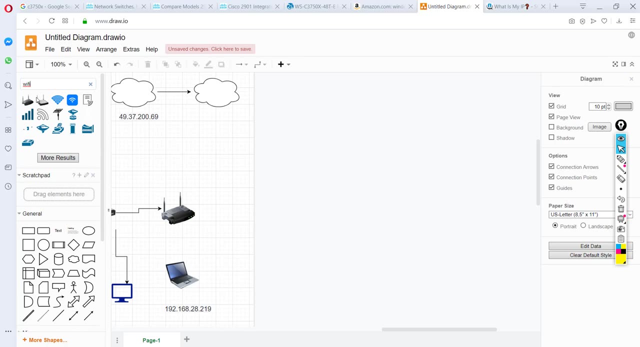 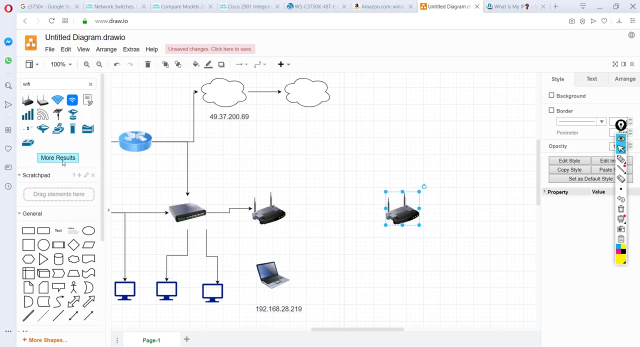 switch and i can extend to few more devices. okay, so, in case you guys want to give a try, so you guys can do it. okay, so you just have to do. what you have to do is you have to get one more. one more wi-fi model, okay, uh, and few computers. 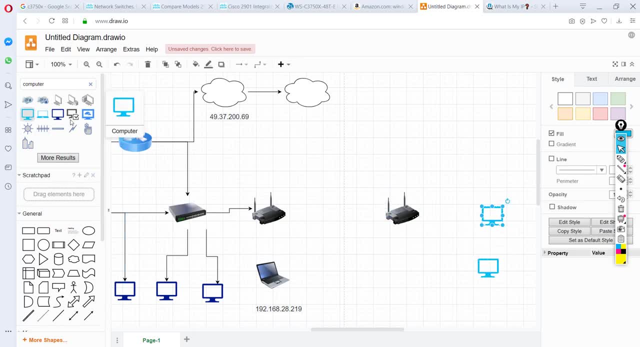 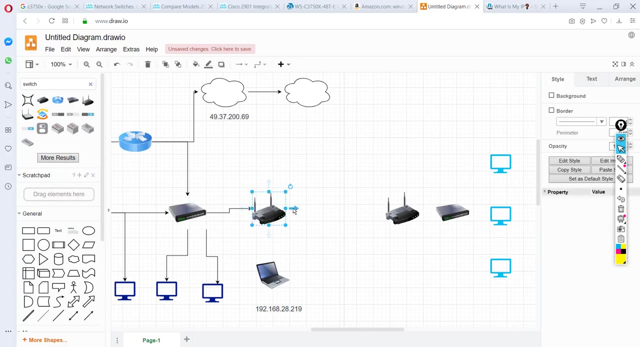 a layer to switch. okay, and now connect from this modem to this modem. this modem will be connected to a switch and then switch will be connected to end devices. okay, and again, these users, if they want to, uh, use internet, so their traffic will flow in this direction. okay, so this is, this is just a small design, just to understand, like how we can connect. 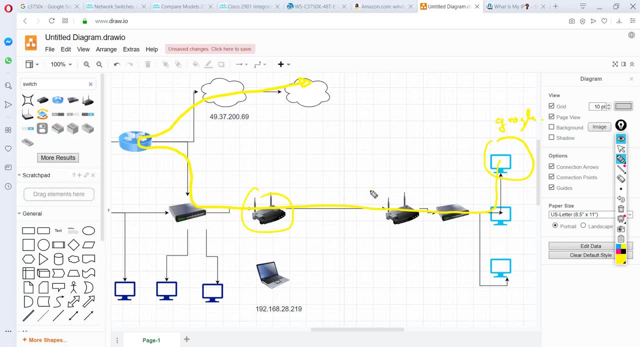 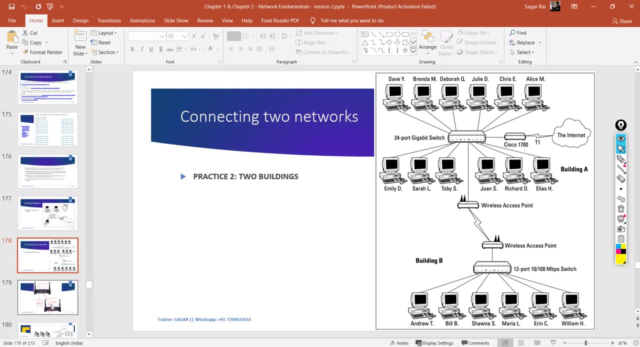 what? what are the possibilities? okay, so this is the simplest thing. like two modems, we can just connect individually. so basically how, how we do is so let's say, we have two modems, we can connect individual. so basically, how we do is so: let's say: 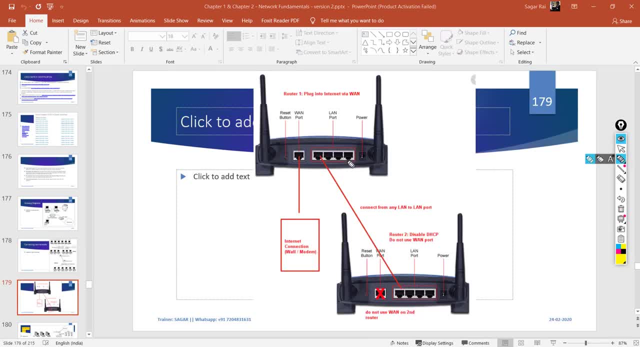 this is one modem on building number one. okay, so this is having the input from the layer 2 switch. so from this switch port I can lay a cable towards this and I can take the output directly from these. okay, so in case, if I have a layer, 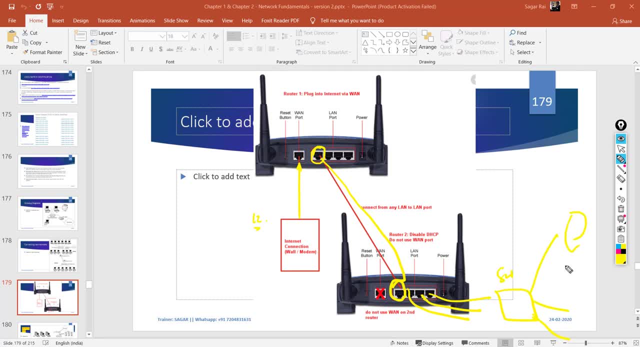 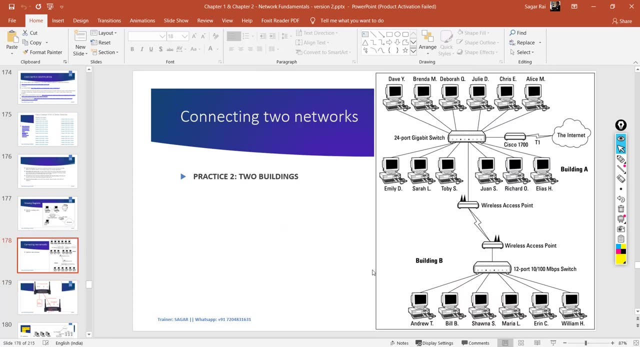 2 switch here. then switch can be connected to different computers. okay, if I have more computers coming in. so this is the case. okay, now if I need like say this, this design has some flaws. okay, the the drawback is I cannot have multiple networks, so whatever network I am sending it here, let's say this is VLAN 40. 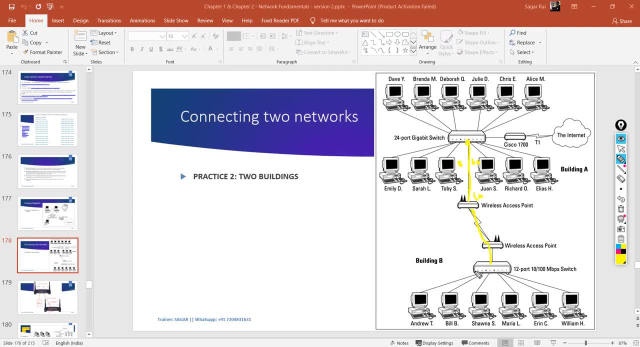 so basically, the 40 is coming here and it is coming over here and it is getting split right now. if I have different networks, like VLAN 20 or VLAN 30 or 40, in this case my Wi-Fi will not work for me. I have to keep some layer 2. 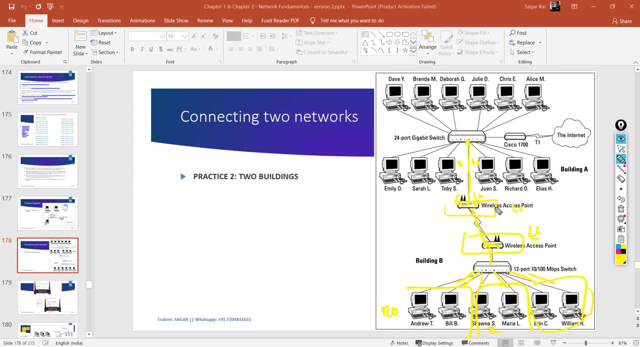 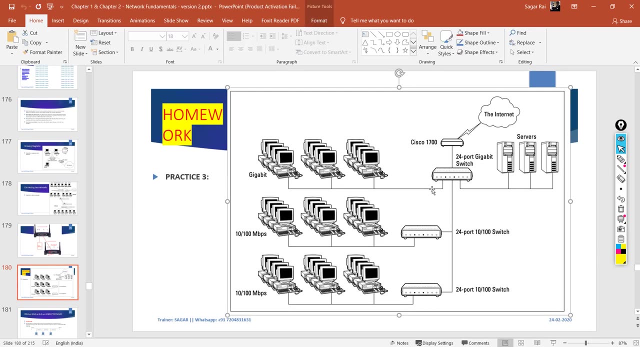 switch only, which is, which is manageable, which I can configure different VLANs, okay, so that is what. you can have any number of designs out of this, okay, and as a homework I would like to give you this design. okay, so you guys can try it out. on the software. 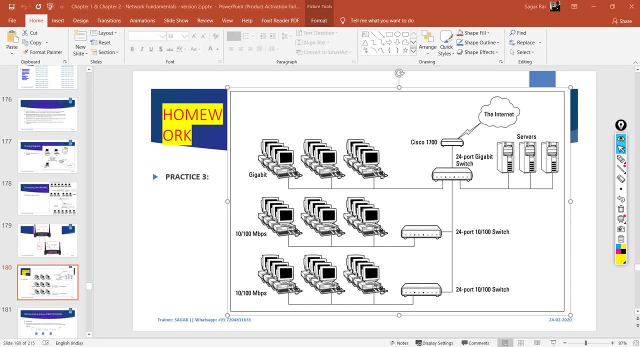 or the online tool which I gave you. so give a try. okay, try to configure something. so, basically, what you need to do is you need to do some computers here. just think of floor, like first floor, second floor, third floor and every floor. you have a switch, okay, and a switch is connected to the router and router is 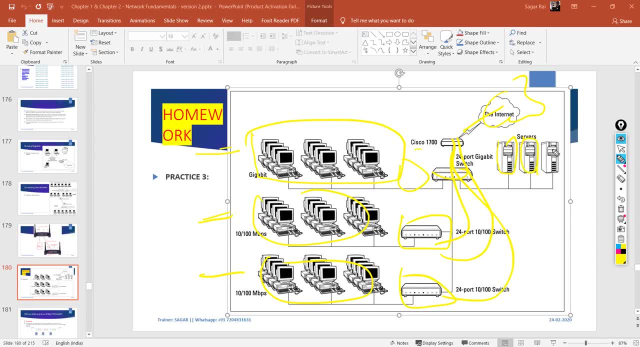 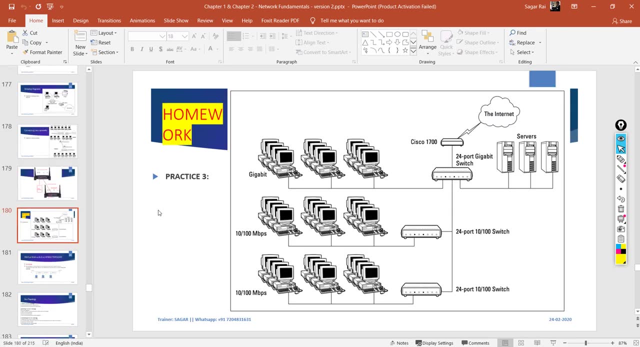 connected to internet. on the other side you have some servers. server is again connected to a layer 2 switch. okay, a simple design just for practicing, okay, fine, so. so any question on the design. but before I move on to the next topic, yes, we are connecting two routers and the two ends. 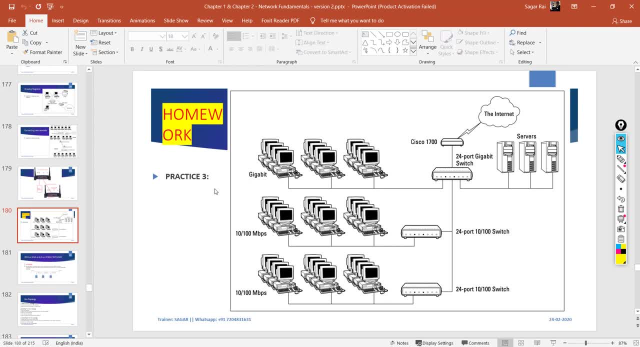 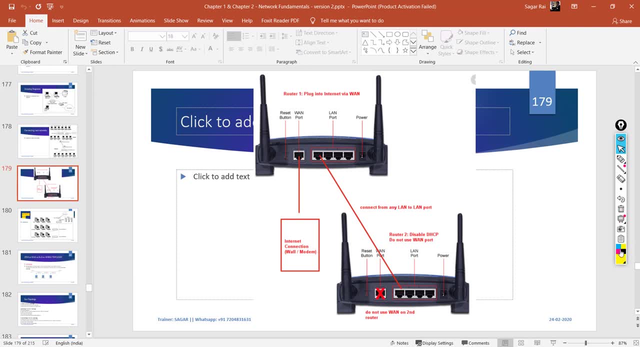 to connect the two switches. so can we get the same speed to this? another switch? we'll pick up later- and AMP innovative router is coming from another router. i didn't get you. please repeat your question, sir. we have a one network first floor. we have a one switch with the router and with the pieces another another floor. 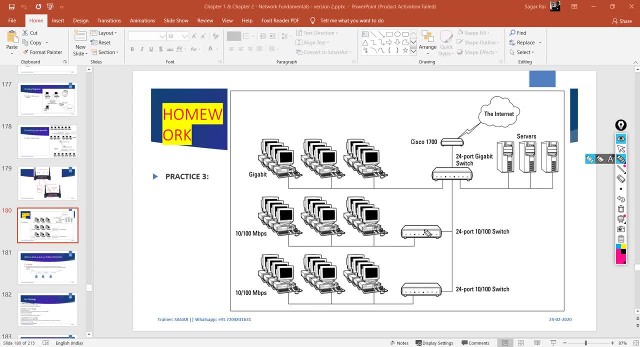 we have a one switch and the pieces and we have a one model which is coming which is connecting from first floor to the switch. so can we get the same speed to the router from the switch? are we getting a low, low speed? see, depends, depends, depends. what is your input here? what internet input you have? 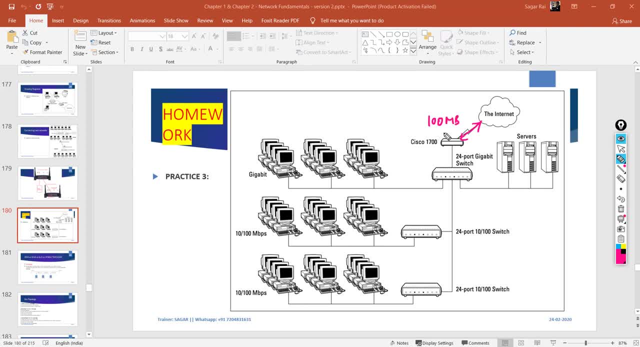 given here. let's say it is 100 mb. okay, so the 100 mb is getting divided into you guys, like it doesn't? it depends on the speed that you have purchased from isp. okay, and there is no uh need of keeping routers here. router is enough if you keep directly with here, which is connecting to internet. okay. 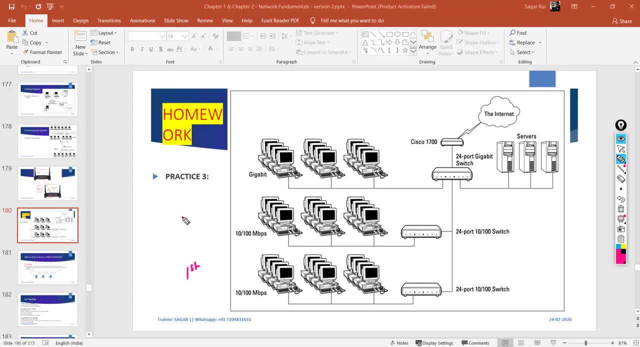 so, basically, if you're taking an example of first floor, second floor and third floor, so your computers are connected to layer two switch, the layer two switch will be connected to a main which, which is core switch, and that switch will be connected to router. okay, now, if you talk about 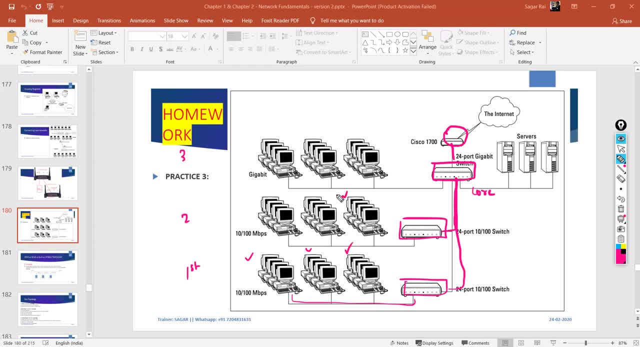 internet speed of this this, this, this, this. so basically they all will have a shared medium. okay, in case the speed is 20 mbps, so everyone should get, let's say, two, two, two, two. but it again depends on a computer. let's say, if the computer is running x, very excessive of. 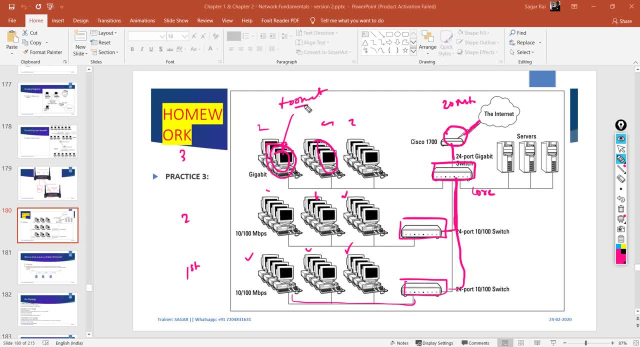 you tube or he is trying to download something from torrent. okay, so basically he is going to make use of 20 mb which was shared with other people. now other people will start complaining that my internet is slow. okay, that could be reason that this person is excessively using the internet. 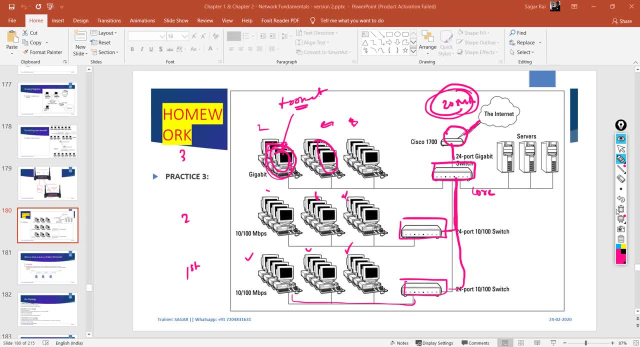 because it is a shared medium. right, you, you can, you can do on the modem if your modem is capable enough. so what you can do is, let's say, the mac address or the ip address of this is like 192, 168, 1.1. so you go, you can go to the modem and you can say that this person should get only one. 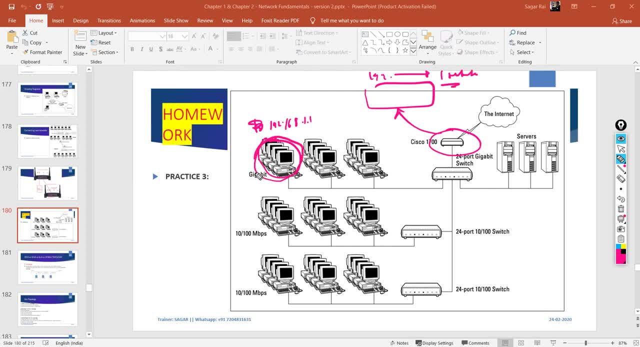 mbps, not more than that. now let him uh use any torrent or let him use any youtube to watch some movies. he will only get one mb. so other guys are not getting impacted. so that is your modem. which modem can do what you say modem? see, that is what modem, router, your third party controller, so basically anything. 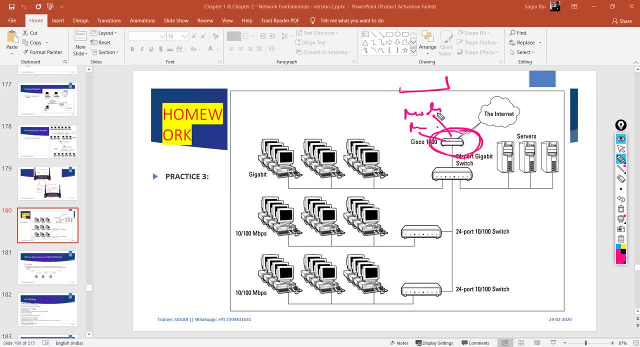 which is over here. it can be router, it can be modem. so basically modem router. see what is modem? basically we use it. whatever we use in home, uh, the home setup, we call it as modem, some people call it as router, some some people call it as internet. uh, modem, right. so? 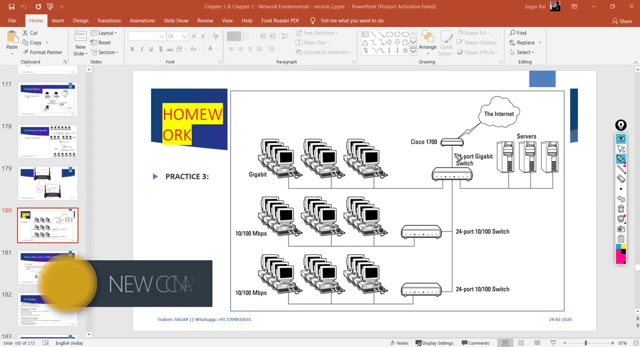 basically they are same, okay, but when we talk about enterprises, so i would prefer calling it as router instead of uh, modem. okay, modem is like for home users, okay, okay, thank you, thank you, yeah, so just think that of a router, but again, uh, whatever you were trying to uh correlate with 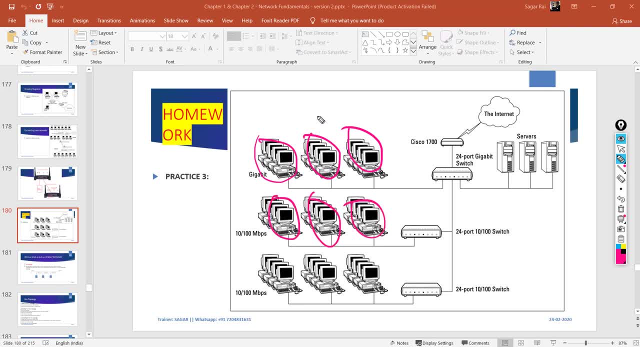 some, some scenarios with this diagram: okay, to allocate some fixed thing, so we we don't do it on router. okay, instead of router, we make use of some other third-party uh vendors- okay, or we can call it as like uh byod or mdm managements okay, where we have much more uh controls to uh control individual systems. 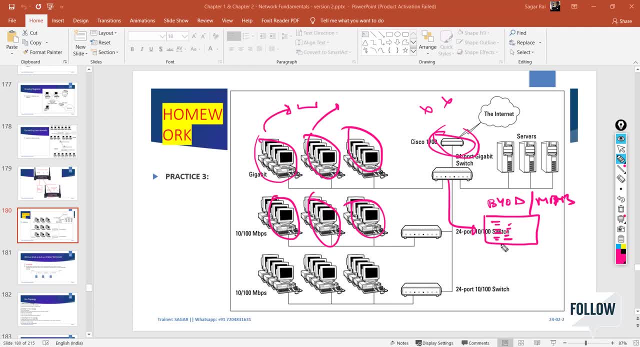 okay, router is not a good device where we can do, uh, such tuning, okay a in a router. the max I can tune is the data packet or the voice packet. okay, with the help of QoS. so what is QoS? imagine, this is all data packet, okay. 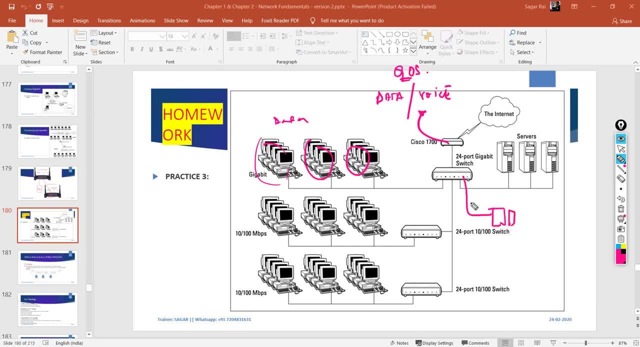 along with computers, I have some IP phones also now, like you told that these people are consuming so many datas. now there is a problem with voice, so what I can do with the help of Qs is I can give a dedicated bandwidth of twenty percent to voice and eighty percent to data, so that my IP phones are not facing any. 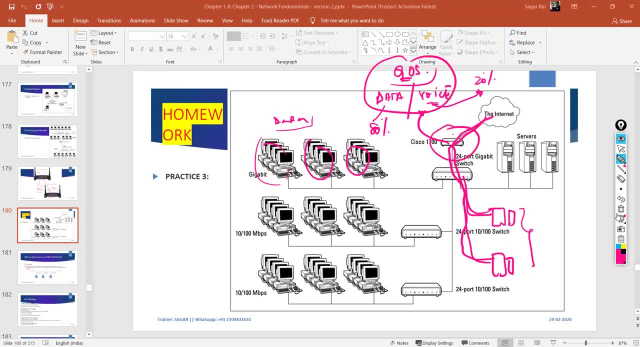 issues. okay, so this I can do on router. but what you are telling individually that router is not a good device to do that? okay, we have some better option. we have better option where you can control systems, okay. okay, so we, we will not prefer doing it on a router. okay, so we can have a different services there are free. 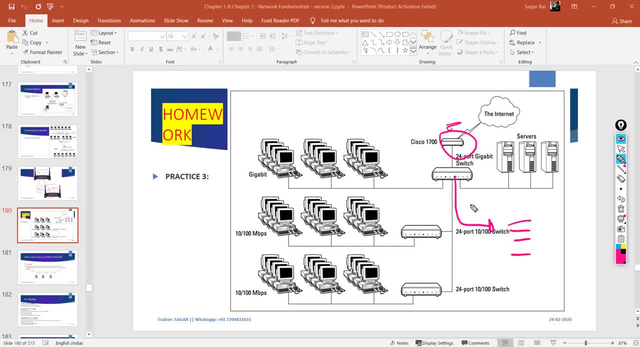 services. there are paid services so we can buy them. like we can install it in one server and then that application can control each and everything. okay, so that answers your question. yeah, it will be connected. no, no, it will be it. it is any vm server. let's say you are. 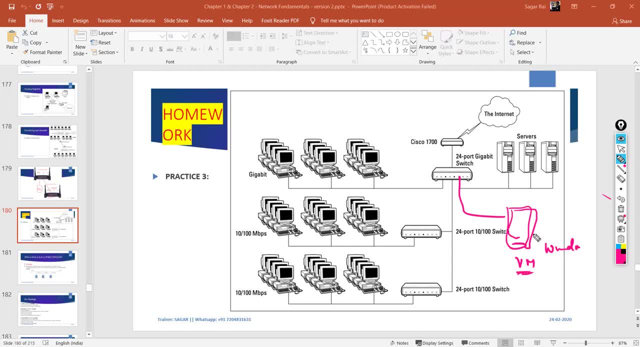 uh building one windows vm server. okay, it don't have to be physical server. okay, if you have uh. if you have a uh main server where you have some vm installed, you can build multiple vms right. so in that you just have to uh install the application. 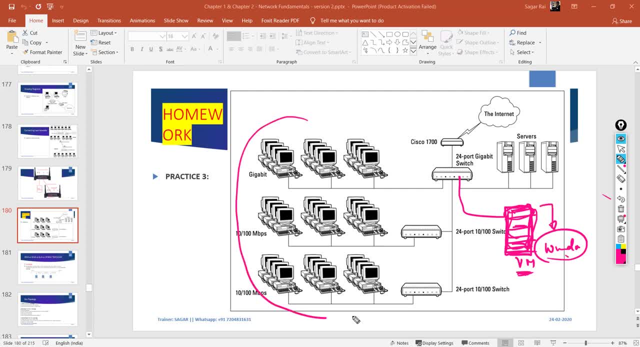 okay. and that application can record every activities. okay. it can record activities, like if someone is installing some application, someone is trying to download torrent, so basically everything can be visible on the software. so my point is: router is not a right place to monitor the services or who is downloading what. who is consuming uh bandwidth? okay, so we have. 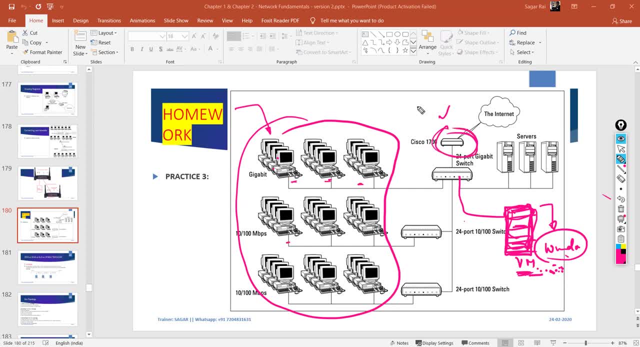 different applications. who can do that? okay, router is for routing the packet, so we are going with very small investment over here, like two hundred dollars to three hundred dollar uh investment. so basically our users can make use of internet for browsing or sending email or or such purposes. okay, 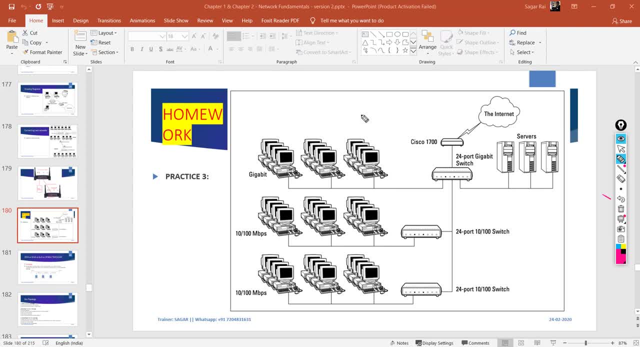 fine, okay, okay, hello, hello, yeah. tell me, can you please emphasize exactly what those servers connected to the switch, what is what they do on this network? you mean to say, uh, the servers? yes, yes, please, okay. so let's say i have three server, so let me name this server as abc and the abc server is loaded up with some. 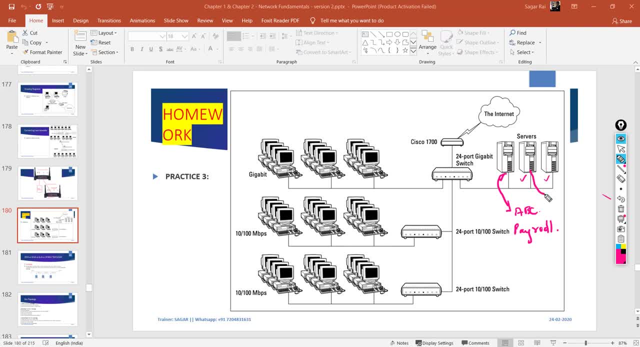 payroll application. okay, the server number, uh, let's say two, is loaded up with some, uh, login and log out application. so basically what is happening here is, let's say, this user is logging daily at 10 am, okay, so that should get recorded here. if he is logging out at 5 pm, so that. 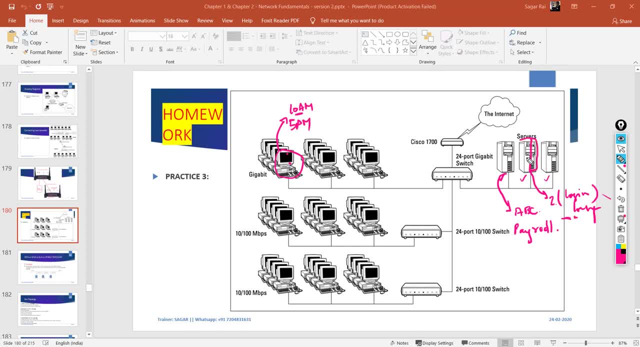 information should be recorded on this server. so servers are placed to serve some purpose, okay, like, for example, payroll. so might be. this is a user who belongs to hr team- hr team or accounts team- who is calculating the salary of individuals. does they want to see who has taken half day leave? who has taken a complete leave? so, basically, they. 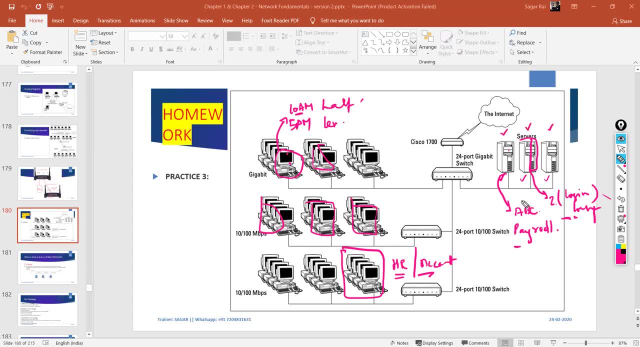 will get all the records from the servers. okay, so this is that payroll server where the application will be running. they are uh feeding the inputs. let's say, user uh abc took payroll from the server half day today, so his half day payment is getting detected. so are we going to manage some book and 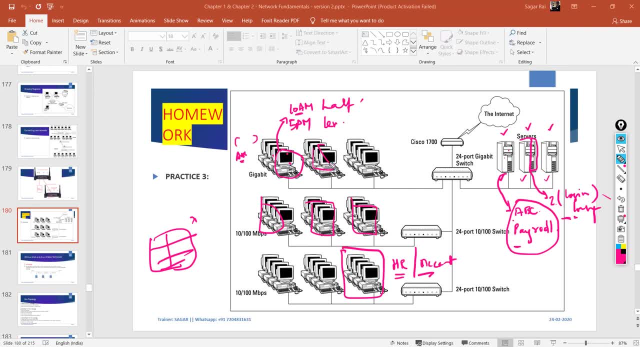 pen that this person took a half day. so basically it is all automated now. right, so it is all uh been stored in the server. so server is uh nothing but which can serve the purpose, okay, so what type of servers can we uh basically see? okay, so if i, if i talk about server, 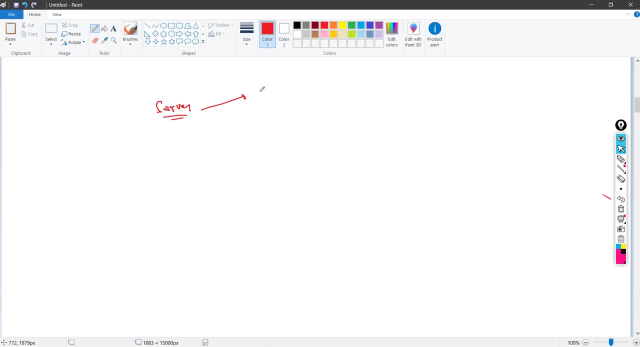 servers. so we can see servers where we can store some web page, like your company's official web page, xyzcom. okay, so server can be used to keep web page. now your office has a lot of mails coming in and coming and going out, so basically you can keep a mail server. 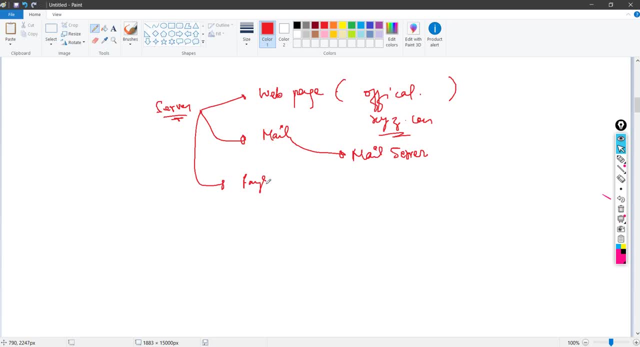 okay, similar way, you can keep some payroll application in a server which is calculating every employee's payment related uh information. okay, similar way, someone is uh taking a off or maybe he's going on some paid leaves, so who is going to keep a track? it's your server, okay. so basically, server is nothing, but you can load applications different.